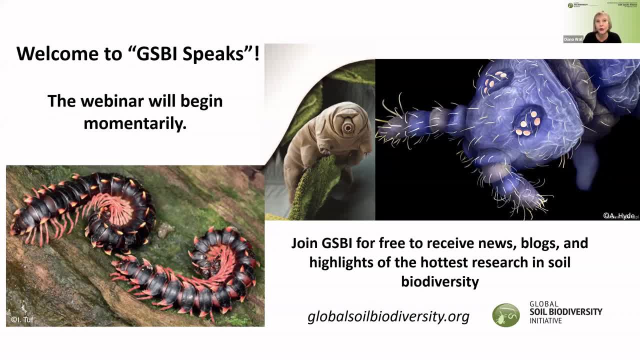 housekeeping news for you. Please use the question and answers The question and answers have. we'll be monitoring those, but we will not answer. we will not write answers to you because this is all going to be recorded and it's going to be on YouTube And so the answers won't show up. but 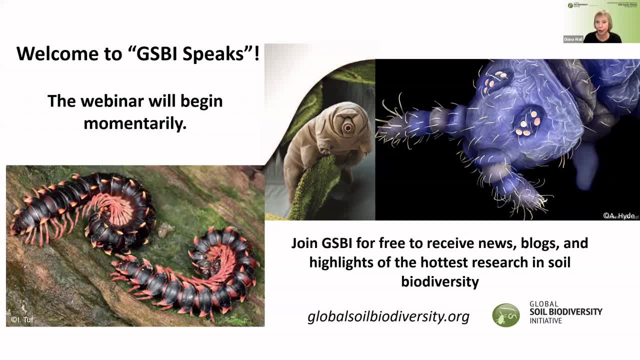 please answer in Q&A only, not in chat or anything else. The other thing that I want to do is just make sure that to make the questions come throughout the whole webinar, please do keep looking at the question and answer button. If you have any questions, please do keep looking at. the question and answer button. If you have any questions, please do keep looking at the question and answer button. If you have any questions, please do keep looking at the question and answer button back and see. if your question hasn't been answered, you may want to re-enter it. 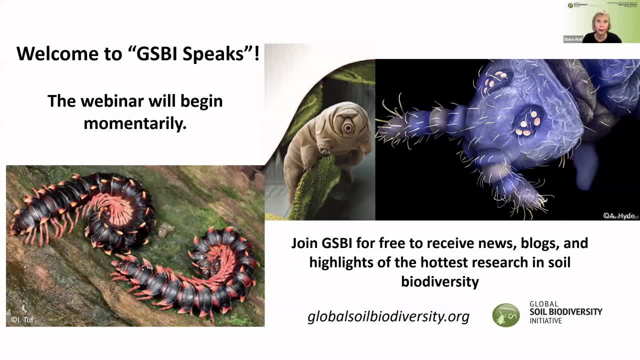 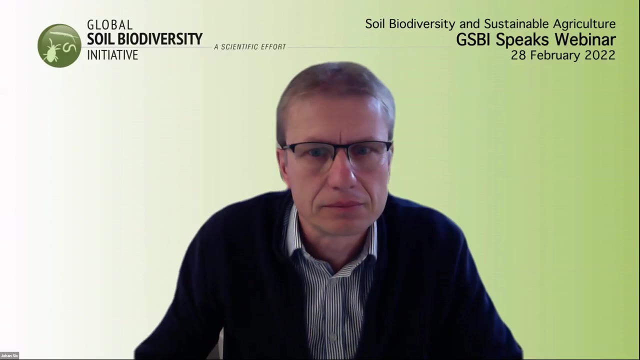 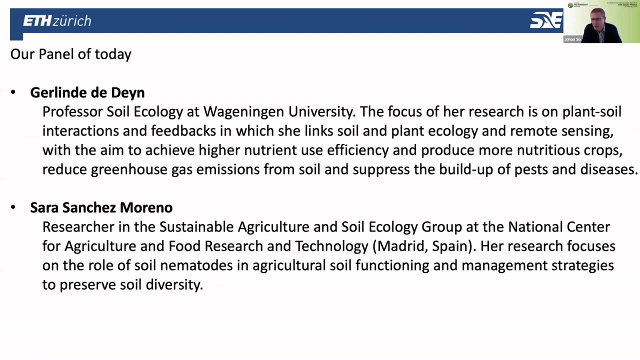 So now, what I'd like to do is introduce our moderator, Johan Six. Johan is from ETH in Zurich. Johan, welcome, Thank you, Diana. So welcome to all of you, And I will just quickly share my slides. So we have today quite an interesting panel. We have, you know, quite a bit of caliber. 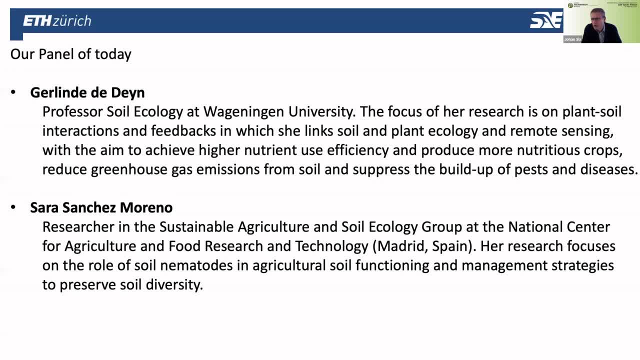 in our panel, And so I would like to just shortly introduce them, And then I will also just give a short introduction to the whole webinar. So the first person on our panel is Herlinde Dede, And she should be showing up. Yes, there is Herlinde, And so she is a professor of soil ecology. 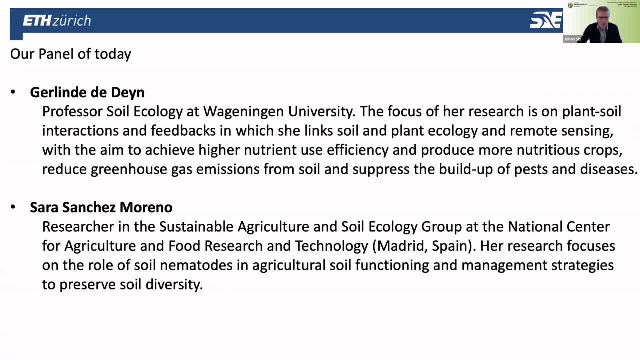 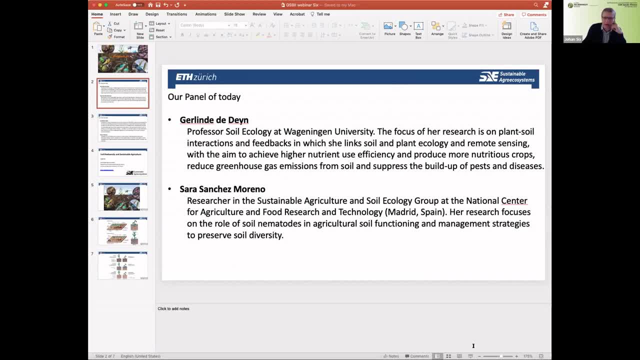 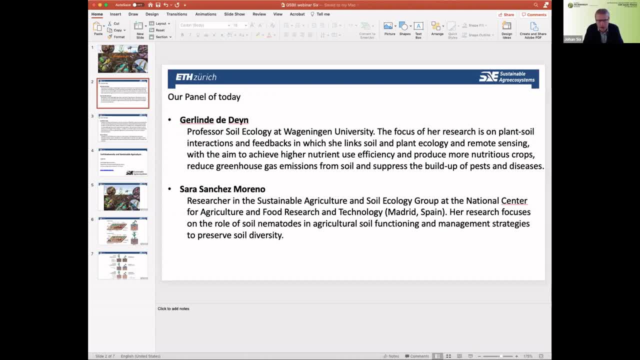 She is a professor of soil ecology at Wageningen University. The focus of her research is on plant-soil interactions and feedbacks, in which she links soil and plant ecology. and produce more nutritious crops is Sarah Moreno. and Sarah Moreno is at the National Center for Agriculture and Food Research. 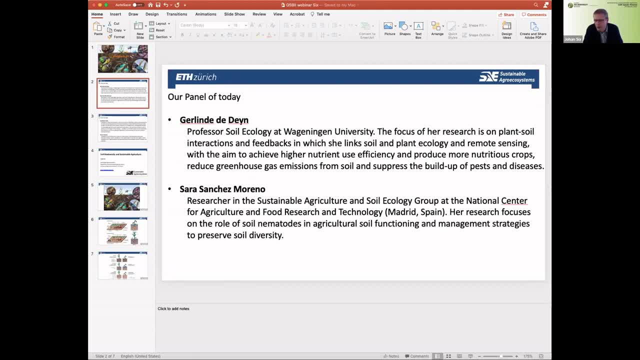 and Technology and that's located in Madrid, Spain, And she really focuses on soil nematodes in agriculture, soil functioning and management strategies to preserve soil diversity, And so, again, Sarah will also give some further explanations on that. The second third person. 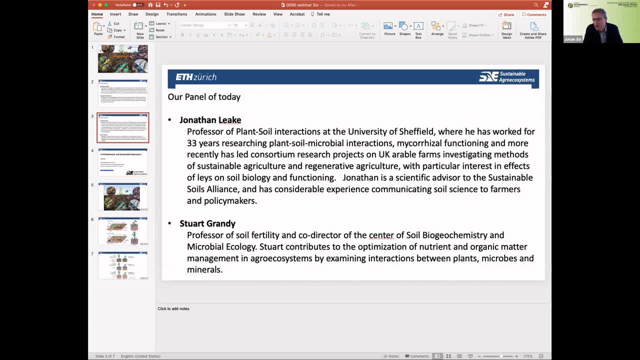 is Jonathan Leak- and you will see there is Jonathan- and he is at the University of Sheffield as a professor of plant-soil interactions. He has worked there for quite some time on plant-soil microbial interactions, mycorrhizal functioning, and more recently has also led some bigger research efforts in the field of plant-soil microbial interactions And he has also worked there for quite some time on plant-soil microbial interactions, mycorrhizal functioning and more recently has also led some bigger research efforts in the field of plant-soil microbial. 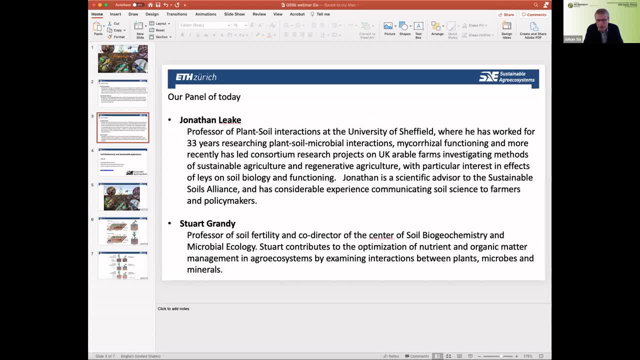 interactions, mycorrhizal functioning and more recently has also led some bigger research efforts, consortiums on UK arable farms, investigating the methods of sustainable agriculture and especially then regenerative agriculture, And there he has a particular interest in the. 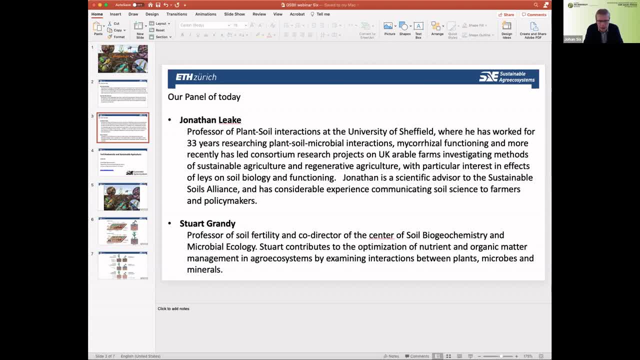 effects of lays on soil biology and functioning. Jonathan is also a scientific advisor to the Sustainable Soils Alliance and has considerable experience communicating soil science to farmers and policy makers, So I'm sure you're also looking forward to hearing from him about lays and how to 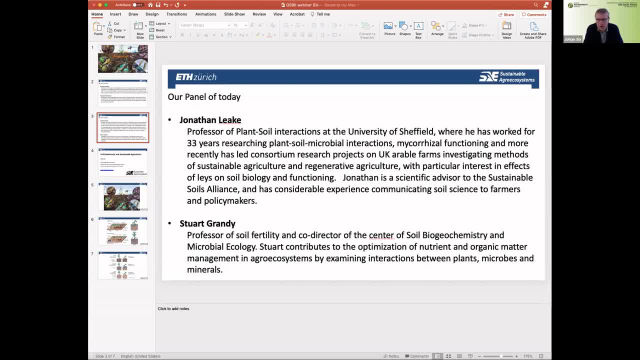 communicate about that with farmers and policy makers. And then, last but not least, we have Stuart Grandy. that's also joining us today, And you should see Jonathan coming on soon enough, And he is a professor of sulfur tillage And he has also worked there for quite some time on. 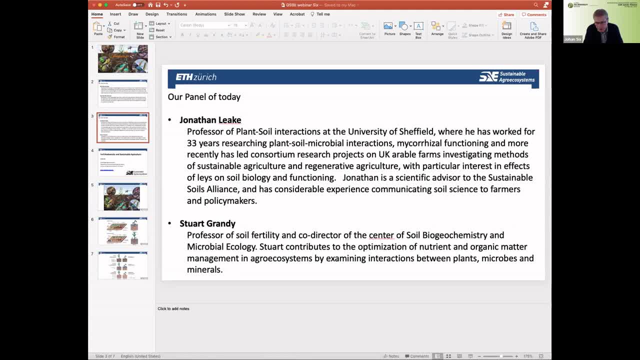 sustainability and co-director of the Center of Soil Biogeochemistry and Microbial Ecology. Stuart has mostly contributed to the optimization of nutrient and organic matter management in agro-ecosystems by examining interactions between plants, microbes and minerals, And also. 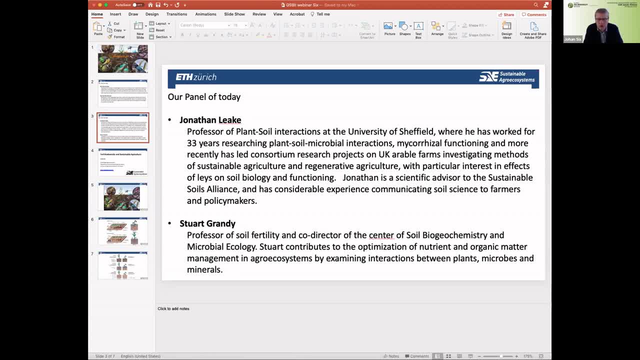 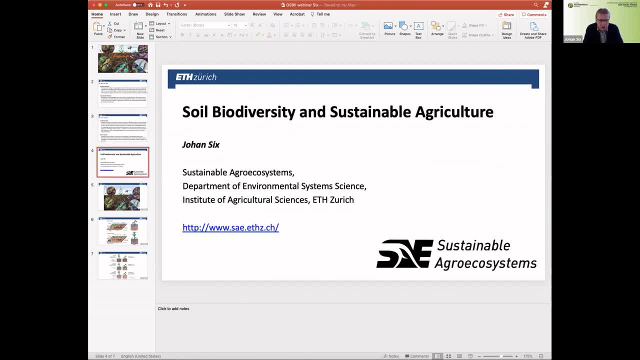 he will give some more details on that in his short presentation. So myself, just to give a bit more background: You know I do work here at ETH Zurich as a professor and I basically lead the group of sustainable agro-ecosystems, And so obviously that also explains why we're today talking about. 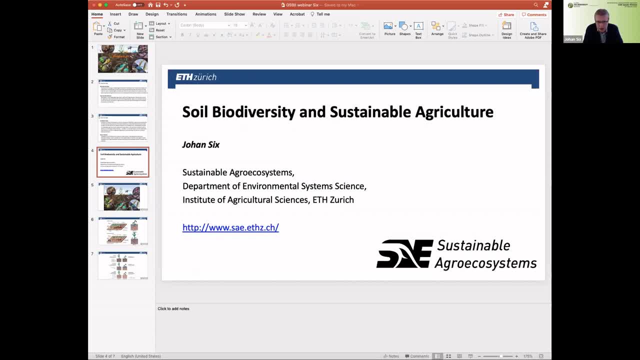 soil, biodiversity and effectively sustainable agriculture, And I've given a bit of task to all of our panel members to introduce them to some of the topics that we're going to talk about today, To indeed, you know, not talk too much in theory about this, but effectively come up with some. 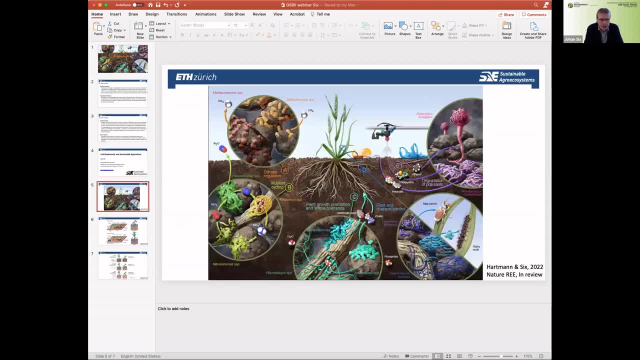 examples and practices of this, Because I think we indeed know. you know quite well, you know what microbes and our soil biota can do in general. You know they are obviously very important for nutrient cycling, They are important for degradation of pollutants. 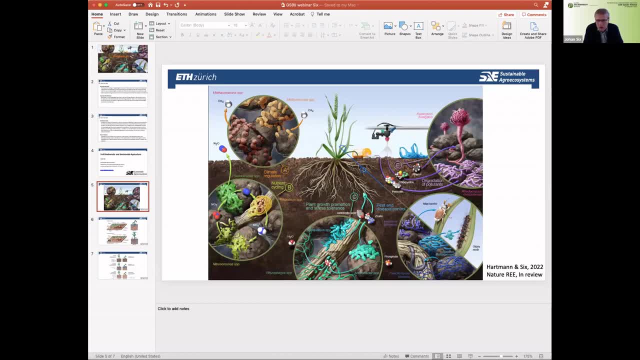 They can also help, obviously, with plant growth and stress tolerance. We there's a lot of talk today about how they can maybe help with climate regulation, you know, by regulating methane and CO2 and N2O emissions. And then also, you know more and more. it's also evident that they can. 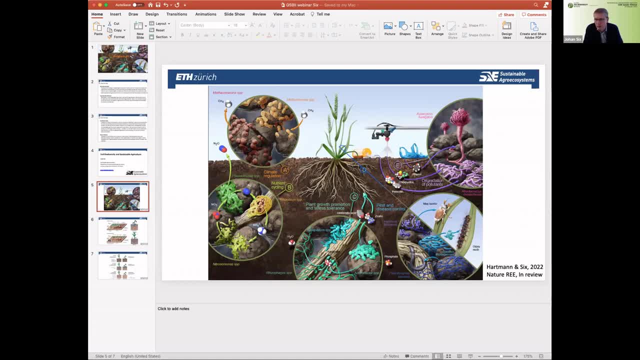 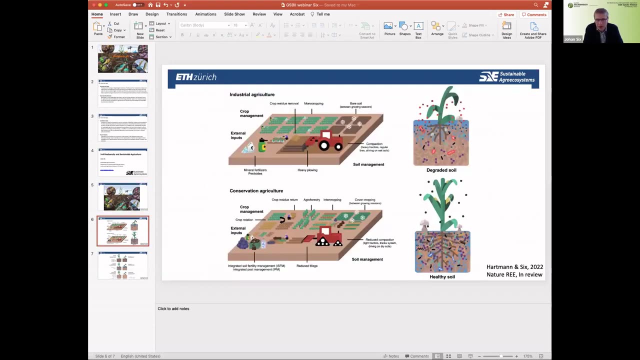 play a role in pest and disease control, both below ground and above ground. So you know, those things are quite well known, But some of the details clearly not. And then I think especially you know, we know already that agriculture can have quite a bit of an influence on that, Because 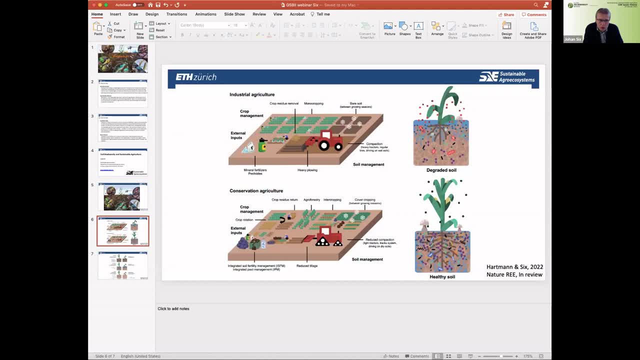 you know, lots of the industrial agricultural practices are effectively degrading our soils and therefore affecting our soil. So I think that's quite a big question. Thank you, our soil biota. and then the question is indeed: what can some of these alternative practices in agriculture do to actually make it again a healthy soil and a soil that is really helping maintaining these soil biota in their functioning, And so there's actually quite a bit of research on that too, and obviously it has a lot to do with you know how we're managing our soil directly and how much we can keep the structure. and the connectivity going, but then with the hope, and that's where I think, indeed, quite often it's then just assumed: if we have a better soil that indeed is enriched, biodiversity can help with nutrient cycling, again doing methane oxidation, having lower nutrient leaching, and so that's where we, today, will go. 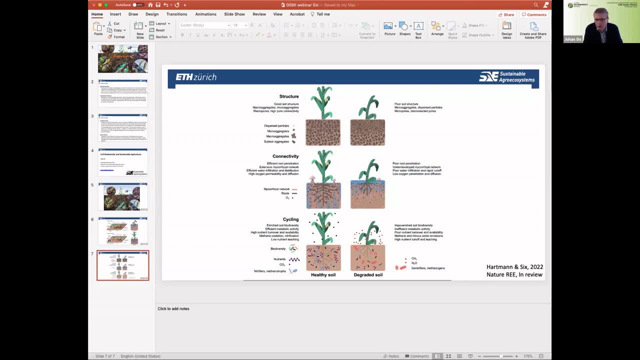 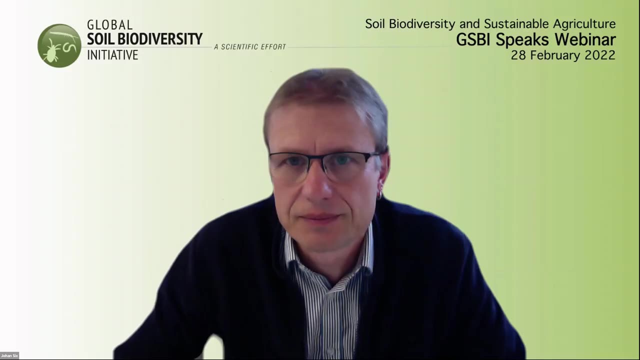 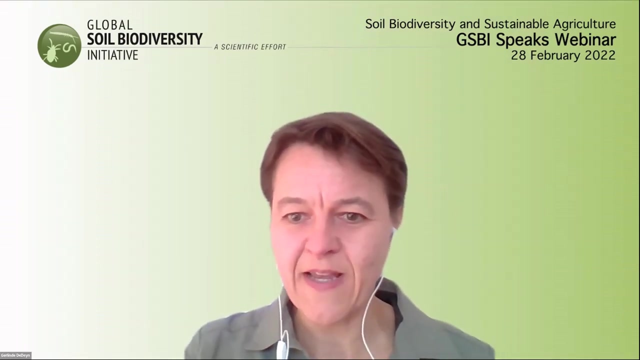 So, then, be talking more and giving some examples of how this could go. So, with that, I would like to open the floor to Herlinde, so that she can give her short introduction. Thanks a lot for the introduction and for the invitation, of course, and indeed I'm happy. 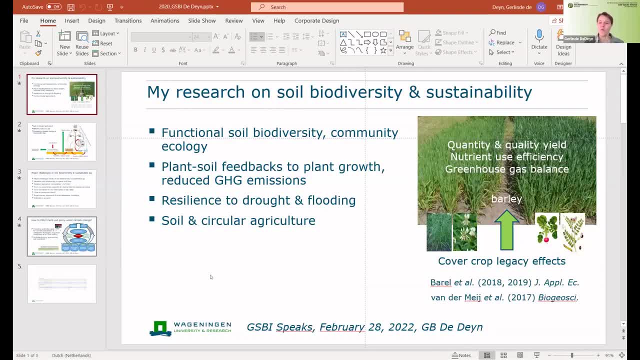 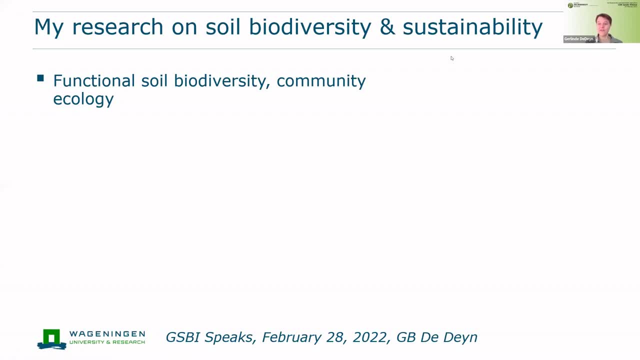 to take on this challenge, to present very briefly What my research is about and also to actually address the three short questions that were posed to us. I hope I can capture them in five minutes, but basically this is just the onset, for then the discussion later on. 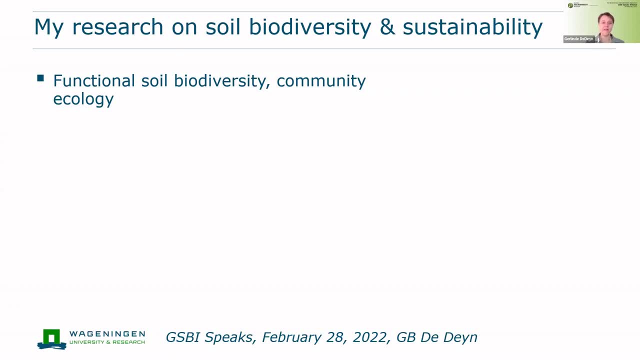 So what do I really do in terms of this soil, biodiversity and sustainability? Well, I'm mostly interested in this functioning of this soil, and mostly from a community perspective, and even more so specifically: how do plants interact with the soil and how does it then feed back to plant growth, but also to reduce greenhouse gas emissions and other soil based? 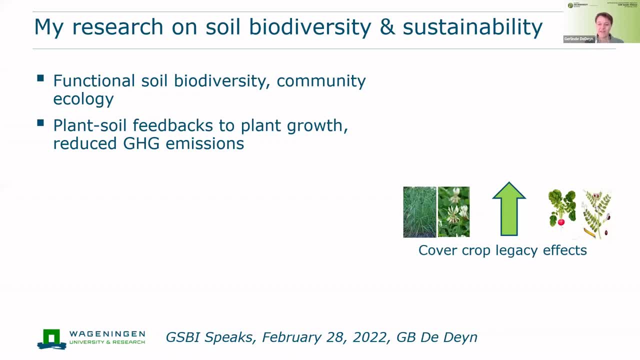 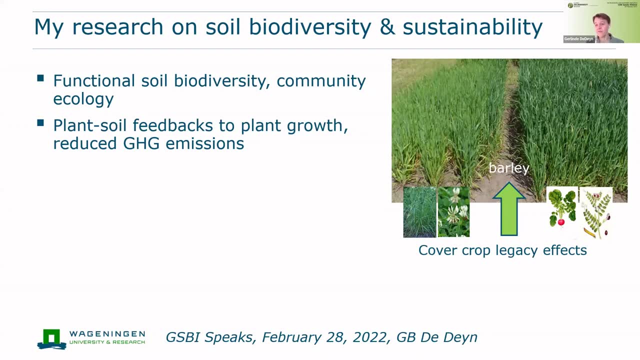 functions, And one of the tangible examples here is how cover crops create a legacy to subsequent main crops, and this is just an example of how we played around with different monocultures and mixtures. and here we can clearly see on the left hand side this is a legacy of a mixture. 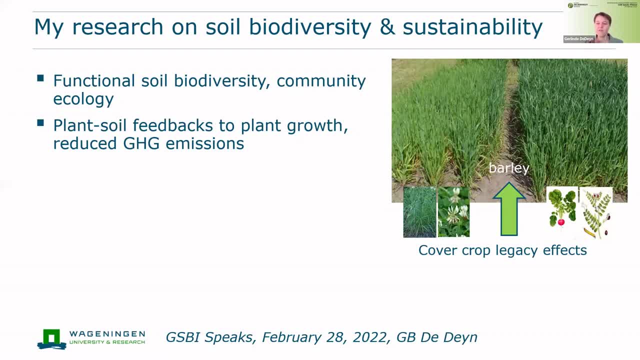 of two species, which actually was worse than the average of the monocultures, while on the right hand side We get this legacy that was better than the average of the monocultures of these two species. And so the way it works is indeed via nutrient cycling effects, but actually it's because 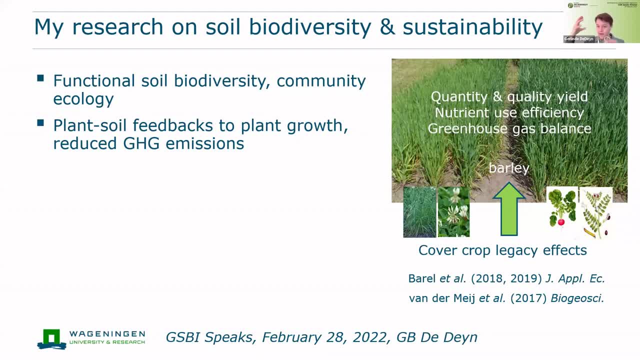 of the quantity and quality of the amount that goes in here above and below ground. that has knock-on effects on this soil community. that changes in activity and in size. So that's very relevant and actually we also made use of drones there to study that in. 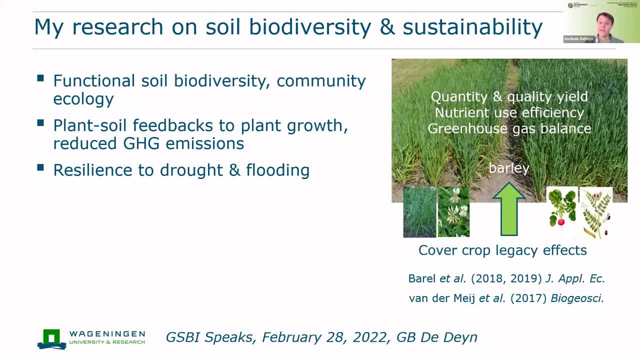 more detail. We also study effects of resilience and, to draw them flooding, in relation to management of agricultural systems. but I can't go into detail there, And my work also gets more and more connected to this idea of circular agriculture. And what do we mean with that? 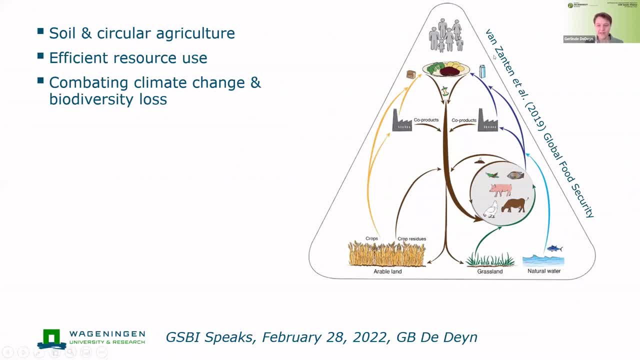 Well, here is a scheme on the right hand side. I hope you can see that fully because for me there's a bit of overlap of the zoom layout. But basically what it is. What it illustrates is that indeed, we harvest from the soil and we produce food with that. 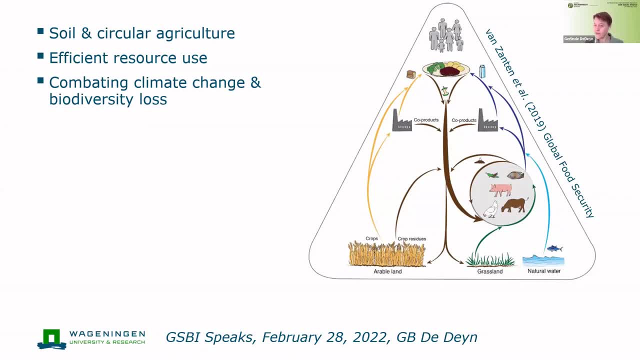 And the idea is that we actually should also return as much as possible back to the soil and keep the system as close as possible in terms of nutrient use and also in terms of energy use efficiency, And hopefully also, on the one hand, combat climate change with that so reduced greenhouse. 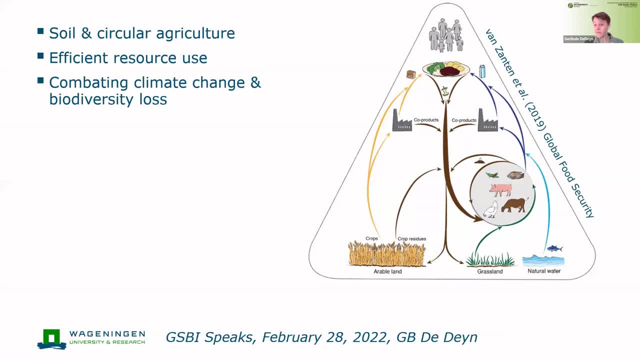 gas emissions, but also even promote diversity. because of this impact of managing our soils, We should- We should- reduce impact on the more natural environment as well, And indeed the soil is the basis here. That's the idea And that's also a role for us. I think to stress this because the idea is that a lot of these 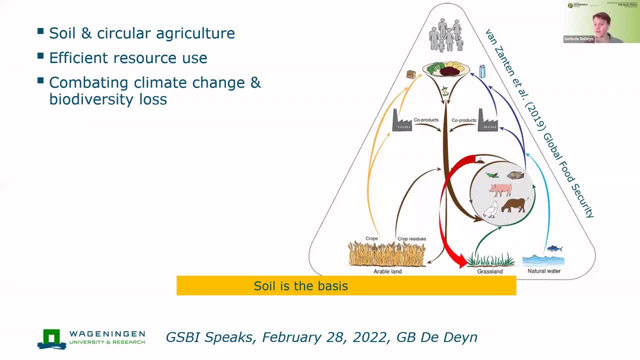 new kind of returns come back to the soil, And one example is like animal manure. But we have to be careful there that these manures can also have antibiotic residues, for example. So that's one of the studies we do is checking this impact of different types of antibiotic. 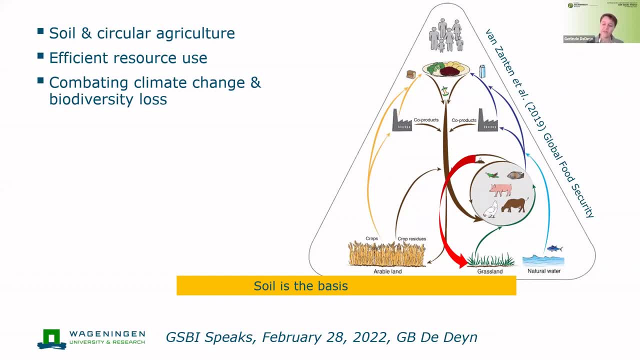 residues in manure On this, knock-on effects on the functioning of the whole soil microbial community and the emissions of greenhouse gases, and so on. Next to that, you see this connection also to natural systems, because there we have the issue of eutrophication, which is suppressing diversity. 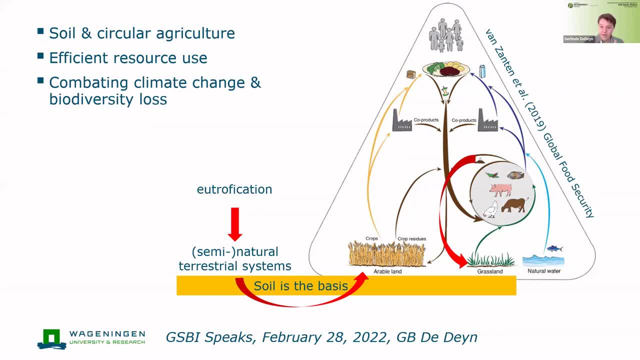 So what we do there is make use of harvested plant material from there, export it from the natural system and bring it back to the arable system. So that's in different ways like composting, bokashi and different forms, With the idea that we will build up or restore soils in the arable systems and promote biodiversity. 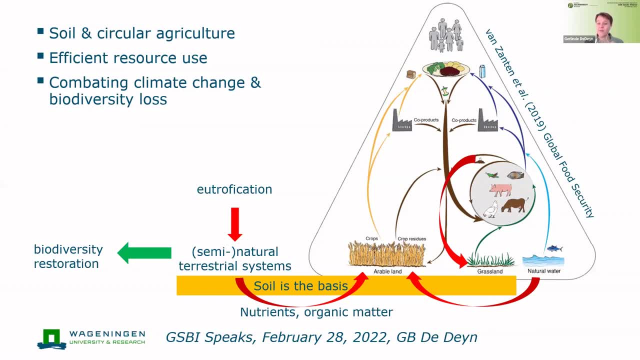 in these more natural systems again And we even connect there with aquatic systems where we make use of invasive aquatic plants, and that's a study we do in Zambia. So just to show that it becomes more wide, in a way more connected, what we're studying. 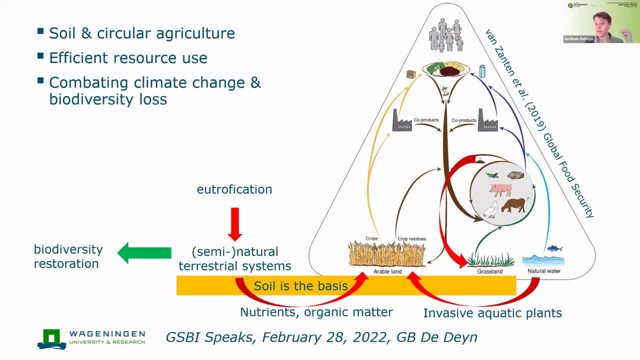 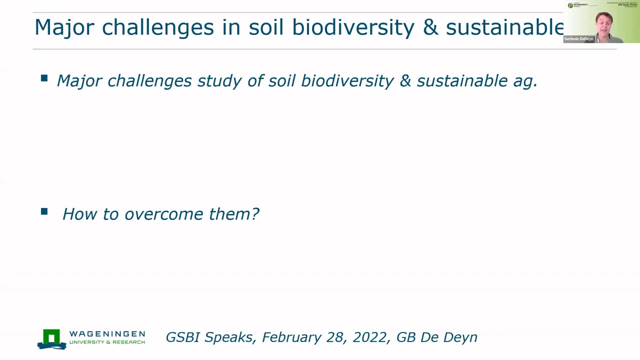 in terms of soil in agricultural systems, just because we're so interconnected by now, Thank you. And in the end that even feeds back to healthy food, so it really becomes relatively big. Then what are the challenges? and I'm just listing a few here because of time. 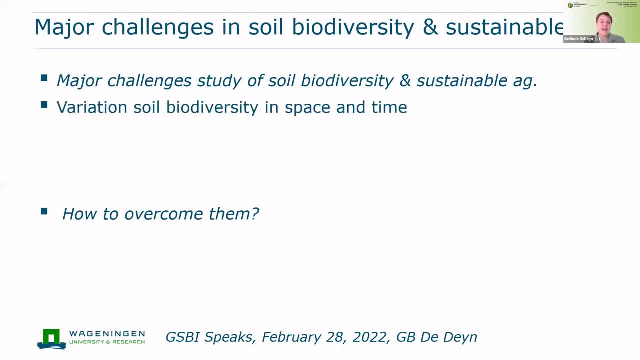 What I think are still pretty big challenges, or still this variation that we have to deal with in terms of biodiversity in space and time, This connection between really the taxonomy and the functioning and ideally go really make more mechanistically still and go in situ. We know a lot of things in the lab, but still these dynamics are happening in the fields. 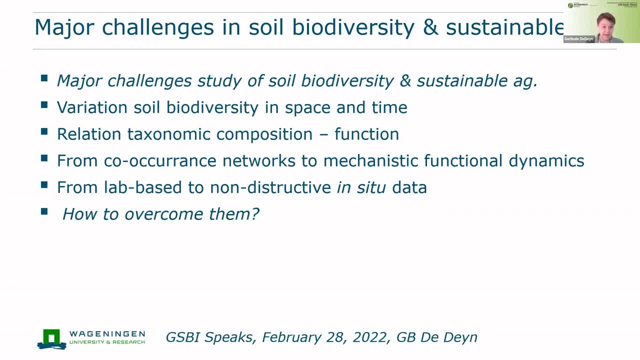 and to give advice to farmers. they have to manage their fields right. What can we do to overcome these challenges? Well, we still need experiments, I think, to be able to disentangle causes and consequences, Having these nice databases on how taxonomy and trades characteristics are really coupled. 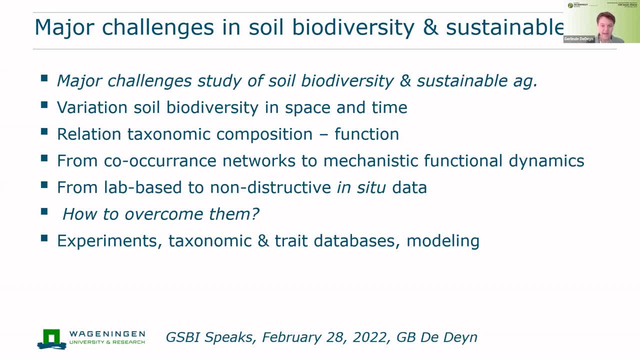 and if we really understand, we should be able to model it as well. I think- and modeling it also helps us to really zoom in and out at the right level to know what do we really need to know And, I think, in practice, to connect also to policymakers, indicators can be very helpful. 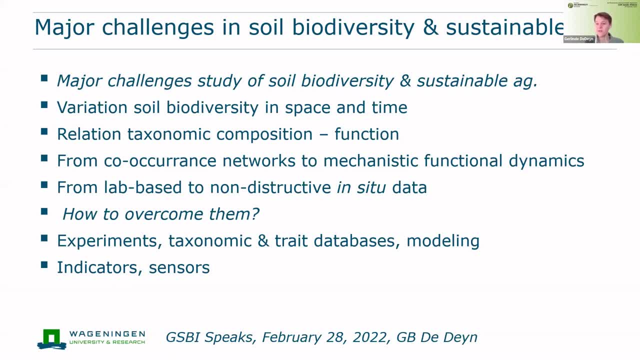 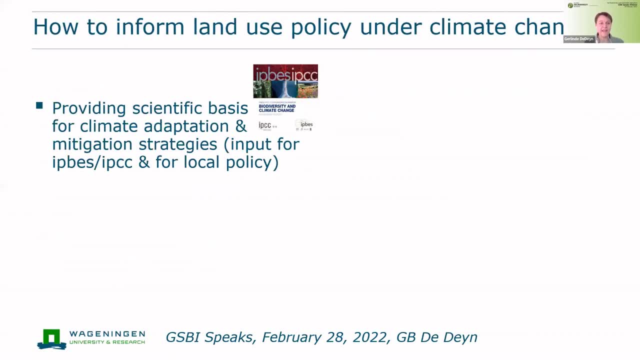 and for in situ measurements, I think sensors can be of good use. Some sensors are already available. others may still need to be developed for fitting our own purpose. Then I come to my final slide. that was the question on how can we inform policy or how. 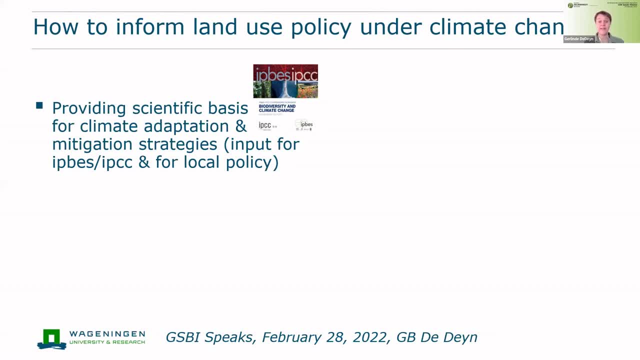 does our work contribute to policy? I think, in the first place, it is providing the scientific basis for these reports produced by IPPS and IPCC and also give advice to more local policy, like sometimes we do get these questions like, for example, the impact of solar ports on soil quality on arable fields. 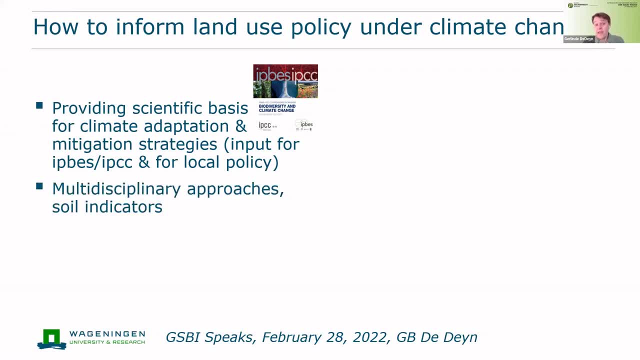 even And next to that, I think, yeah, we really need to work very multidisciplinary. and again, these soil indicators, I think can be a good communication component and also something that can be used to really see track where we are in the trajectory to where we want to get. 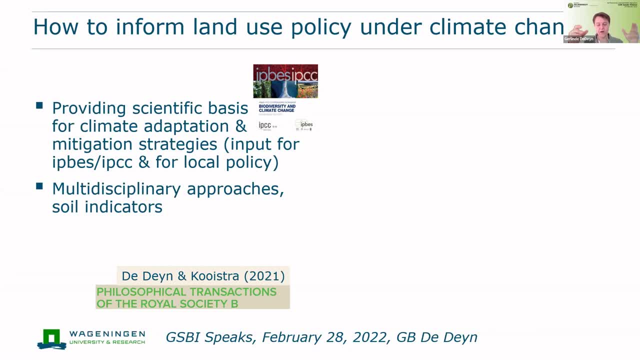 And related to that in this publication last year, which was part of a special issue on soils and nature contributions to people, we made this scheme. It's a little bit of a busy scheme but just to illustrate, I think indicators can indeed. 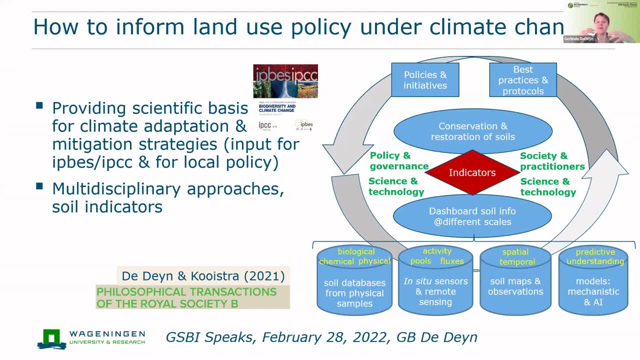 be a very handy tool, But you do need to connect them together with the stakeholders, together with the policy makers, so that you do speak the same language and that it is really science based And from the science perspective. that's what we have on the bottom side, all these different 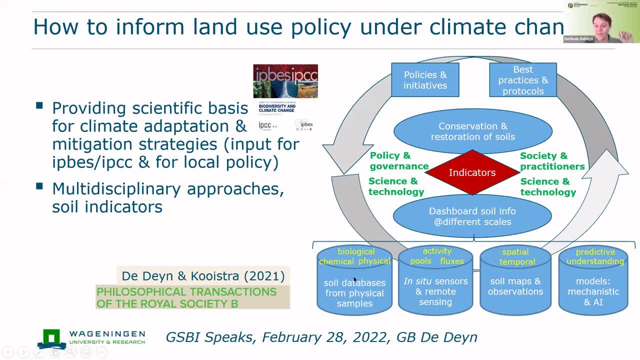 pools, let's say, of information that we have. So soil biology is definitely a part of it, but it's definitely not the only part of it, And we do need to have this integrative approach to really get and get to get to change. basically. 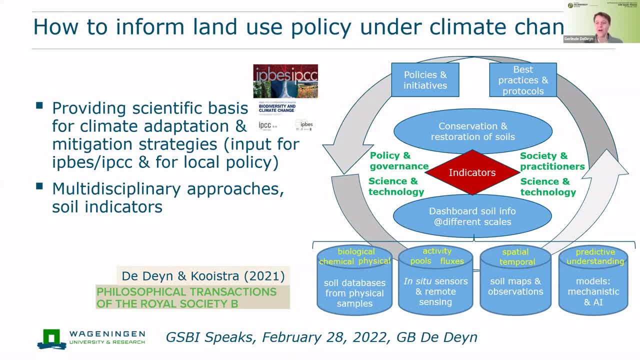 and for sure we can't do it on our own, But given the current situation and technologies and the communication we can, we can, I think, achieve a great deal in the next couple of years or the next decade, And with that I'm happy to stop sharing. 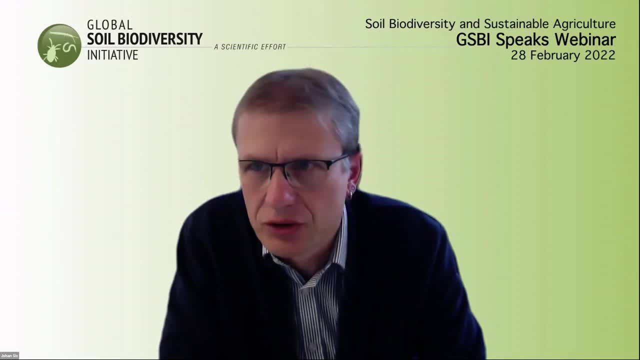 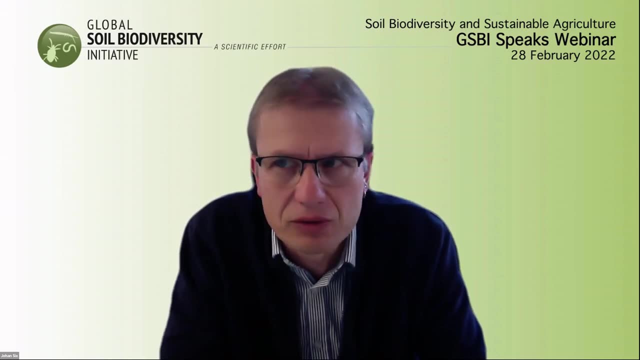 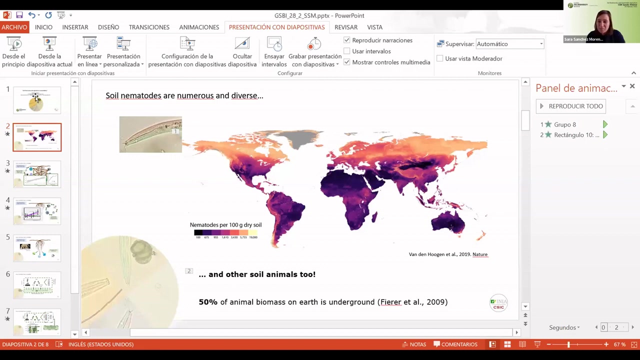 Thank you, Herlinde, And so I just want to remind the audience that you can indeed start putting questions into the chat. You can ask any question and answers And if I could indeed ask now Sarah to share and her expertise. Thank you very much, Johan. 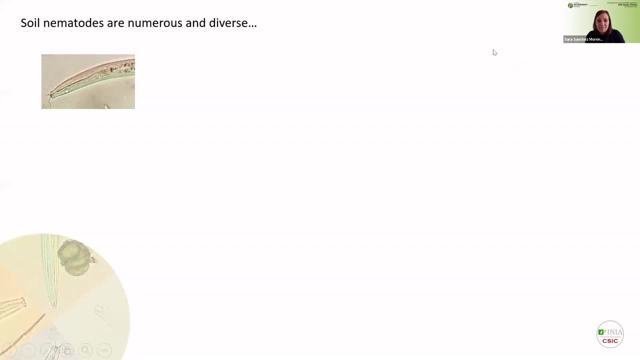 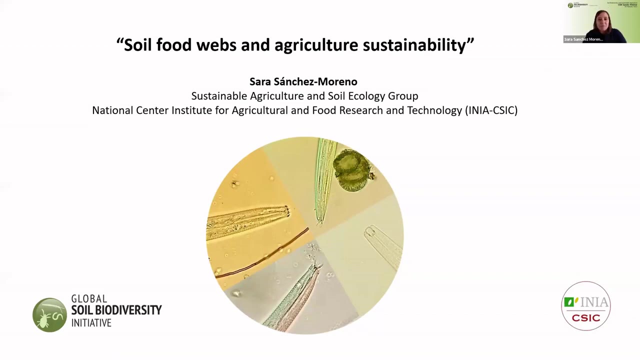 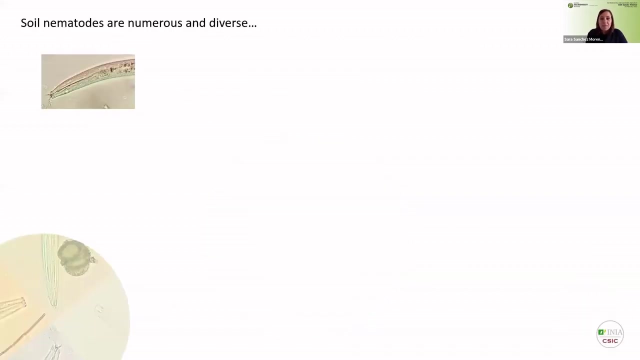 And thank you very much, Herlinde. Let me wait to take this out. So the title of my talk today is Soil Food Works, And I will cut our sustainability. I do work with soil nematodes. As many of you know, soil nematodes is the group of soil animals which is extremely abundant. 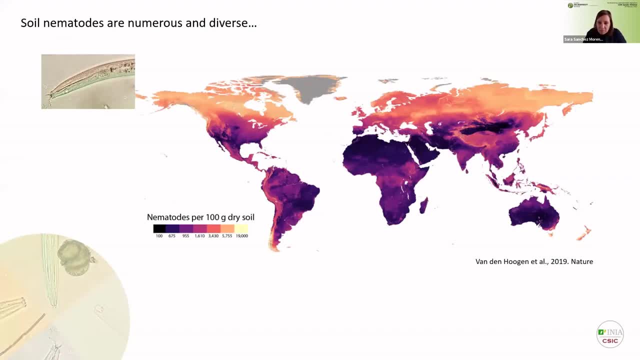 and extremely diverse. The recent paper showed that nematodes in soil. nematode abundances in soils range from a few hundred to several thousand nematodes per hundred grams of soil. That makes nematodes probably some of the most abundant animals on Earth. 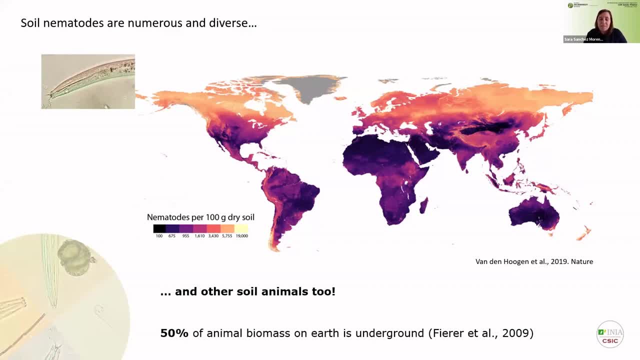 And they are not alone, because other soil animals are extremely abundant too, such as mites, columbula and so on. Some estimates say that 50% of animal biomass on Earth is underground. So my research clients deal with how to manage the soil. 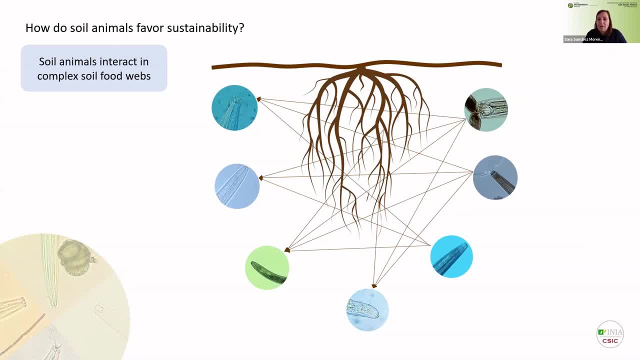 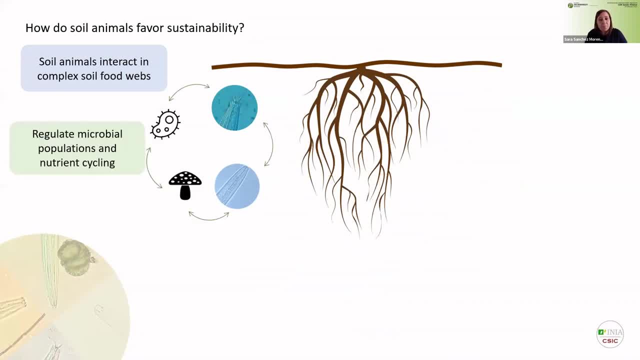 and with other components of the soil biota. For example, many nematodes and many other soil animals are bacterivores and fungivores and they feed on bacteria and fungi and they regulate microbial populations and nutrient cycling, increasing soil fertility. Previous research: 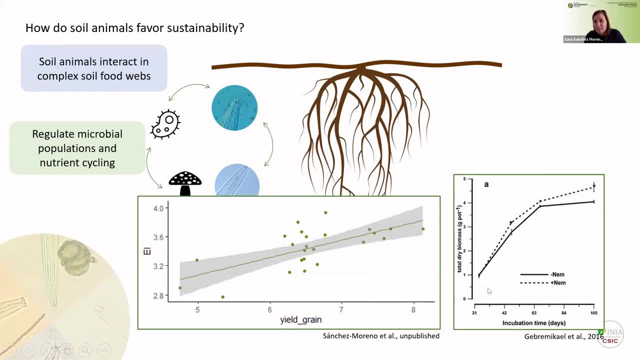 showed, for example, that crop biomass is higher in soils with nematodes than in soils in which nematodes have been experimentally excluded. We have also found that some nematodes, those bacterivore nematodes, closely related to 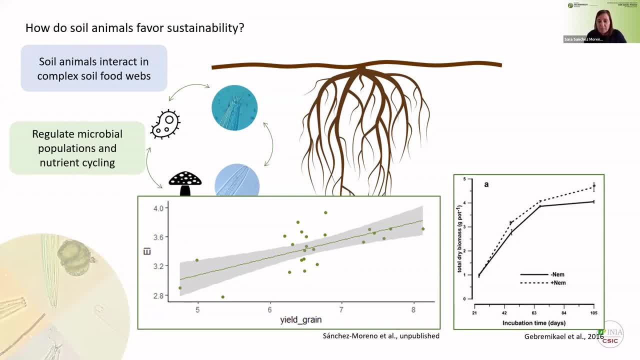 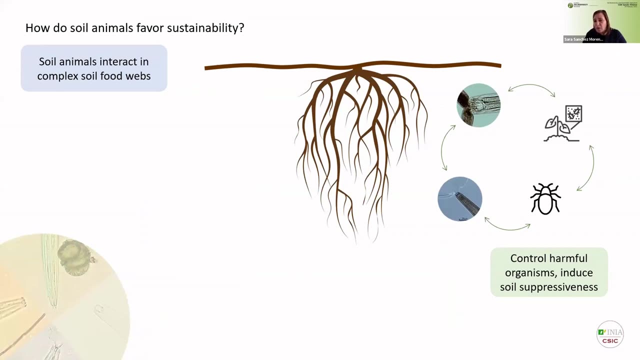 microbial communities in the soils are very related to grain gels in agricultural systems. Other soil animals are predators and omnivores and they control harmful organisms inducing soil suppressiveness. Soil suppressiveness is the ability of soils to fight against diseases and pests, And we have also worked. 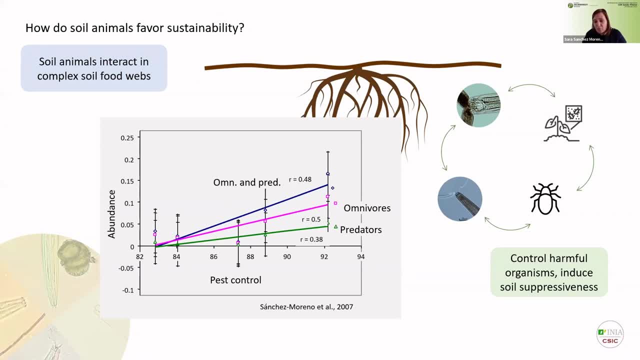 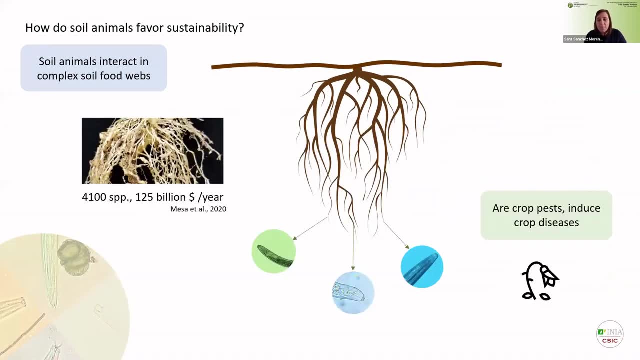 on studying how these predatory and omnivore animals in the soil exert as pest control agents. But of course, not all soil animals are beneficial to crop yields or crop performance, and many of them are crop pests or they induce crop diseases. Actually, more than 4,000 nematode species are plant parasitic and they cause losses of 100%. 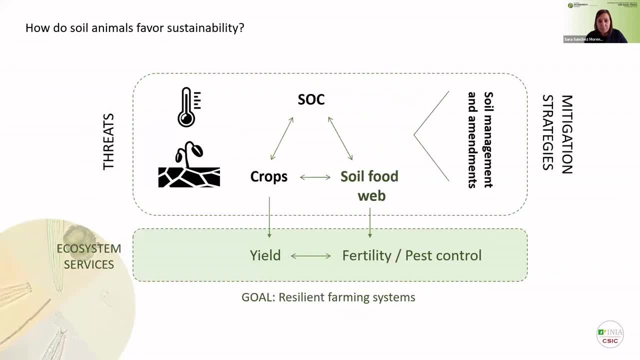 of their life expectancy. so they're 60% of the rate of production of the soil. The final metric is the increase in soil efficiency by about 12.5 billion dollars a year. So my research line deals with how soil food webs relate to soil, organic carbon, other nutrients and 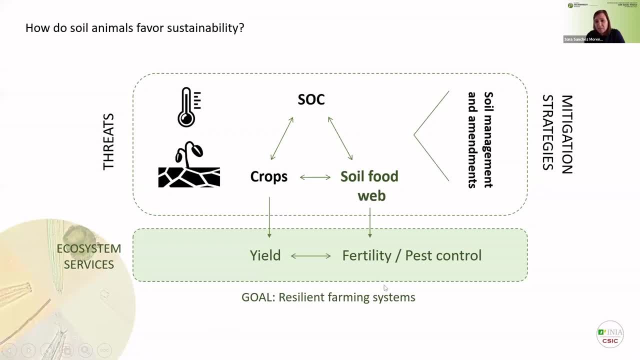 crop performance In general. how soil food webs deliver ecosystem services such as germ fertility and pest control. These relationships here are threatened by climate change, but these relations will be preserved for the next decade. We also looked at a particular study in 2016 that was done in the United States. A study who has a very similar approach to soil, organic carbon and other nutrients, is a scientist whose research has been in the area of plant onset and for over 30 years he was involved in a research team in the United States. The scientific research team has contributed much to this research project, which has been 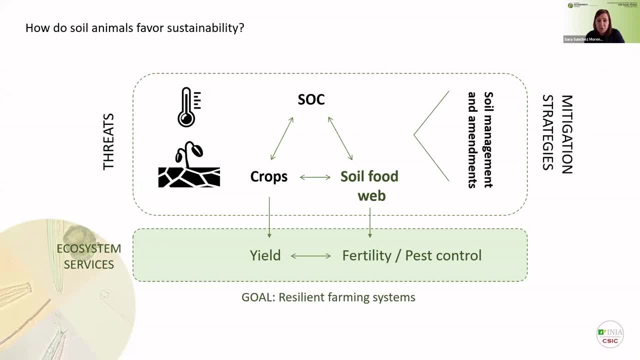 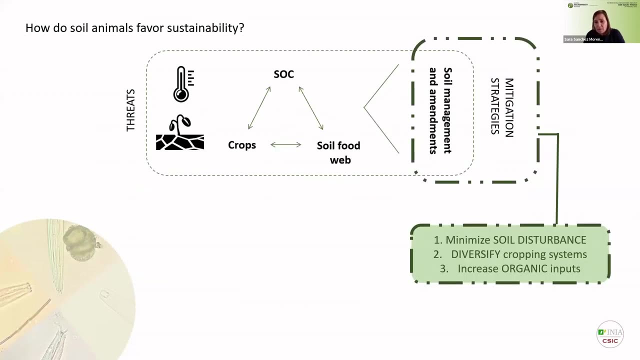 working at a larger scale of monitoring, and his research team has been working climate change factors such as warming and drought, and we studied how different types of soil management may act as mitigation strategies against climate change. Those mitigation strategies are, for example, minimizing soil disturbance. 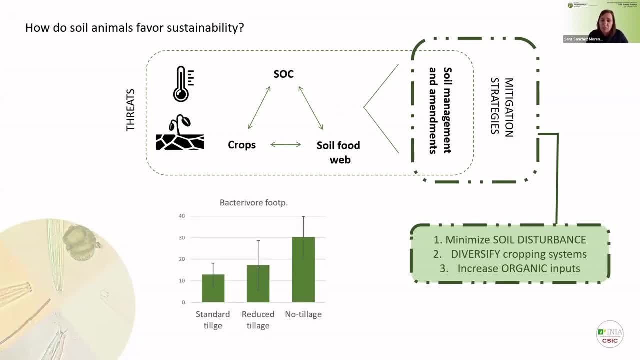 We've clearly seen how reducing tillage- for example, using reduced tillage or no tillage- increase the participation of those bacteria or animals in the soil, mineralizing nutrients and increasing soil fertility. The second strategy would be diversifying cropping systems. It is 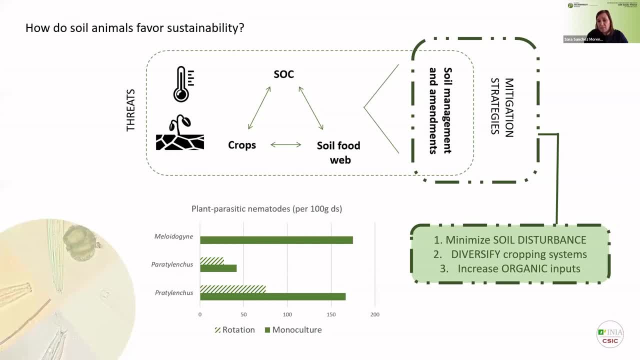 well known. it has been shown everywhere that including rotations in agricultural systems reduce the amount of pests in the soil, for example, reducing the abundances of plant parasitic nematodes And, finally, increasing organic matter inputs, especially in the soils in which I work with. 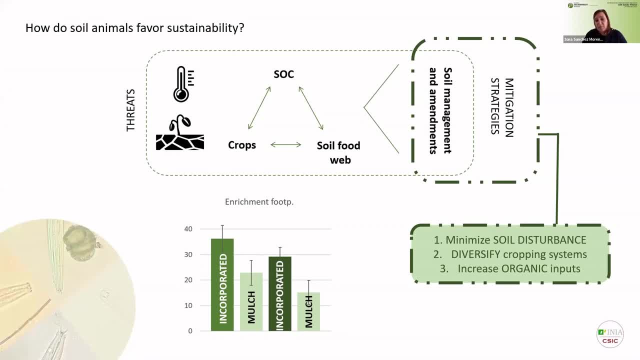 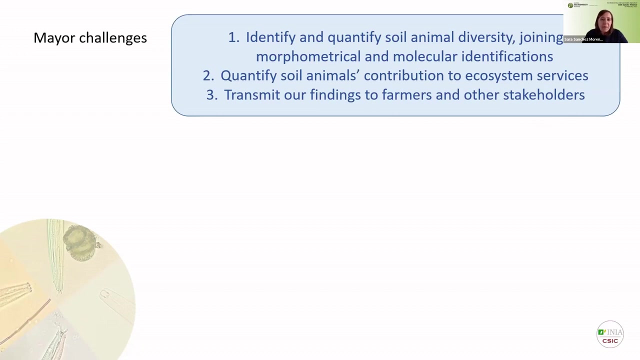 are very poor soils with low contents of organic matter in quite arid conditions. So we have seen that incorporating cover crops into the soil also optimize the participation of soil animals in nutrient cycling, increasing soil fertility. For this reason, species can beaquipmenters with high resources has prevent euphoric. 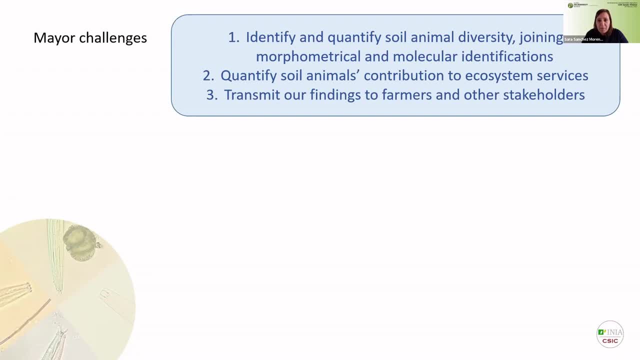 and cytokines fromましょう. So, in relation to the major challenges in this topic, I think the first one would be to identify soil animal diversity, joining morphometric and molecular identifications. third one: transmitting our findings to farmers and other stakeholders. I think it is very, very, very. 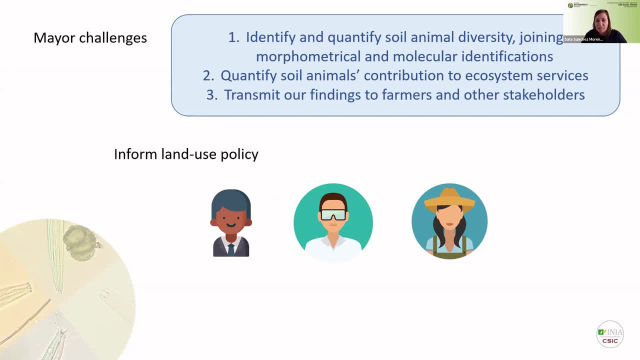 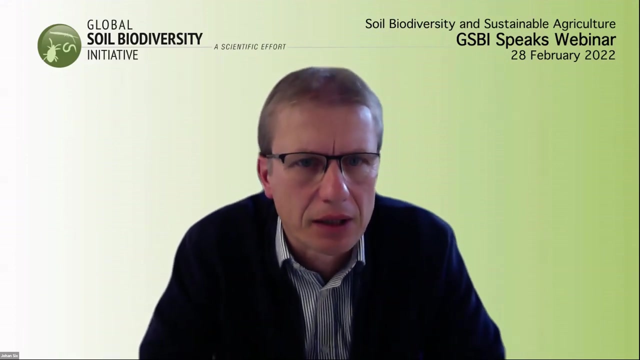 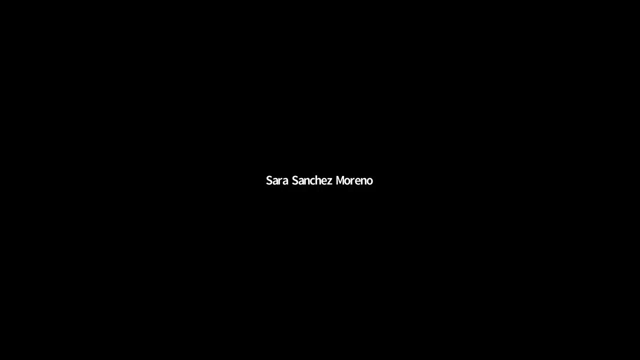 important to establish effective communication channels among farmers, scientists and policy makers to transmit that protecting soil diversity and soil fauna is protecting agricultural sustainability worldwide. And that is all, thank you very much. Thank you very much, Sarah, and if I could ask Jonathan to present, 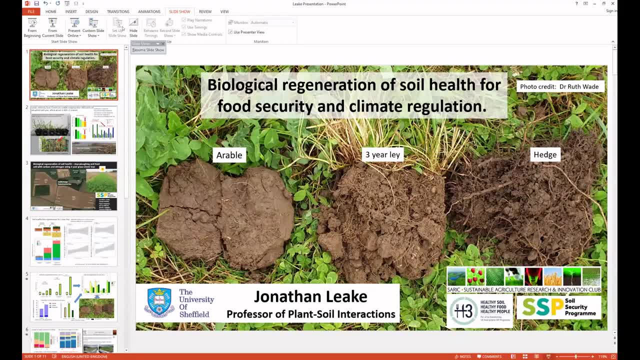 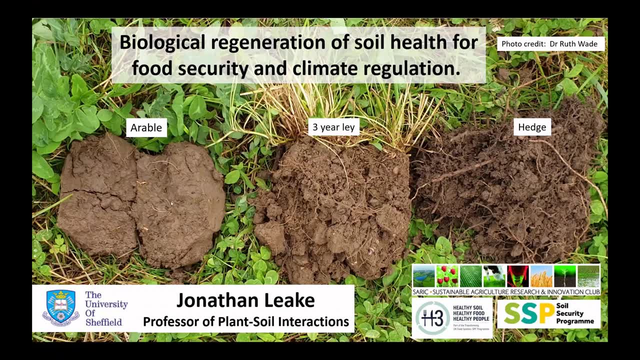 Jonathan Weston. So thank you very much for the invite and I want to just talk to you a little bit about some of the work that we've been doing on biological regeneration of soil health. I mean, the opening photograph tells a big story. actually, it's just: we have a permanent arable. 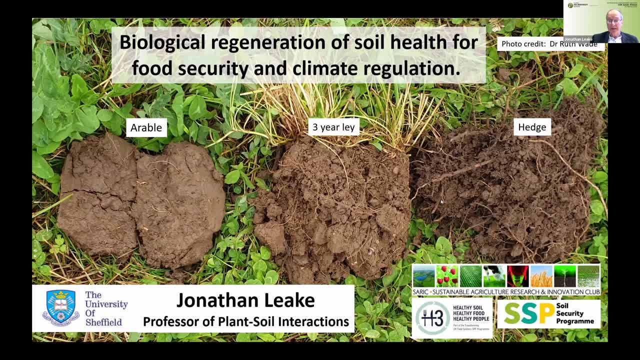 field into which we introduce a three-year lay. So it's grass and clover. it was just mown and the soil radically changed over that three-year period. The stopping tillage, the feeding of the soil with roots and nitrogen fixed by the plants. 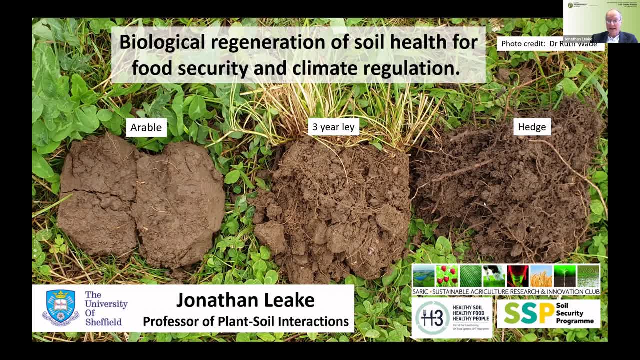 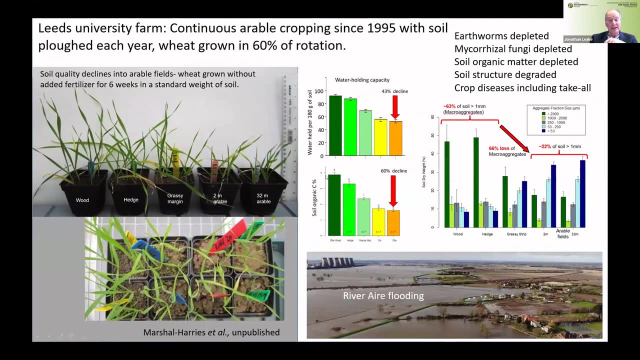 was transformatory- and I'll come into the details of what it actually achieved shortly- And you can see that it's rebuilt some of the structures that you see in these long-term permanent hedge soils which are decades, well, probably centuries old. So I suppose our starting point was actually looking at the extent to which 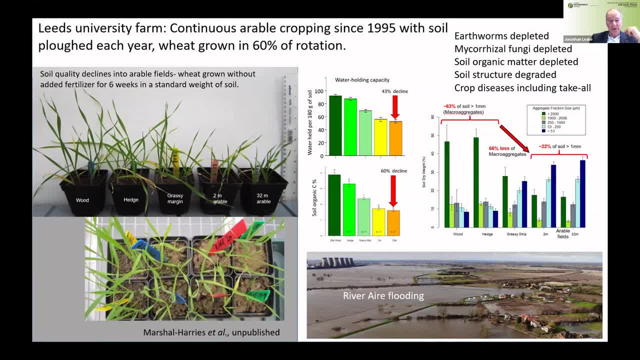 intensive arable cropping was causing soil degradation and the simple way of looking at this initially was to take a standard weight of soil and grow wheat in it, just watered with standard tap water, no nutrients added. and looking at what happened And when we looked down into these soils, we could see such a way they were. 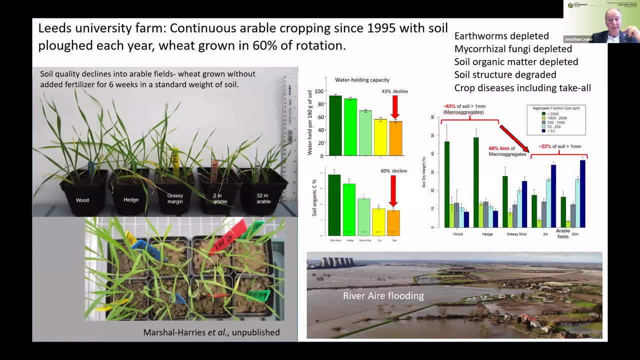 very different in structure and enormously different in function, as you can see from the response of the wheat plants, And the structural differences resulted in very major losses in water holding capacity, associated with a very large loss in soil organic matter, But also- and you can see this very clearly here- the soil lost its structural stability with this. 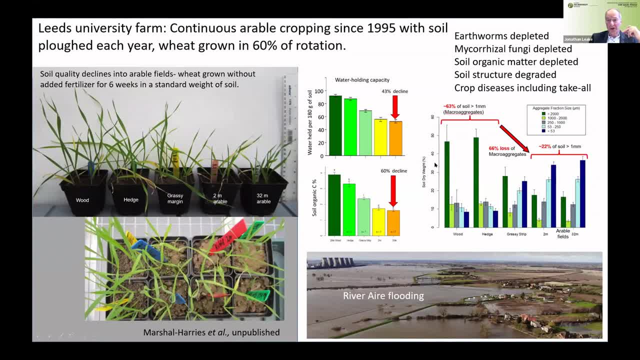 loss of carbon and so the larger aggregates which are dominant in the better structured, organic rich hedgerow soils and soil And field margin soils. in these permanently arable soils, these are lost and the major aggregate fraction that we see here actually is the smallest fraction, less than 53 microns. 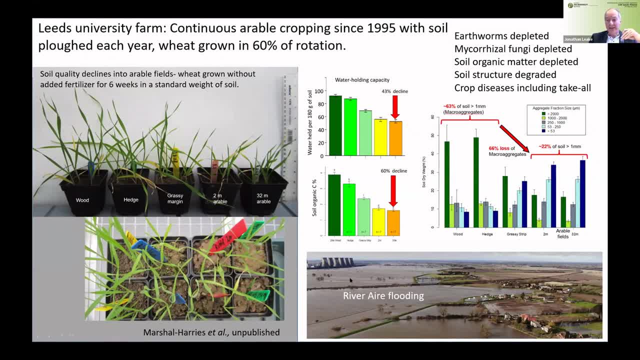 And there are consequences of these changes. This is a landscape scale effect that we see over much of Yorkshire, where these soils came from, And it's an area which is now subject quite often to extensive flooding that affects properties and livelihoods, And the soil is biologically depleted. It's not just structurally and chemically depleted. 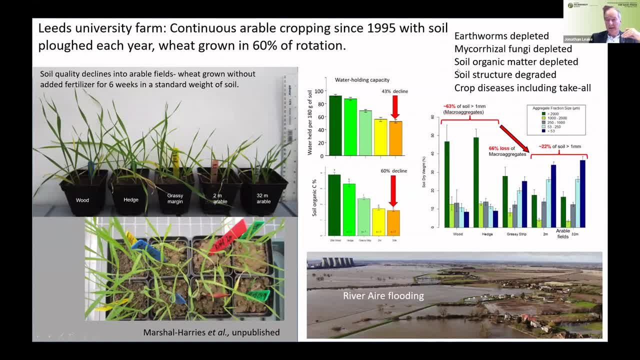 The earthworms are depleted, the mycorrhizal fungi are depleted, the organic matter is depleted, as I've already said, The structure is degraded And we also have problems here of crop pests and diseases that are also connected to this loss of soil biota. 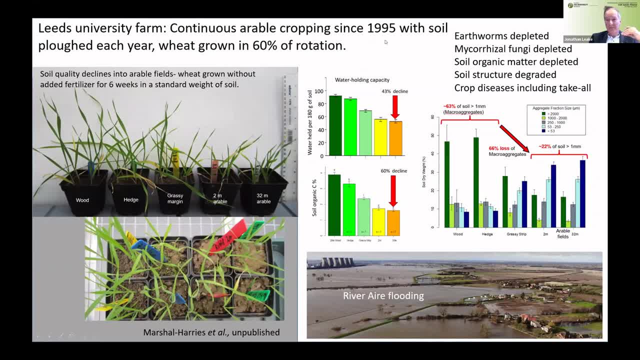 What's been going on here is continuous arable cropping for decades, soil ploughed every single year, Wheat being grown in 60% of the rotation. So we were interested in trying to reverse that, And so what we did was we put in lay strips into these permanent arable fields so we could 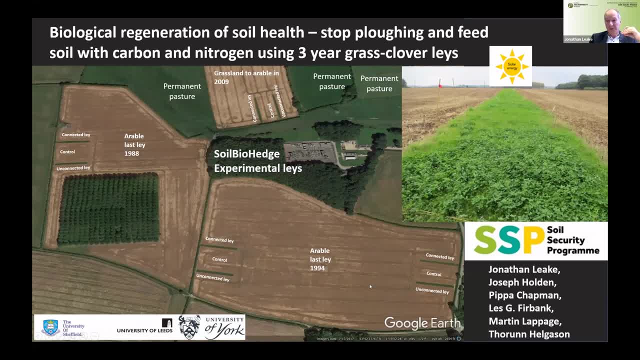 compare alongside the same field, same soil types. all we did was locally change the management and started to investigate what result that this was, And I suppose one of the first things to note is that this is when the wheat crop's been harvested off the arable field And in the late summer we've still got a bright green. 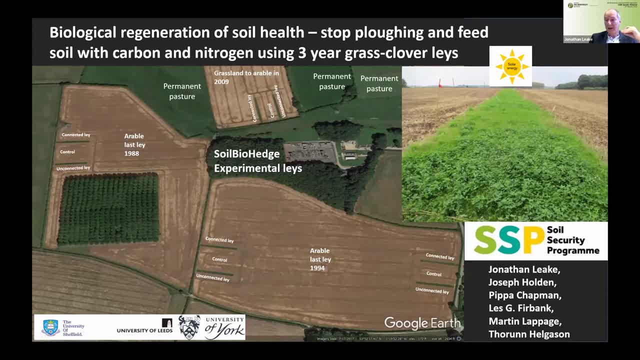 strip, photosynthesising, fixing carbon and supplying carbon into the soil, And other data suggests that actually these kinds of lay systems probably more than double the amount of carbon going in through roots into the soil. Feeding the soil with live roots is probably one. 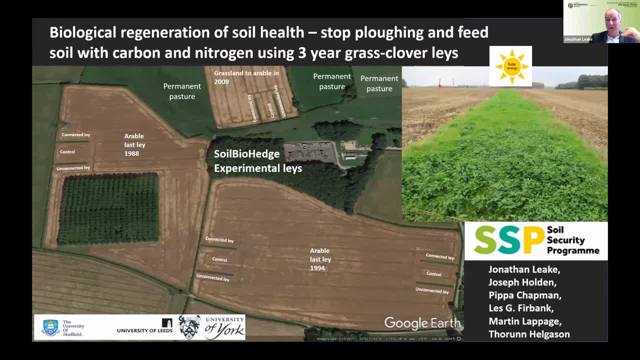 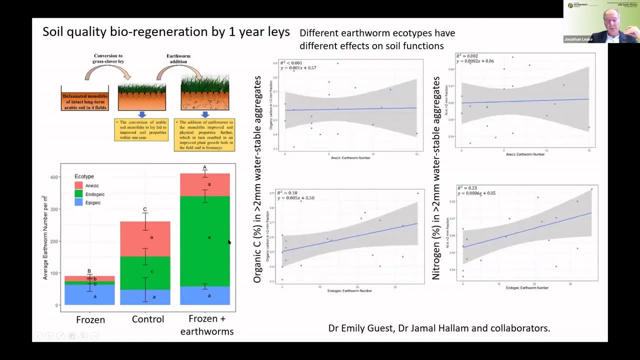 of the key processes to support soil biology actually, And it's a central, pivotal role in regenerative agricultural systems. So this is what our system looked like, as I say, And then we also conducted more detailed experiments within this system. So we actually dug up blocks of soil, shoved them in a deep 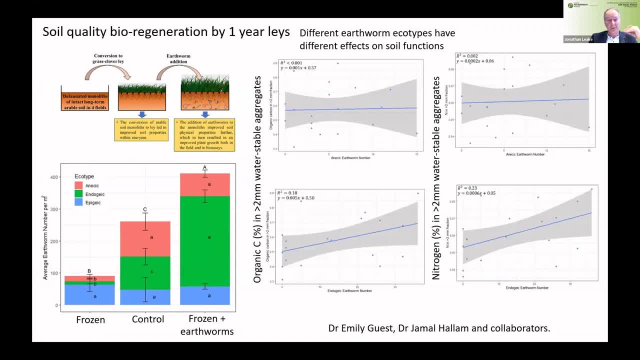 freezer to try and eliminate earthworms or largely eliminate earthworms, put those blocks of soil back in the field, sow them with grass and clover and then some of them we added earthworms to augment the earthworm population. So we had controls that we didn't freeze. 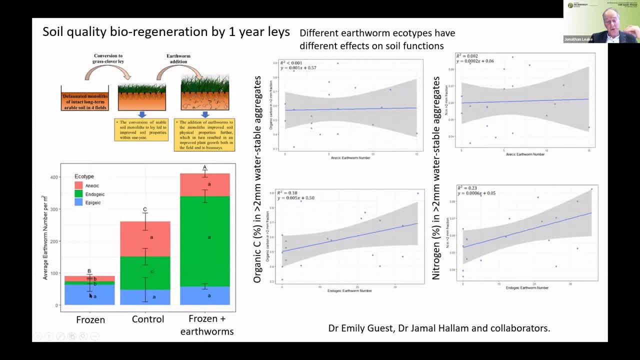 And so the frozen samples got a few earthworms in over time, but not very many. The controls which were not frozen had a moderate amount of earthworms and the ones that were frozen and then we added more earthworms back in. we managed to boost the earthworm population. So 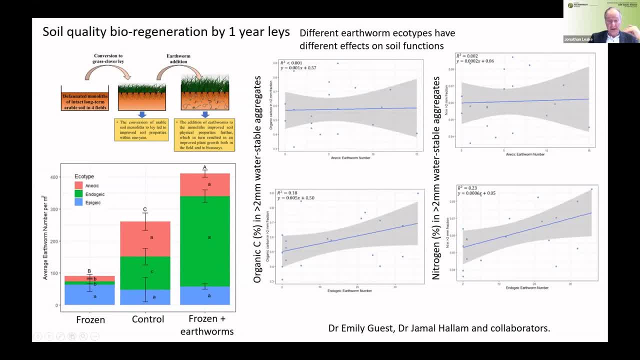 this is work that Jamal Hallam and others have done. Some of this is published and some of it's not yet published. So, looking at this, one of the key things we found was that the organic carbon in the greater than two millimetre aggregates the organic carbon in the greater than two millimetre. 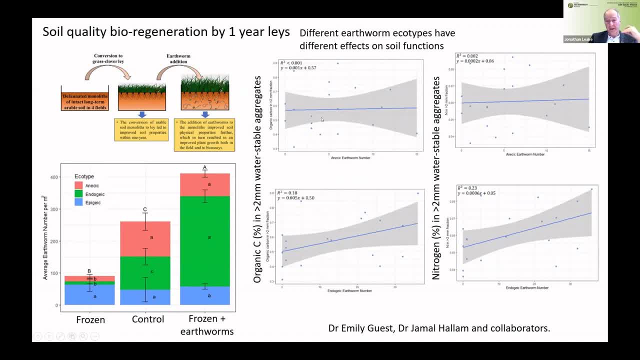 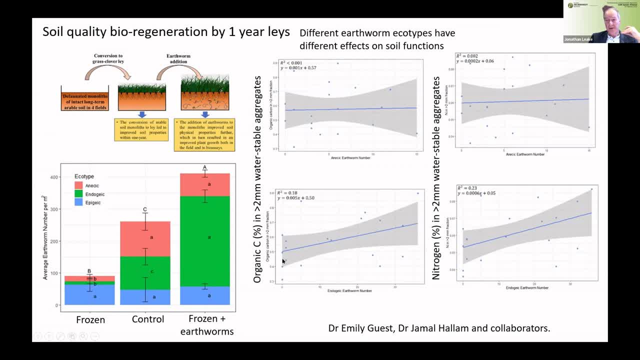 difference, but the number of endogeic earthworms, those that burrow through the soil, really was significant in terms of its effect on soil carbon storage, and the same applied to nitrogen. So I suppose one of the key messages here is: it's not just about the numbers of organisms, it's also 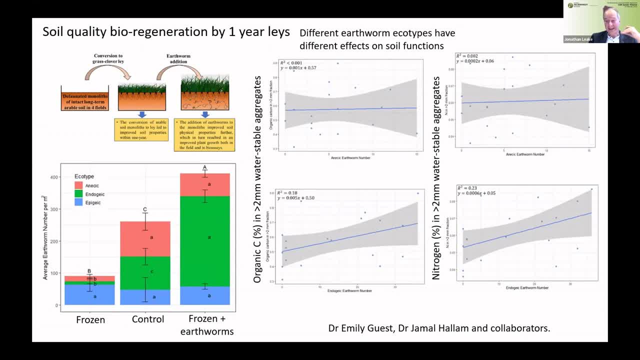 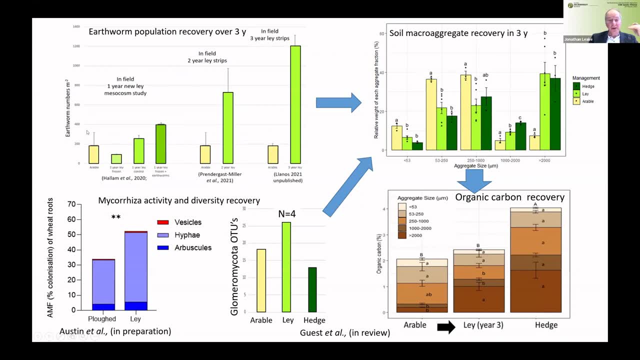 about the types and the numbers of particular types of organisms which start to become important. And sorry, this is a very busy slide, but to tell the whole story, these are the data I've just showed you in terms of earthworm numbers and then compared also to a one-year lay in the field. 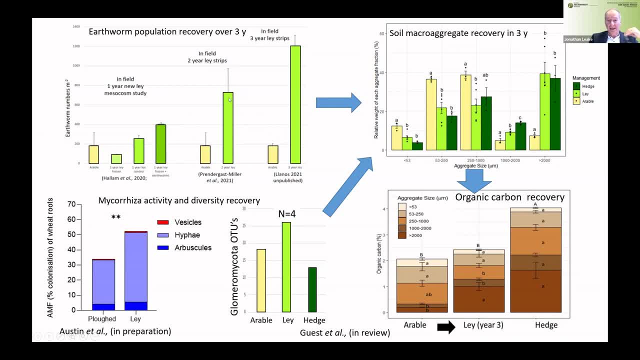 enriched with earthworms. This is what happened by two years in the actual lay strips themselves and this is by three years And you see the massive increase in earthworm populations over this time. There was a positive feedback. Mycorrhizal fungi also in terms of their 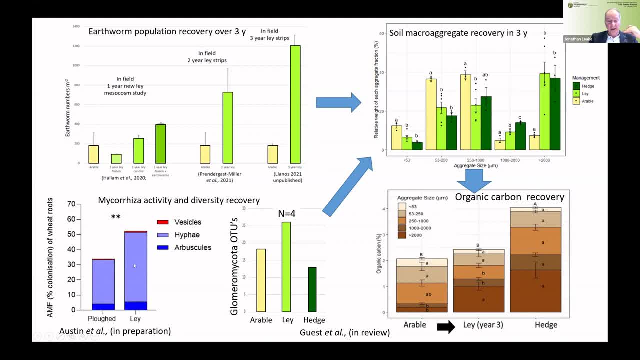 colonisation of wheat, in particular, in terms of their colonisation of wheat, in terms of their in field trials, also massively increased in the lay over a three-year period, as did the diversity of mycorrhizal fungi increased And, of course, earthworms and 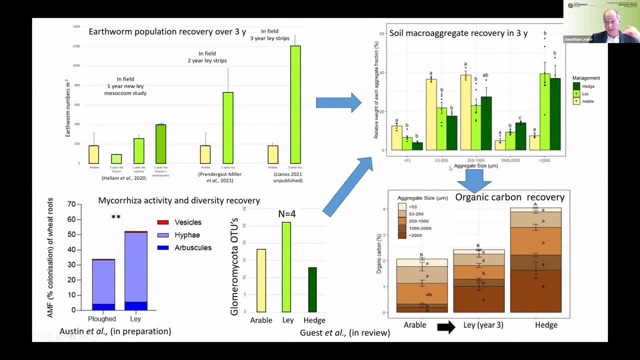 mycorrhizal fungi are implicated in helping to build soil aggregates and we see this big recovery in the larger aggregate size water-stable aggregates in this system. So the lays in this case recovered to similar values of a lot greater than two millimetre water-stable aggregates, as we 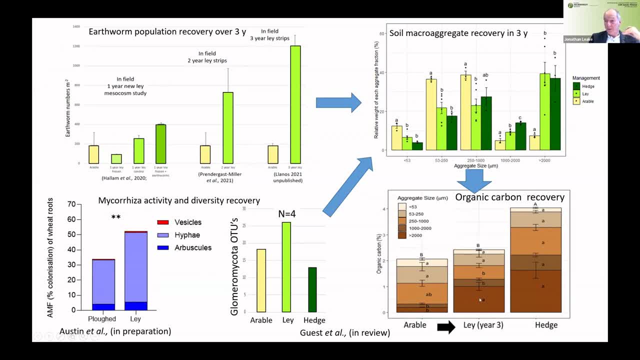 had in the original undisturbed hedgerow soils, And what we then also see is that carbon is accumulating into these larger aggregate fractions. So here we have a biology-driving structure, structure resulting in protection of carbon and the accumulation of organic matter and the restoration of some of the properties associated with the soil as a result. 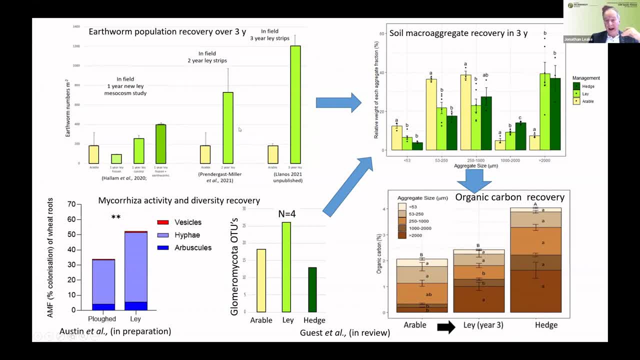 So there's a strong positive feedback. Now I highlight earthworms and mycorrhizal because we know mechanistically these are involved, But of course other organisms that we haven't tracked may also be involved in some of this. 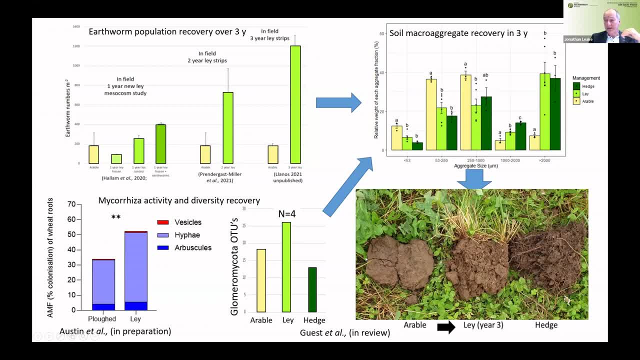 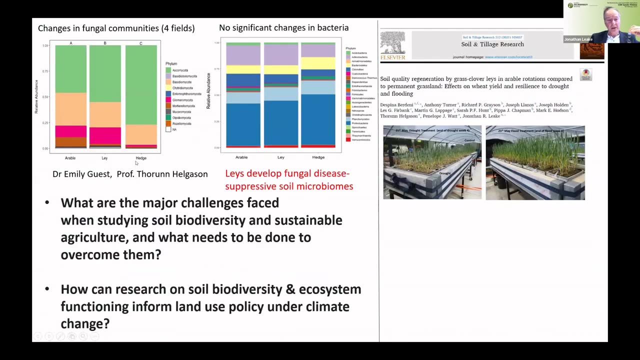 And these interactions we think lie at the heart of this kind of really substantial structural and biological and chemical alterations that we see and recovery that we see in this soil Work that Emily Guest, a recently completed PhD student of mine, with Thorin Helgeson at the 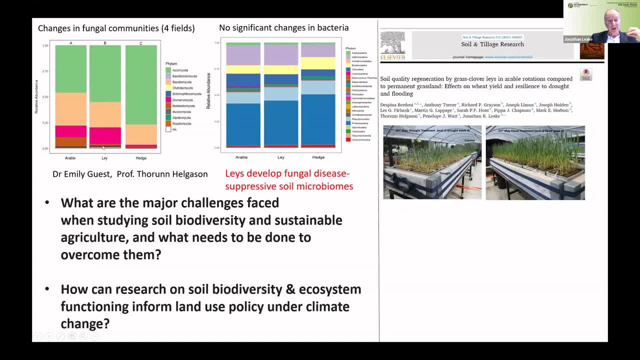 University of York. they'd looked at the communities of mycorrhizal fungi in these systems and they noted, for example, that the lay increased the diversity of mycorrhizal fungi and, in particular, the abundance of mycorrhizas relative to other fungi. 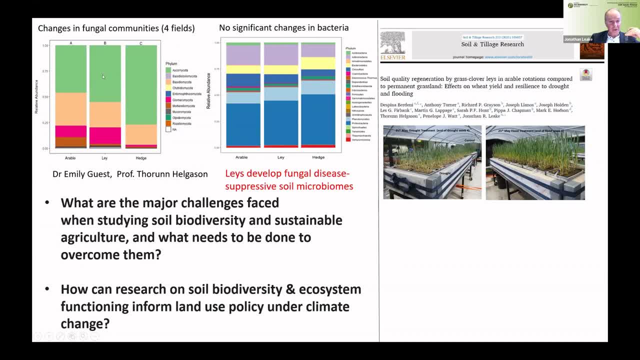 So this is arbuscular mycorrhizal fungi. these are other groups of fungi In the bacterial communities. actually, and these were averaged across four fields, there were no significant differences. There are different differences, but they're very subtle. 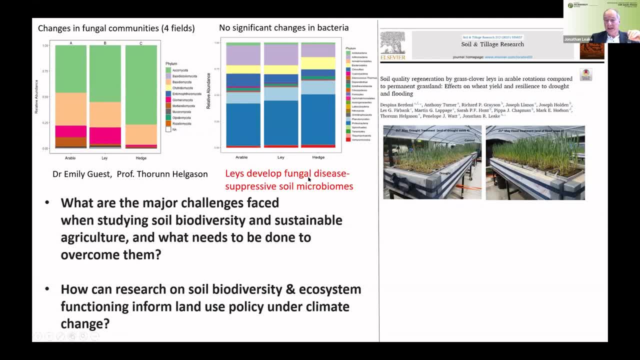 But, on the other hand, we did find differences in the amount of disease within the crops, and it was suppressed in the lays, And we know that these lays are developing disease-suppressive microbiomes. We think bacteria are probably involved in this, as well as fungi. 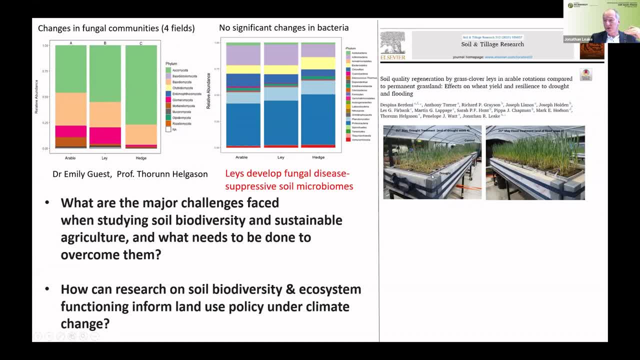 And the upshot of this was when we ran trials with wheat grown on the soil. out of these lays, what we found was really improved wheat growth, greater resilience to drought and flooding and substantially boosted yields, No doubt as a result of the nitrogen inputs from the clover. the structural improvements- 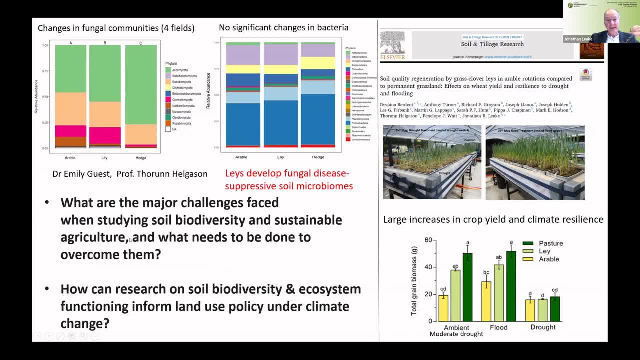 better water storage capacity, et cetera, et cetera. So, coming back to these two core questions, one of the major challenges faced when studying soil biodiversity in sustainable agriculture and what needs to be done to overcome them, I think one of the major challenges is that, clearly, in trying to characterize which organisms are, 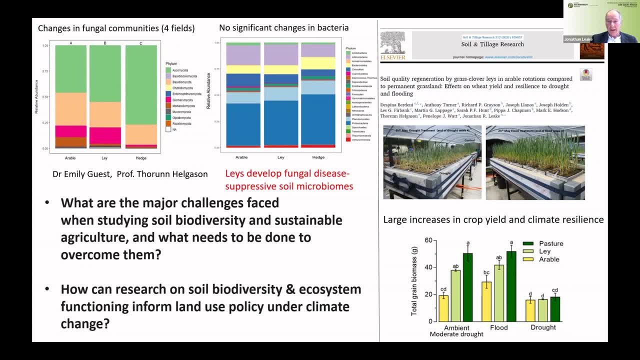 really important for sustainable agriculture. it clearly is the case that not all organisms are in important to the same extent, And so identifying key indicator organisms which are really informative and helpful is quite important, I think, because these studies, for example, on bacteria showing no significant changes, aren't really particularly informative. 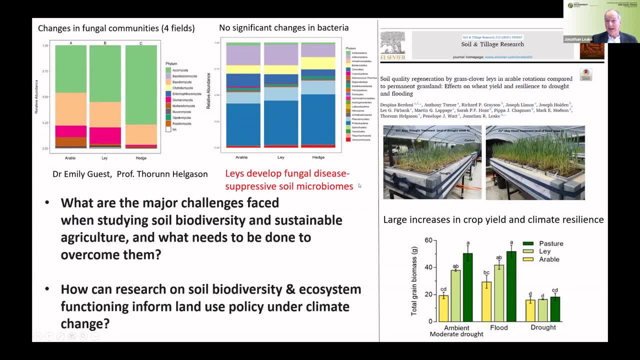 There must be other details in here that we perhaps haven't got a handle on enough, so there may be sub-components of that. Interestingly, actually, we found more pathogens in the lay but less pathogenesis in the plants that were grown in the lay, So there's. 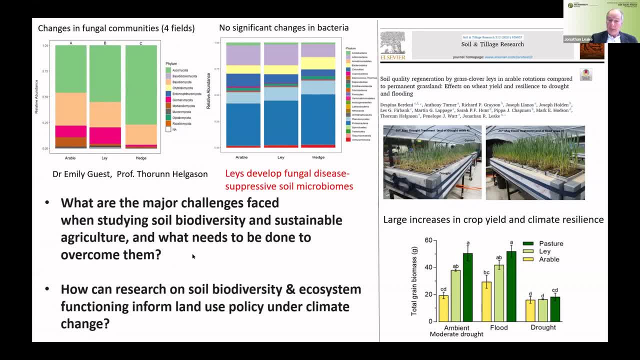 anomalies that are quite difficult to understand. really, What needs to be done to overcome them? I think we do need to focus on trying to characterize more key indicators that are useful, that really provide good ways of monitoring improvements in biodiversity, that lead to functional improvements, And how can this research lead to land use policy under climate change? Well, 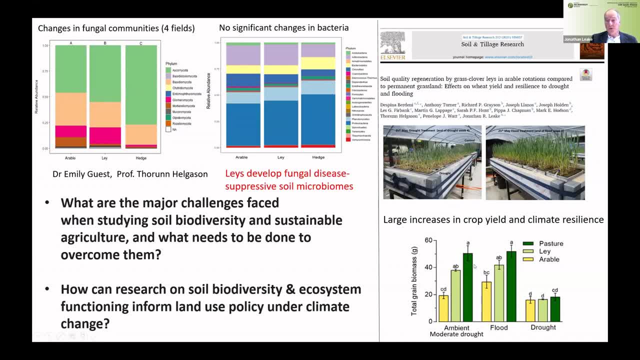 I think the sorts of research we're doing clearly indicates that if you change your management interpretation, you're going to be able to do something about it. If you change your management practices that are beneficial for key groups of organisms, rebuild soil structure. rebuild soil. 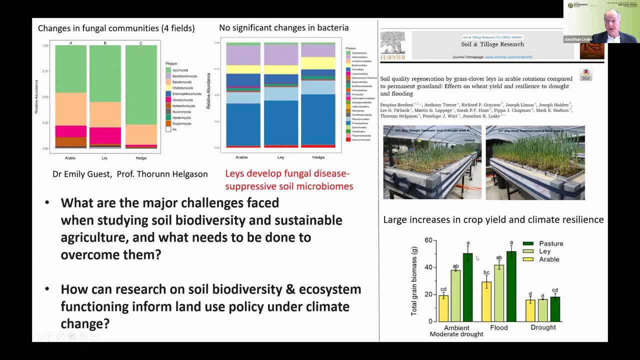 carbon and rebuild disease-suppressive soils. you end up with better yields, you end up with better water holding capacity, you end up with better soil functionality, And so I think this does directly feed into policies, And, in fact, the UK government is now providing financial support. 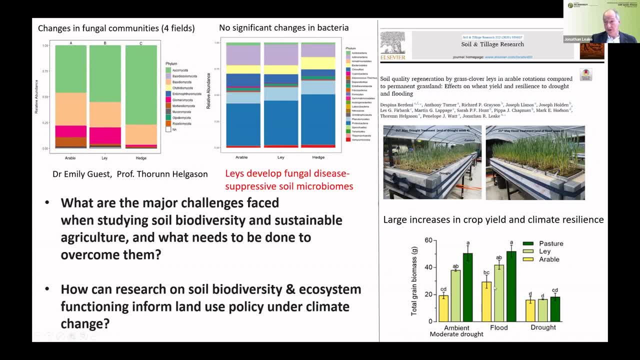 to farmers that are putting diverse lays back into their rotations on the basis of evidence such as that which we're providing from our own research. So I think there are a lot of things that need to be done. So I think there is hope as well that policymakers are actually responsive now. 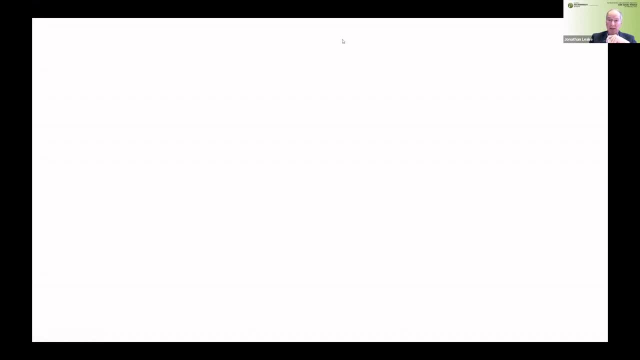 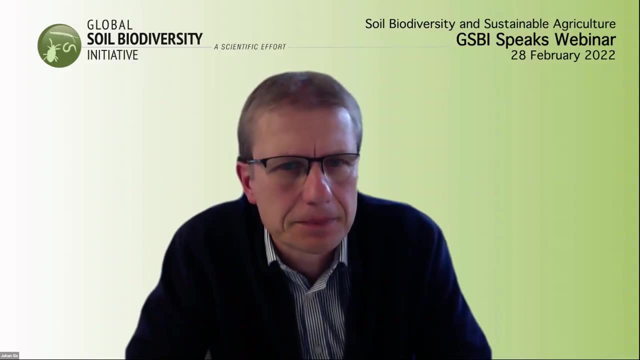 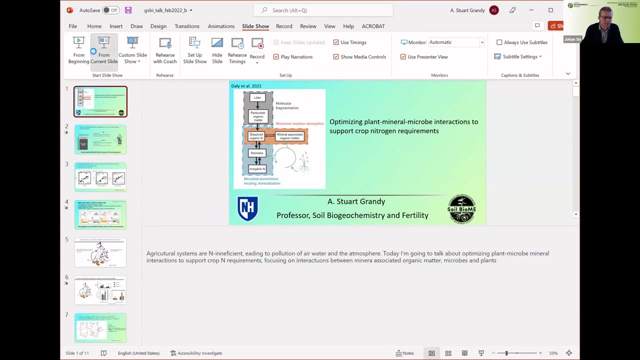 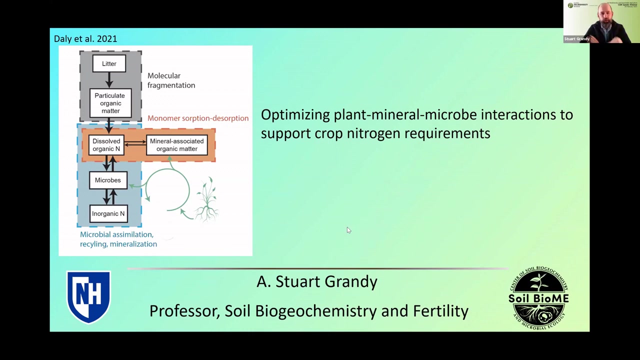 to these issues, And that's my presentation finished, Thank you. Thank you, Jonathan, If I could ask, indeed, Stuart. Thank you, Johan, It's awesome to be here. I'm looking forward to it. Thank you very much. 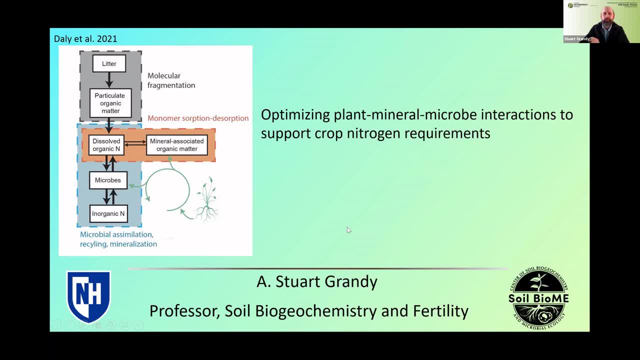 Thank you, Jonathan. I'm looking forward to the panel discussion. Agricultural systems are nitrogen inefficient, leading to pollution of air, water and the atmosphere, So today I'm going to talk about optimizing plant-microbe-mineral interactions to support crop nitrogen requirements. 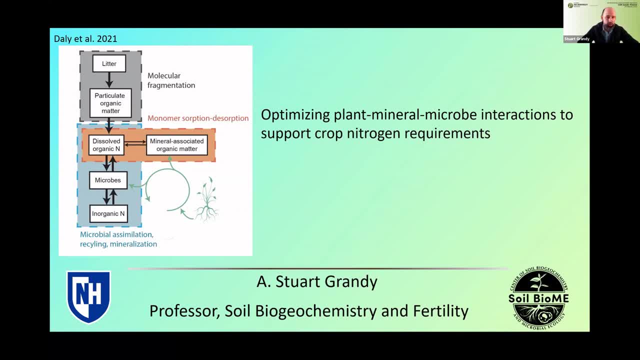 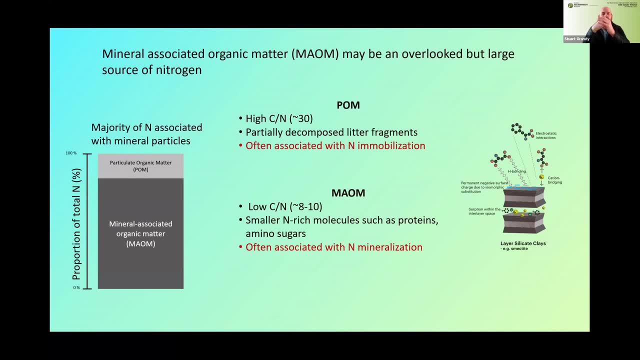 focusing on interactions between mineral-associated organic matter, which I refer to as MEOM, microbes and plants And hopefully begin to suggest some ways that we might be able to better optimize nitrogen in agro-ecosystems, making it more efficient. So mineral-associated organic matter may be an 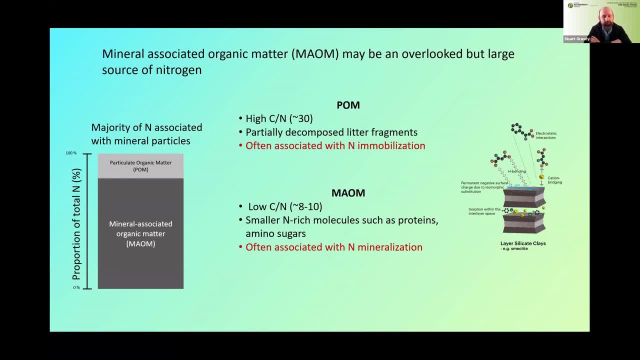 overlooked but large source of nitrogen in agricultural soils. The majority of soil nitrogen is associated with mineral particles in agro-ecosystems. It's often 80 percent or more of the total N is in this MEOM pool, which we operationally define as less than 53 microns. 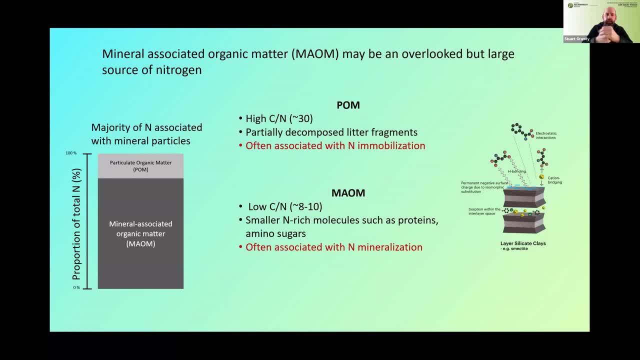 Whereas the POM has a very high C to N ratio and it's often associated with nitrogen immobilization. This MEOM pool, this large pool, is mostly proteins and other nitrogen-rich molecules, And in the laboratory it's often associated with nitrogen mineralization. And while some 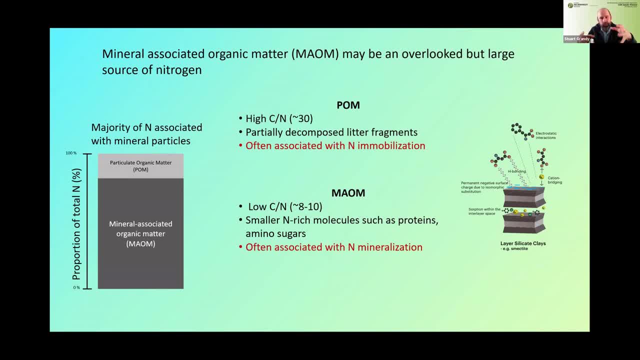 of these molecules are tightly bound to mineral surfaces. others are much more loosely associated and more available than others. So I'm going to talk a little bit about that And then I'm going to go to plants and microbes. So how do we build MEOM and what is the specific role of the? 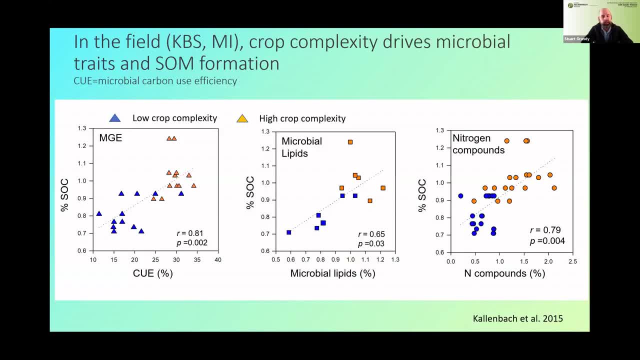 microbial community. Previous work by Cynthia Kallenbach provides some insights into this, linking microbial physiological traits, crop rotational diversity and the buildup of total soil, organic carbon and MEOM, and also specific types of compounds in those pools. Here we have seaweed, which is the carbon use efficiency of 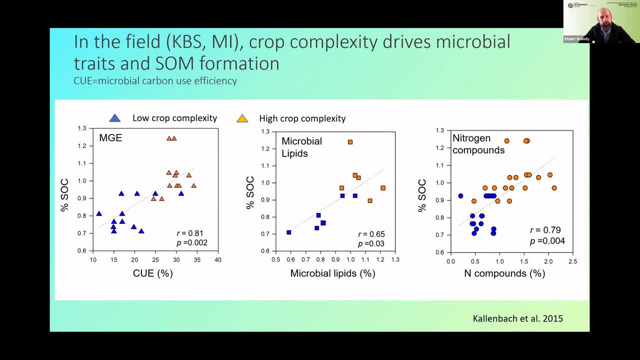 the microbes. And you can see on the far left here this positive relationship between carbon use efficiency and soil organic carbon going from a low crop complexity to a high crop complexity annual rotation. So as we get into a high crop complexity rotation, the microbial carbon use 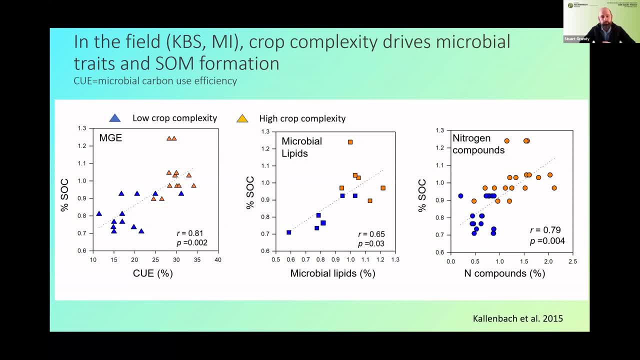 efficiency goes up And the soil organic carbon in particular. we know it's the MEOM pool of carbon and nitrogen that's building in these systems. So we're going to talk a little bit about that Now as we get into this next work by Cynthia Kallenbach. this work is done at the Kellogg. 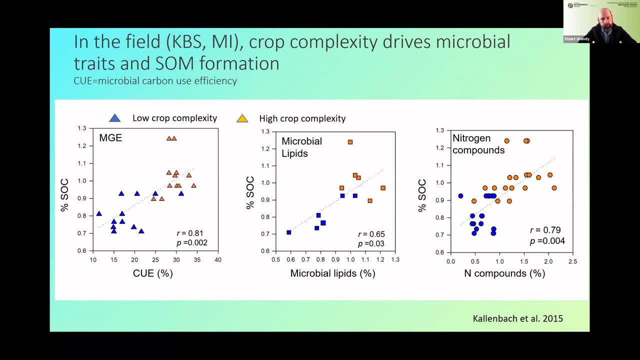 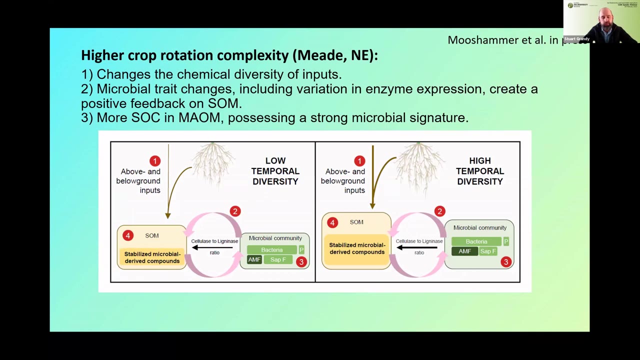 Biological Station at the KelloggቫF Center for Biological Research And in this work we'll look at the different systems that local resources in the city, the state and global cities have. So we're going to talk about those systems as a whole And then in the next work we're going to talk about the microbial carbon. use efficiency at the Kellogg Tree, at the Kellogg suddentary field and at theulated systems. We had two specific interviews and I'd like to start with the first one. We saw this increase in microbial carbon use efficiency in more complex rotations At the same time that we saw this increase. 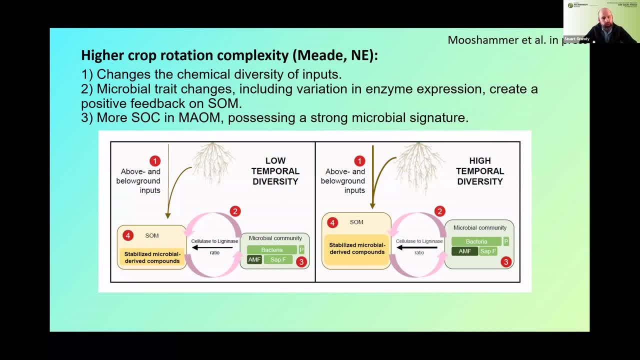 in microbial carbon use efficiency in more complex rotations. we also saw this increase in the deposition of microbial lipids and microbial nitrogen bearing compounds. in particular in this MEOM pool, high temporal crop rotations changed the diversity of chemical inputs. This specifically led to 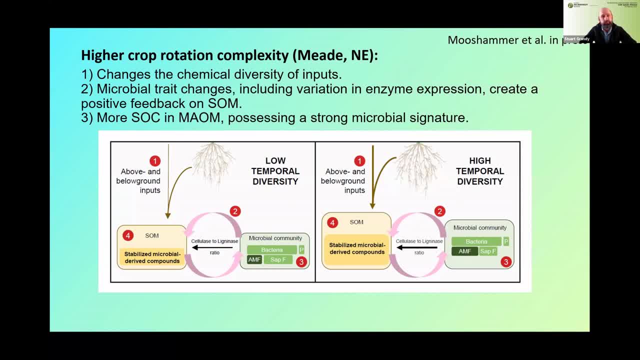 microbial trait changes, including variation in enzyme expression, changes in the abundance of AMF fungi and changes in specific bacterial biomarkers, which created a positive feedback on the soil organic matter pool. In particular, we saw more soil organic carbon in the mayon pool. 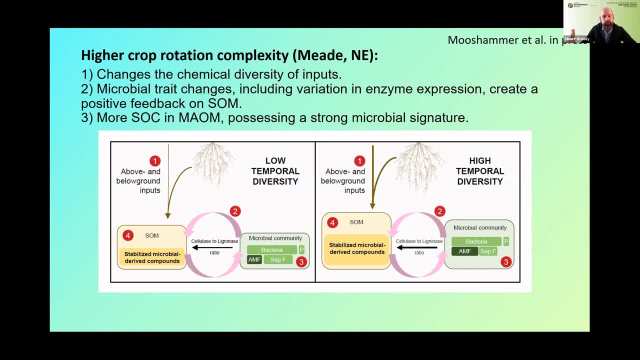 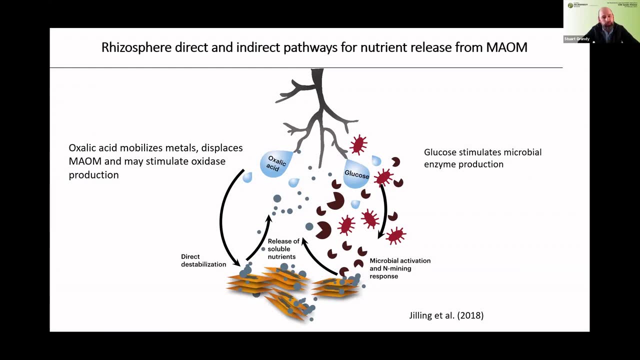 and nitrogen, and this organic carbon and nitrogen possesses a very strong microbial signature. So how do plants access mayon and what is the role of the soil community therein? Andrea Yelling provided a really nice conceptual model of this, and she proposed that oxalic acid. 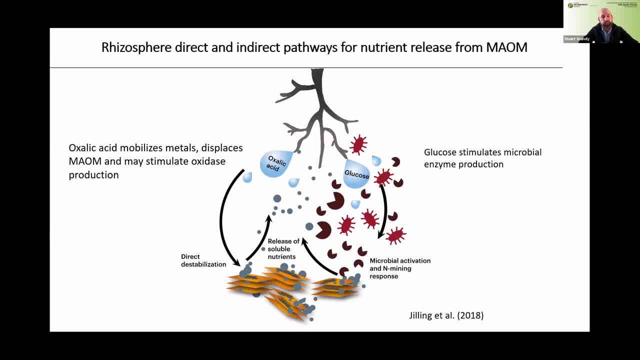 mobilizes metals, displacing mayon and potentially stimulating microbial oxidase production. Glucose, on the other hand, in the right-hand corner of the soil, is a very strong microbial enzyme. So this is a very strong microbial enzyme that is produced by plants and microbes. 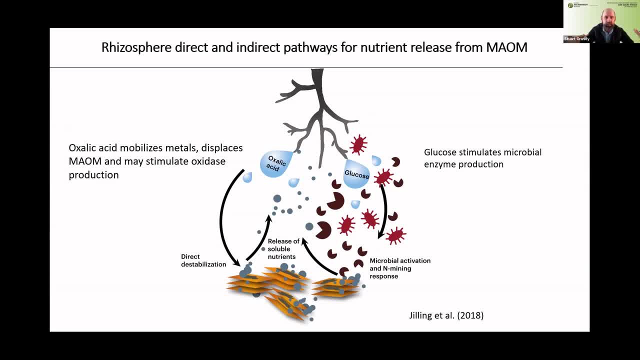 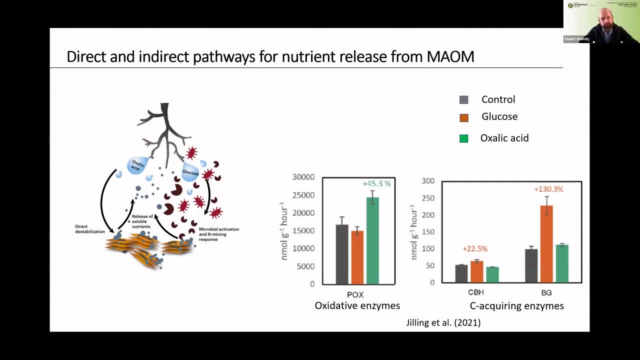 stimulates microbial enzyme production, and both of these separate pathways are capable of mobilizing mayon and making it more available to plants and microbes in the rhizosphere. So Andrea followed up this work, looking at these direct and indirect pathways of nutrient release from mayon, and she added glucose and oxalic acid to soils from Illinois and she saw that. 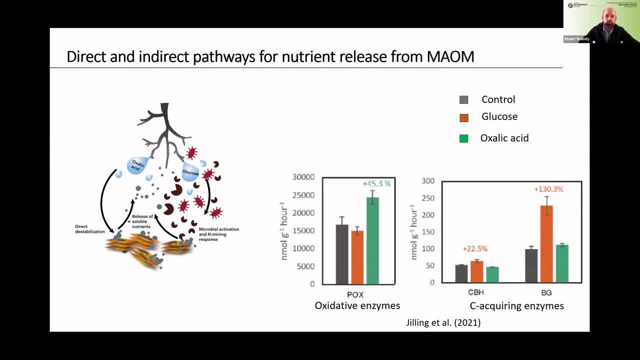 oxidative enzymes increased with the addition of oxalic acid, whereas these carbon-acquiring enzymes increased with the addition of glucose. Interestingly, very consistent with her original conceptual model, she also saw the mobilization of iron and aluminum in solution associated with oxalic acid additions, suggesting again this pathway whereby oxalic acid may be mobilizing. 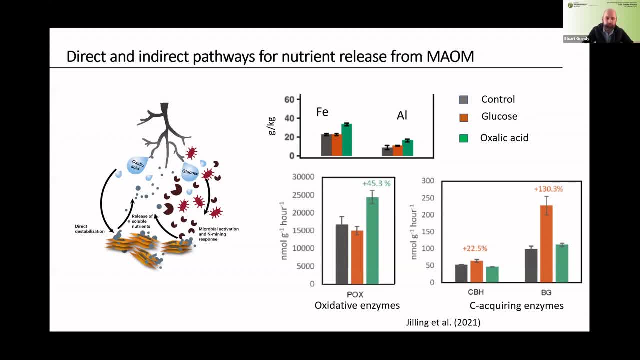 mayon, carbon and nitrogen, And indeed in this study there was a lot of interest in the study. Both of these separate pathways stimulated mayon, carbon and nitrogen priming specifically from the mayon pool. So then we followed this up in a recent study at the 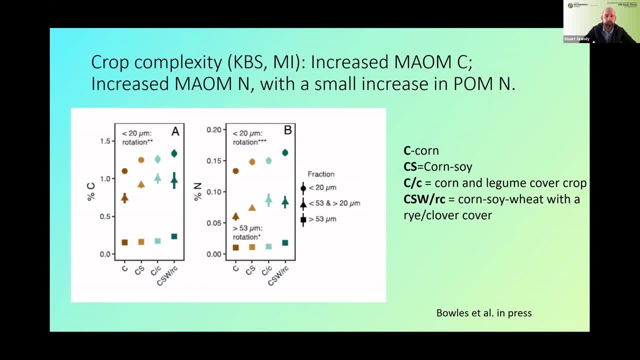 Kellogg Biological Station in a crop rotation gradient going from corn to a corn-soy-wheat rotation with a rye cover crop, Not surprisingly we saw both total carbon and nitrogen increasing with crop complexity. but here is the very finest fraction: It's less than 20 microns. 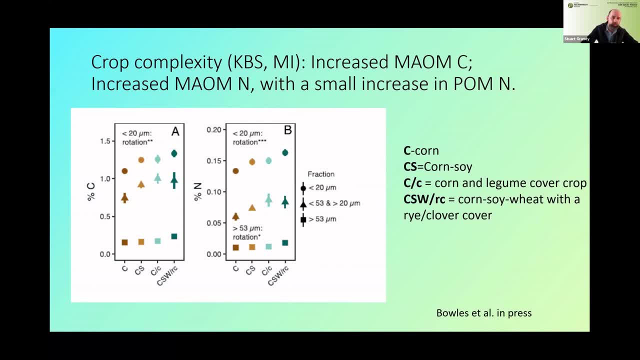 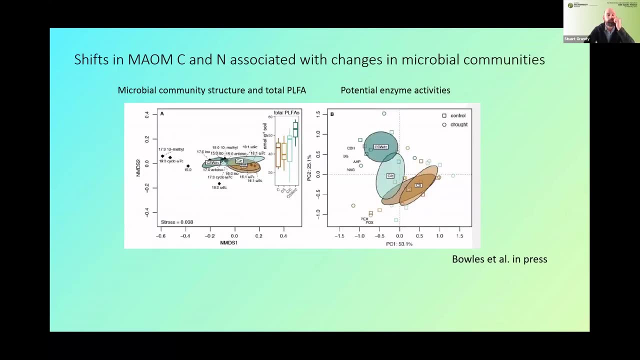 This is the fine mayon fraction. This is where we see most of the carbon and nitrogen gain along this rotation gradient at KBS. So most of the nitrogen gain is there in that mayon fraction. These are sites that are not fertilized. We also saw along this gradient a shift in the 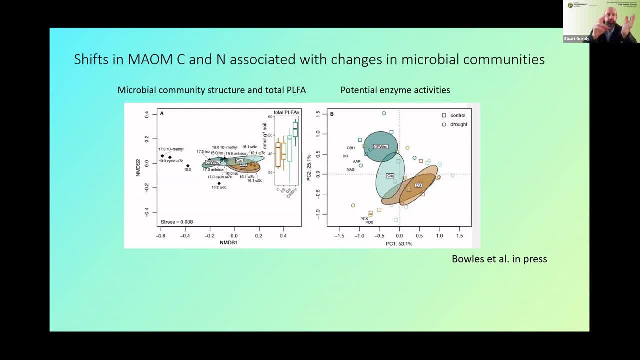 microbial community structure. So we saw a shift in the microbial community structure Again, changes in AMF, changes in actinobacteria and gram negatives and a massive shift in potential enzyme activities, with a switch in the carbon acquiring to oxidase ratio across. 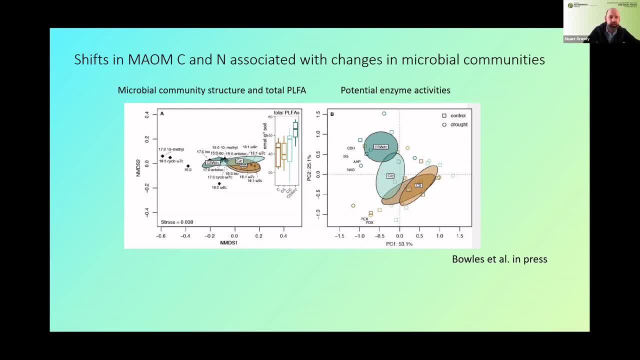 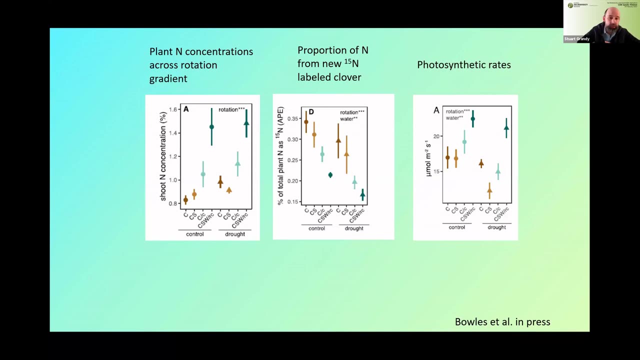 this gradient. So again, crop complexity, shifting microbes, microbial investment and carbon acquisition. And so how did this impact crop nitrogen uptake from soil, organic matter and new sources? So this is the plant nitrogen concentration across rotation gradient in the greenhouse. These were not fertilized plots. You can see here that this complex rotation had a much higher. 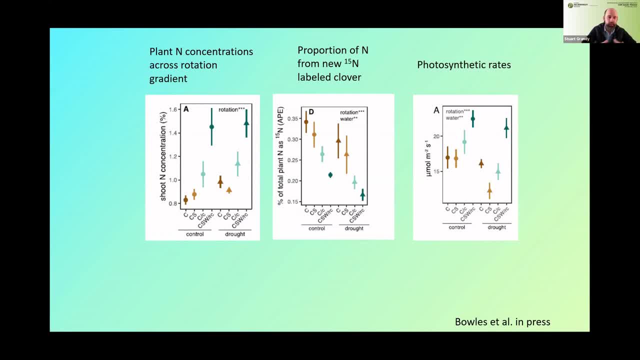 capacity to take up nitrogen and has got a much higher nitrogen concentration. We added 15N clover residue to these soils to look at the nitrogen uptake of new versus old soils. So this is the plant nitrogen concentration across rotation gradient in the greenhouse. It cámる, a mustlifeurious load of he acne-resistant soil, organic matter, which is what we were giving the実 talk about earlier, And this for in this mix. you can see that what the sor woke looks verylassive. It striated off the organic mass right around the damn color in phase. 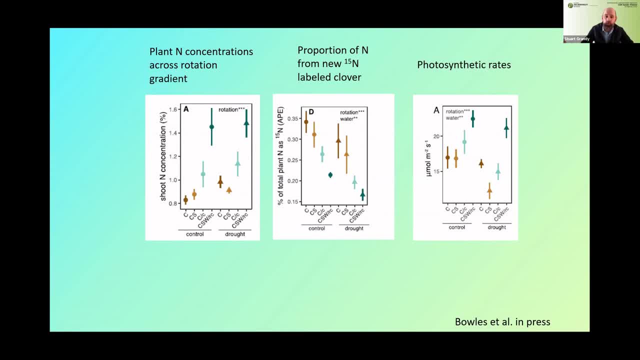 Here's a sample of our micro incompatibility: for the central maionic BMW, for the veget Mango harvester aunt, where we kind of lateralized that glacial large soil organic matter and You can see in this more complex rotation the plants are. 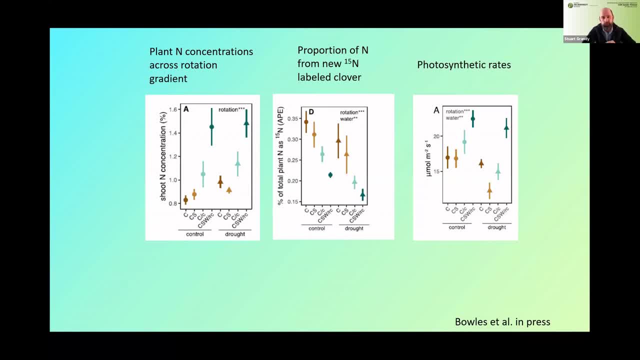 very happy getting the majority of their nitrogen from the existing SOS pools, the majority of which are may of nitrogen. We also saw much higher photosynthetic rates and productivity in those complex rotations, And so we saw overall the complex crop rotation and increased mase. 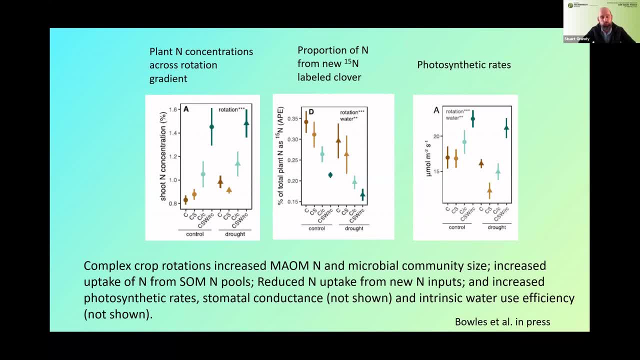 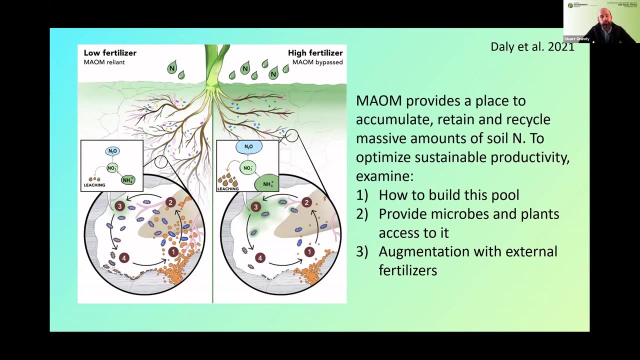 They increased uptake of nitrogen from soil, organic matter nitrogen pools, reduced nitrogen uptake from new nitrogen inputs and increased photosynthetic rates, stomata conductance and intrinsic water use efficiency. Mayom, we think, provides a place to accumulate, retain and recycle massive amounts of soil nitrogen. 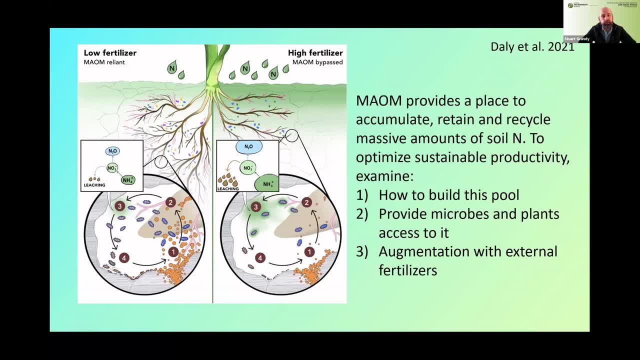 I think, to optimize sustainable productivity, we have to continue examining how to build this pool, how to provide microbes and plants access to it. what are those mechanisms? and then, how do we go about augmenting the internal recycling of nitrogen with supplemental fertilizer use? 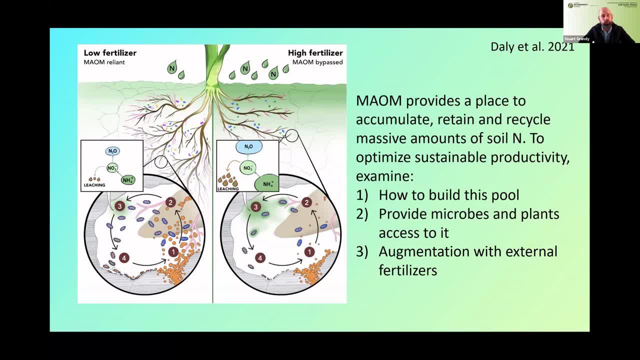 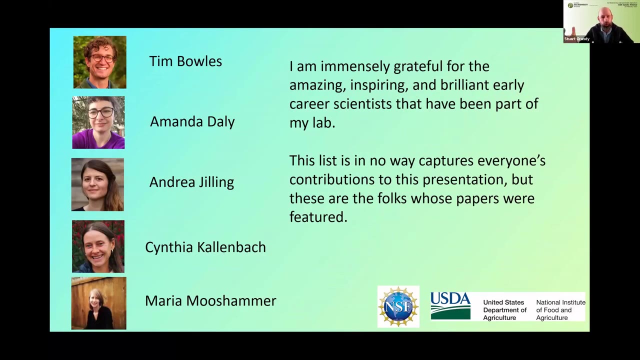 As this graph shows, what we're looking for is to have internal cycling of nitrogen plants and microbes accessing that Internally Internal nitrogen and augmenting that pool just enough with external nitrogen additions to replace lost nitrogen. And with that I'm just going to toss out this acknowledgement slide for all the people who actually did the work that I presented and turn it over to Johan and the panel. 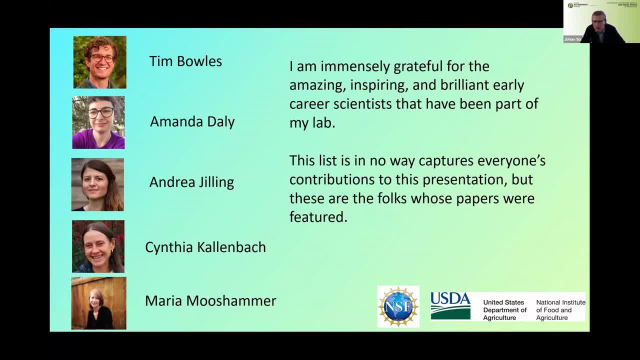 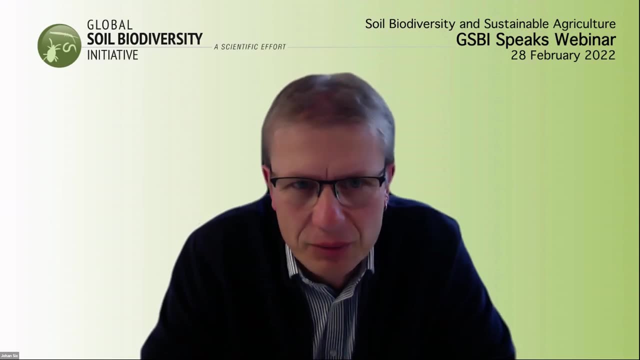 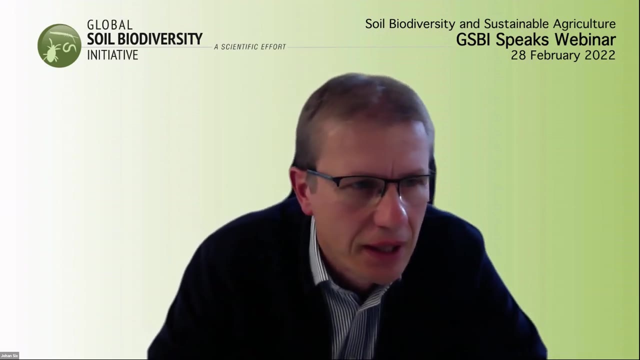 Thank you. Thank you very much, Stuart, And actually I want to thank again all of the presenters, the panel, Because obviously it is quite a rich, you know presentation by everybody that probably stretch your mind from, from you know, quite across the board a bunch of different subjects and I hope you you understood most of it. but I see also that we indeed have quite a bit of questions coming in. 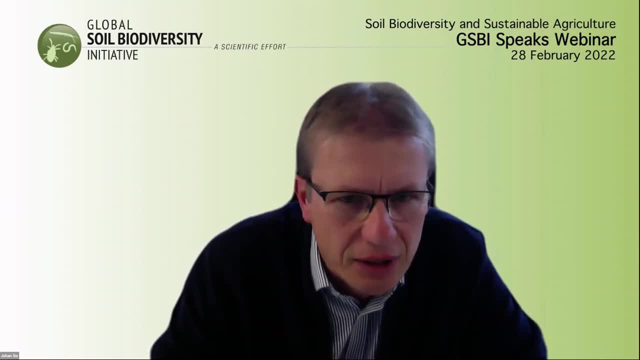 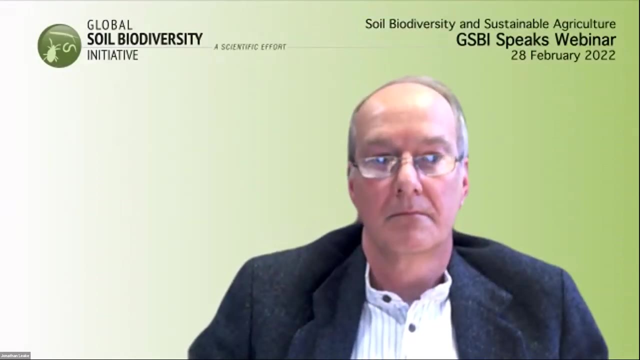 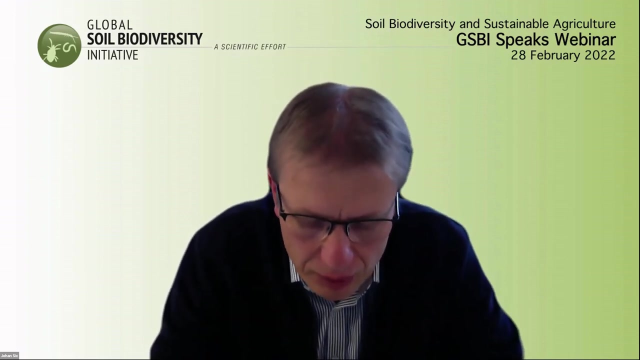 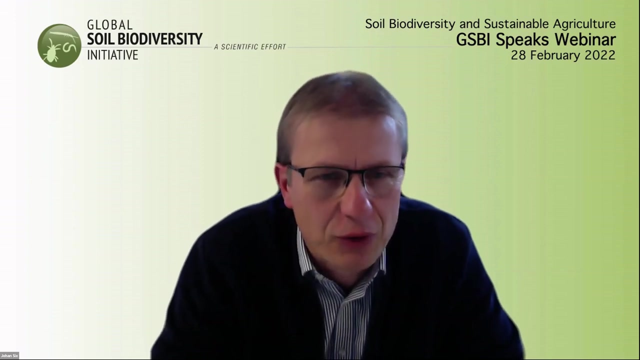 And so I would like to invite, actually now, all of the Panel members to put on their video so that we can have a discussion, you know, with with the audience. So thank you again, and I guess I first question that I see, and that was somewhere to be expected- is indeed that that would you know? what are really the indicators of soil biodiversity that are valuable for farmers? 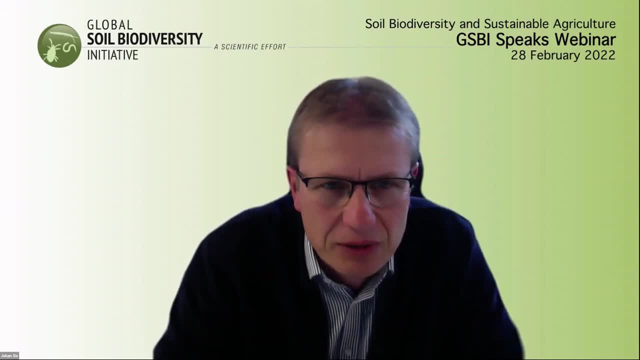 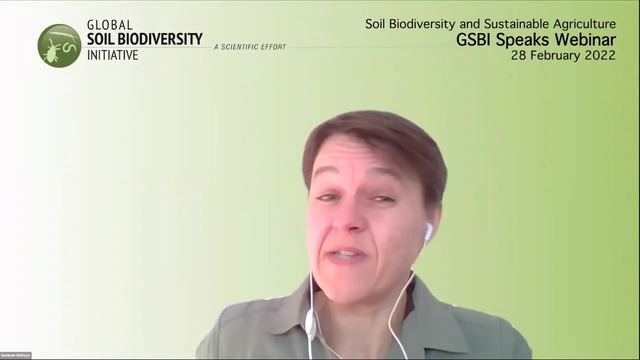 And so I guess I would like to Maybe invite her, Linda, and or Jonathan, to give an answer to what are these indicators now that farmers, you know can't, can relate to, And you then mean specifically the biology? or I mean, I guess the first one would be: but to a certain level, soil organic matter is quite related to soil, microbial biomass, for example, but that's not a continuum. 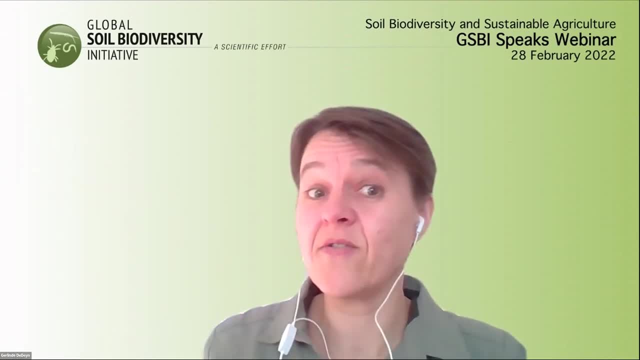 So that is when you are at the low end, But for the very first time, I think that that's a good indicator. I mean, I can, I can't, if you know, if, if you're just a farmer and the land is a good indicator. 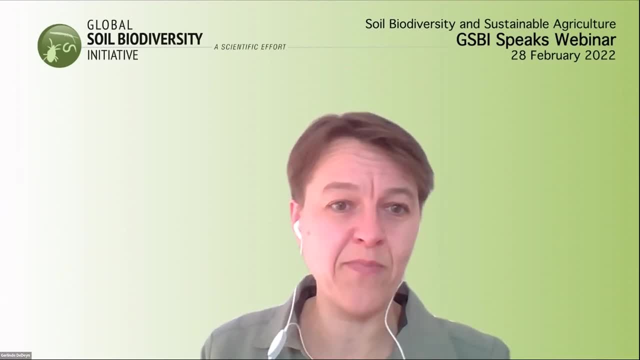 And that that is a good indicator. All the things like pH Can also really help. I mean also when we look at papers from within fields, but also across fields, across the globe. PH is quite a An important indicator in terms of community composition of microbial. 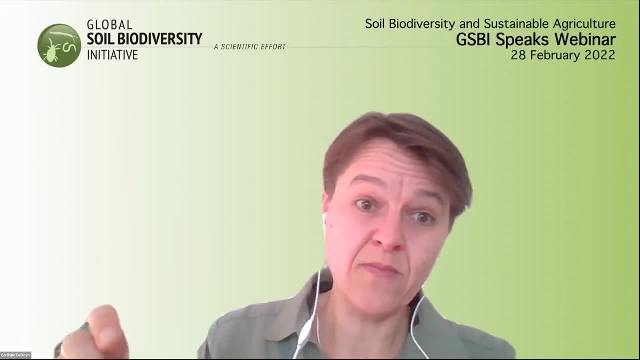 Communities and even abundances. If we go beyond that, then, for example, if a farmer, even in situ, QPCR type strips, you can insert in your soil at certain locations and get a measure of what is the starting point of your level of disease. 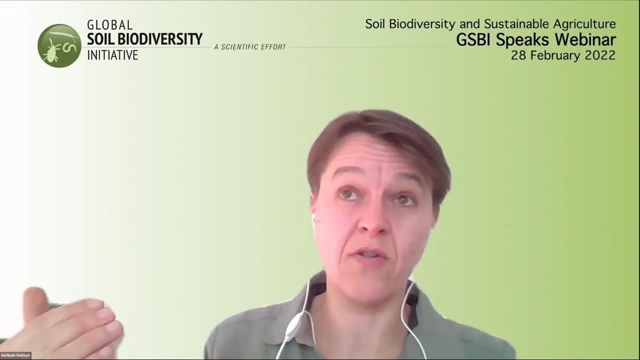 and do you need to be afraid there and choose another crop or something, or is it still below the threshold? So it will depend a bit on your specific question, and the ones I just mentioned now are still relatively general in relation to your specific crop. 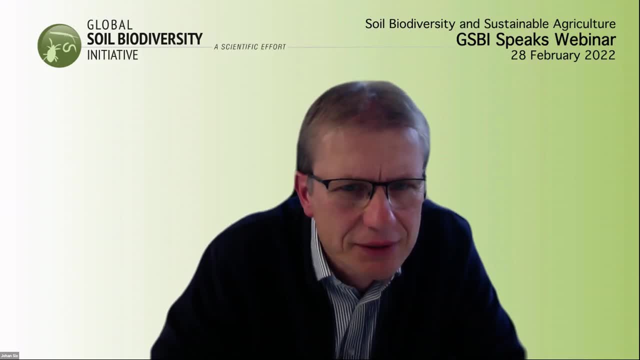 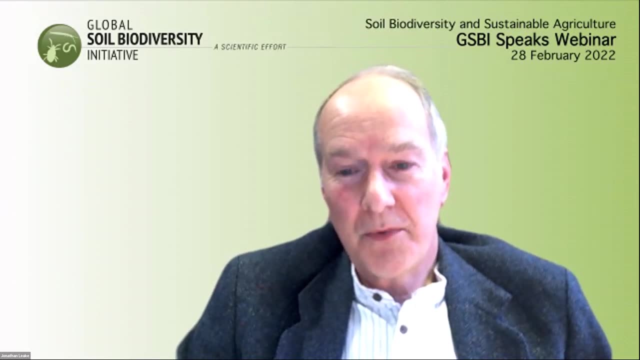 Thanks, Janine. Maybe Jonathan, if you want to add something. I think one of the major indicators that's often recommended are earthworms. I think the issue with earthworms is that they are seasonal and so if you go out in the summer and it's very dry, 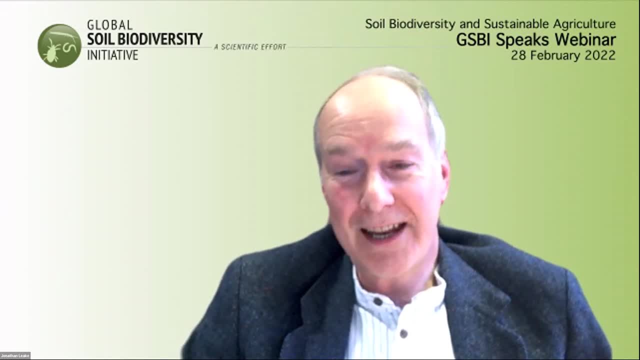 don't expect to find large numbers of earthworms. So there's an environmental context to earthworms. but if you are routinely monitoring your fields- in the early spring, for example, when the conditions have been moist for a reasonable period of time- 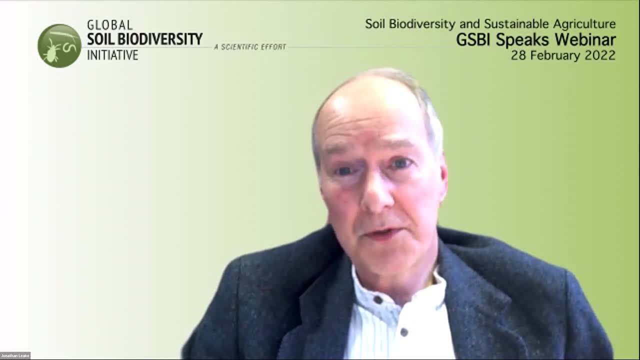 you can do year-to-year surveys that begin to tell you if your soil is more active in earthworms- And I think earthworms are good from a farmer's point of view because they can see them. they generate large biopores. 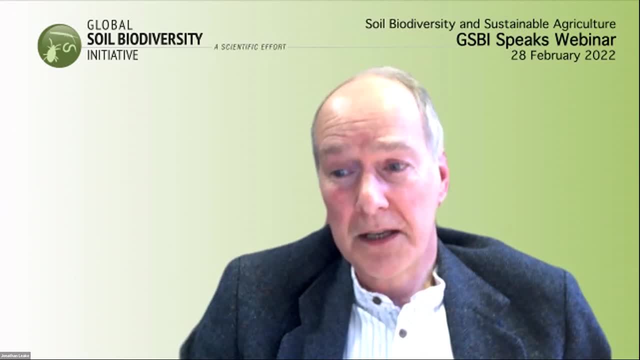 which are important, and they're important for cycling nutrients and soil And also, as I say, improving soil structure. So I think they're a good initial indicator for a farmer, because you can actually see it yourself in the field and you can make records. 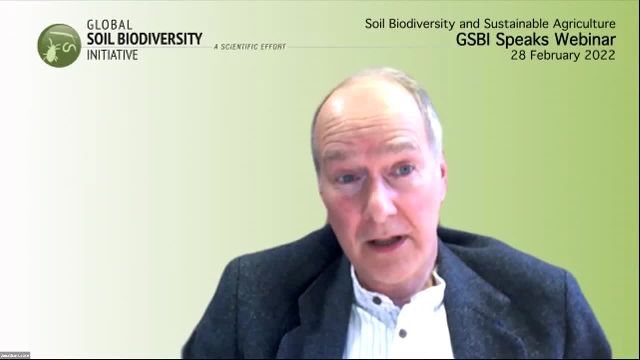 And if you have a standard protocol for extracting and measuring those which you apply routinely, then I think that's great. The other thing I would recommend is doing visual assessment of soil structure, because I think if your soils are well structured and the aggregates are coming together well, 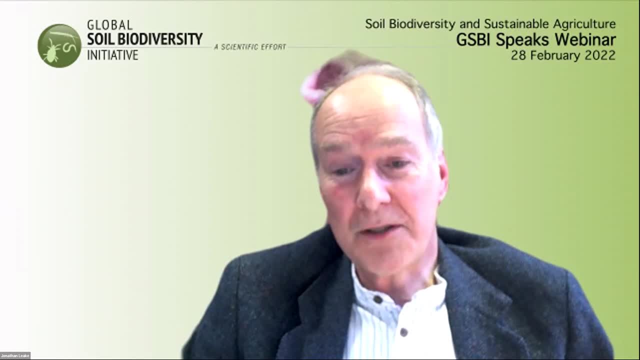 you've probably got the biology mostly right And if the structure is bad, then there may be a number of reasons for that. But the chances are that the bad compacting structure and disaggregating structure will actually lead to poor biology and you'll end up with pathogen problems. 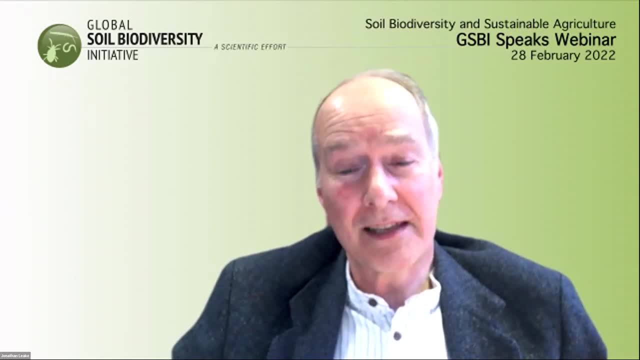 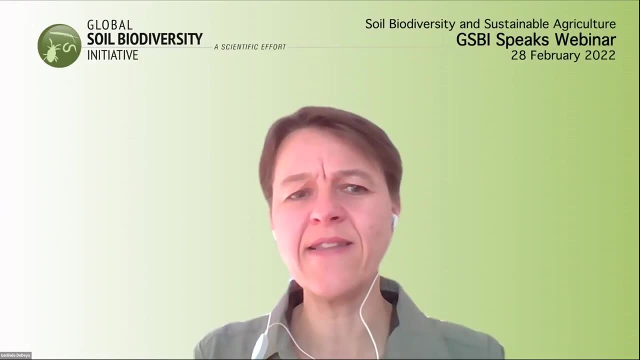 and you'll end up constraining some of the better organisms. So that's another way. visually, you can do things in the field without having to send off for lab tests Like rooting density. I thought that was also an interesting one. that can be very visual. 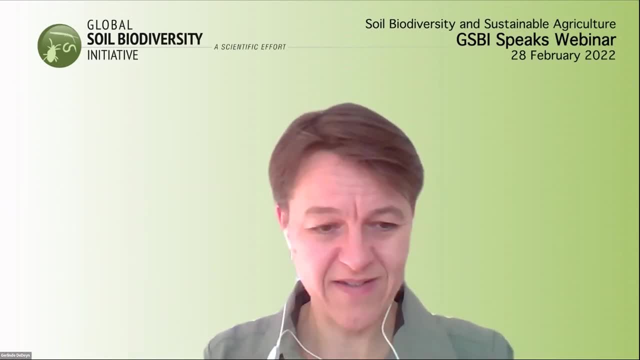 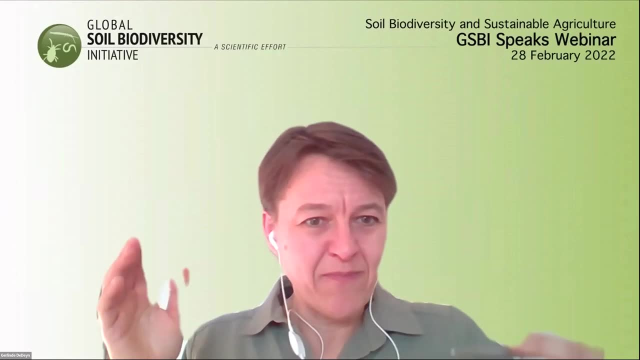 And that's where the food is going. indeed, Yeah, but that's a bit more tricky to measure, as we all know. the root density: Yeah, but maybe if we build that up a bit with taking images and make a certain reference collection, 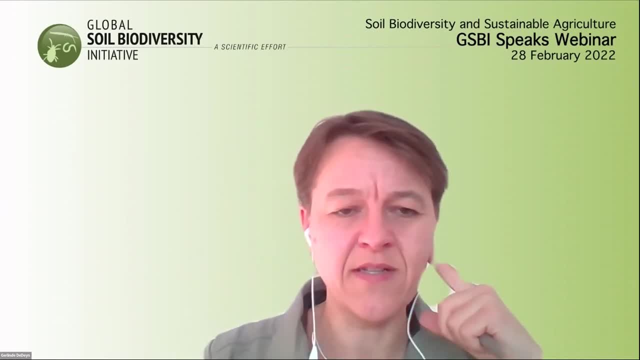 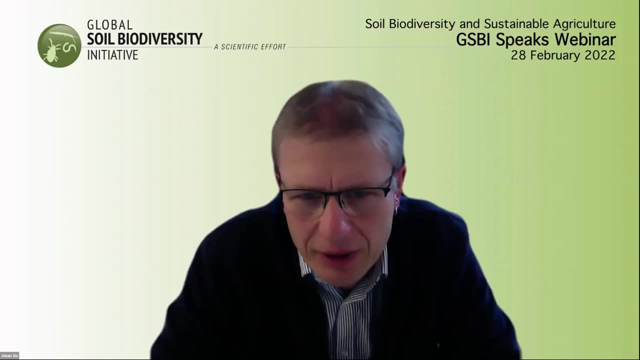 I guess farmers also become more digital in that respect. and the comparative development, Yeah, correct, I mean I guess, Sarah and Stuart, if you have any others that you think from your studies, that you think is a very good indicator. Yeah, a brief comment on soil earthworms. 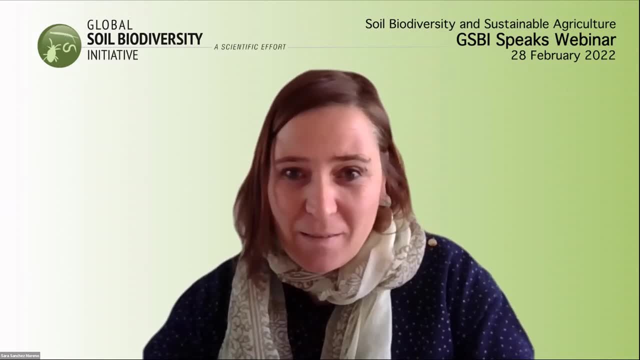 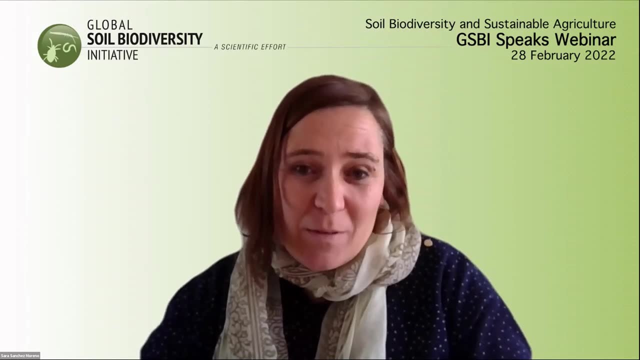 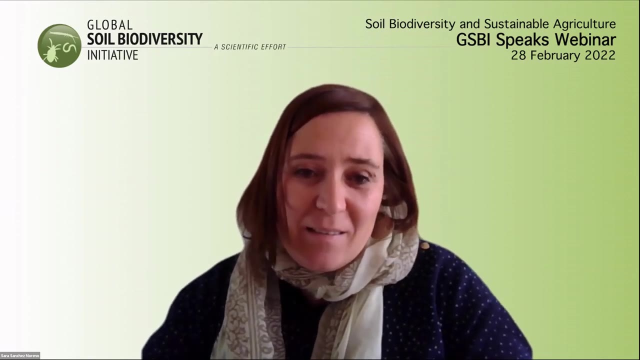 which play a fundamental role in many agricultural systems is that in arid and semi-arid systems many times earthworms are almost absent. So in Southern Europe, for example, earthworms are absent from many agricultural systems. So in those systems to have MS or biological activity, 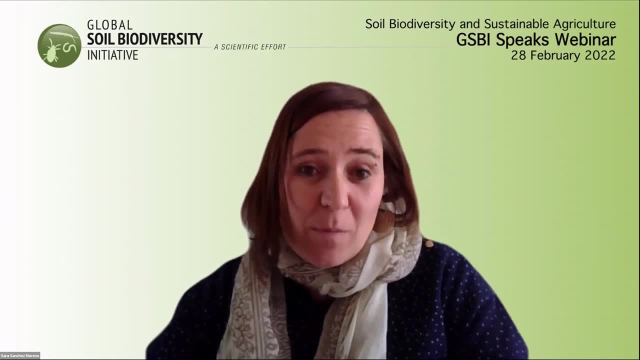 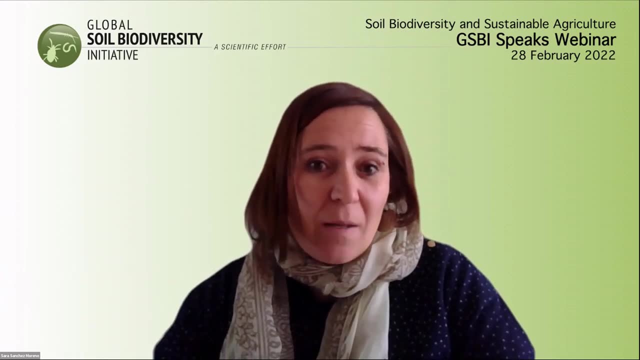 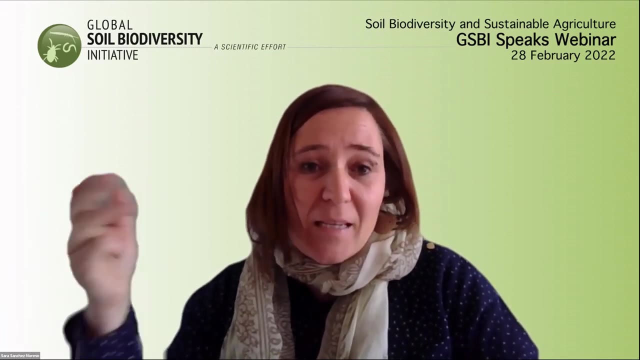 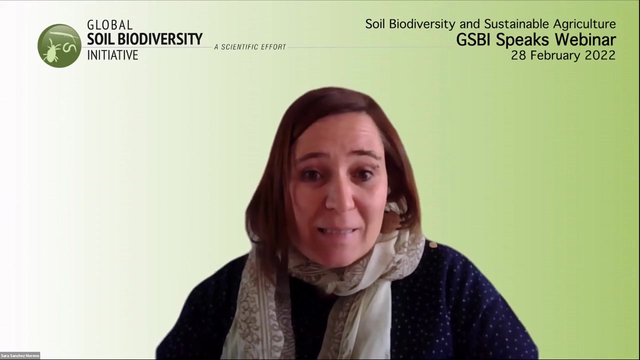 and other indicators could be used which are probably more difficult to see more with the eye than earthworms, such as arthropods, beneficial nematodes or enky traits or other organisms, even ants or other arthropods, But also in these systems. 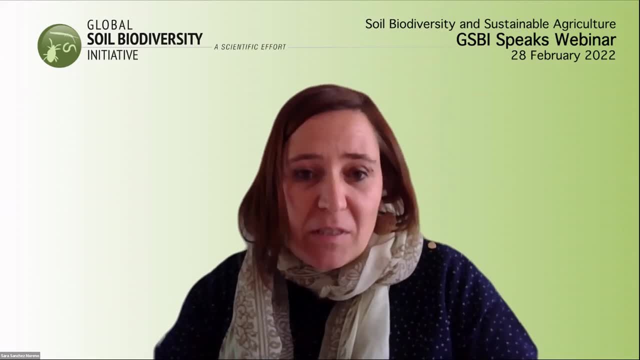 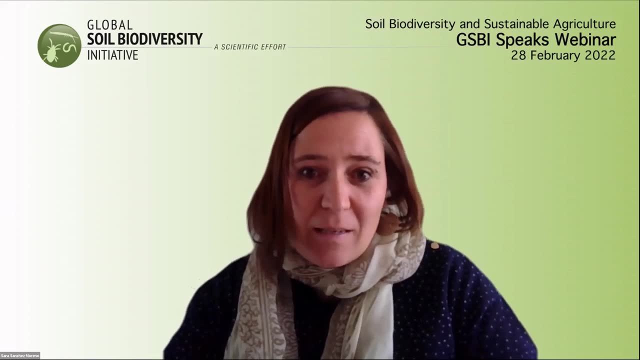 assessing visual soil structure might be very, very, very, very useful. And of course, as Gerlinde said, organic matter. the amount of organic carbon in soil is, in my view, the best, the first indicator of soil fertility and soil structure in most systems. 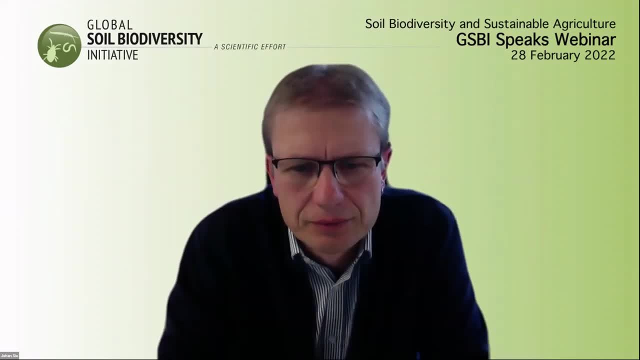 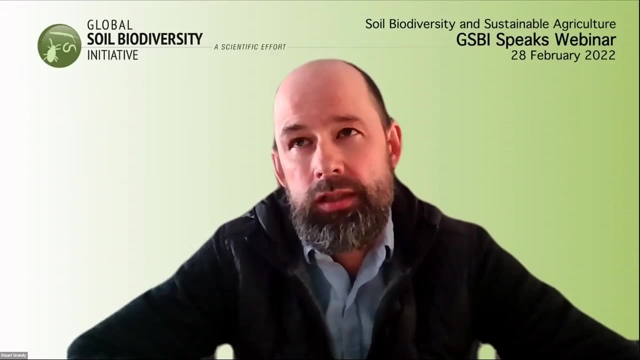 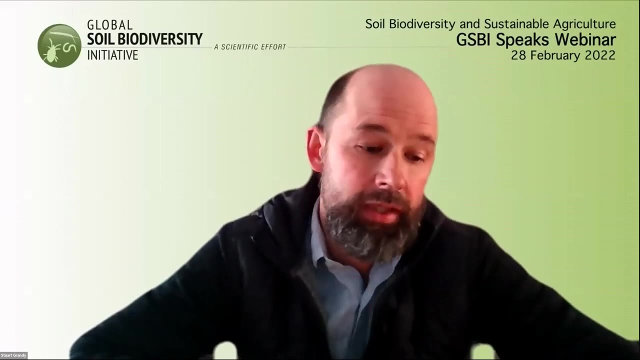 Yeah, Yeah, I have a quick thought on this. I would say the most consistent indicator that we've seen- and this now extends back a number of years and over many, many studies, and it may just be the types of measurements that we make. 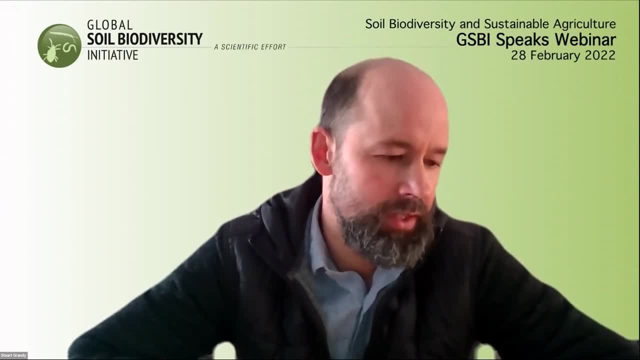 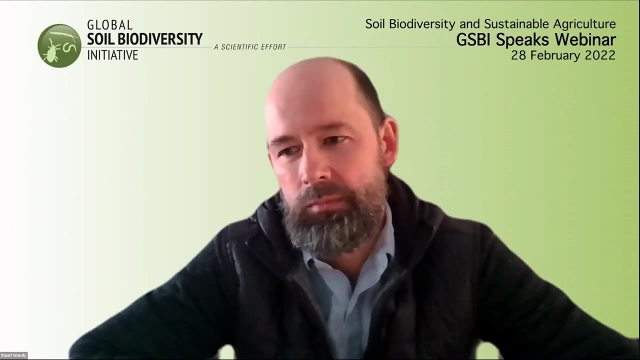 is the ratio of enzymes that we would call carbon acquiring, like beta glucosidase and cellulose, degrading enzymes to oxidases, things like phenyl oxidase and peroxidase, And over and, over and over again, we see as the soil becomes depleted. 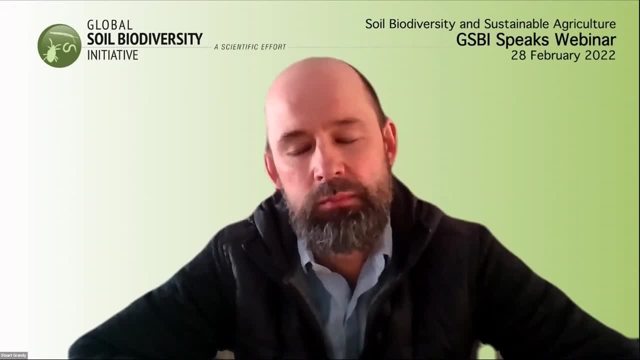 there's more microbial investment in the oxidase enzymes And we could, you know, talk at length about the mechanisms behind that, but we can save that for another day. But we do see that across lots of different cropping systems, gradients, now that we've studied. 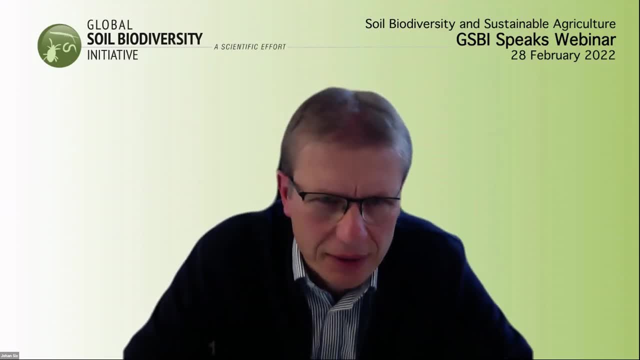 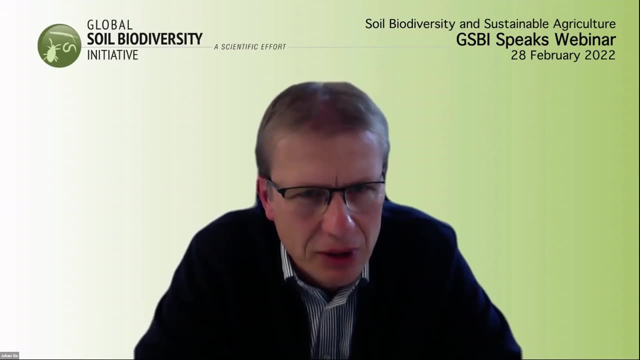 Yeah, I mean, Sarah, actually, since you brought it up in dry land, you have these, you know, so you have to think about some other soil indicators. But there's actually an interesting question also from the audience that is asking, like you know. 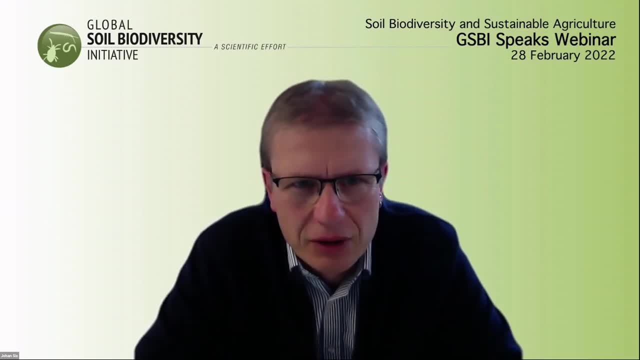 which soil biota would you really like to improve in irrigating? So you know you're under dry conditions, That's when you're using irrigation, And we know that irrigation is not always very beneficial. But so how do you do? you know? 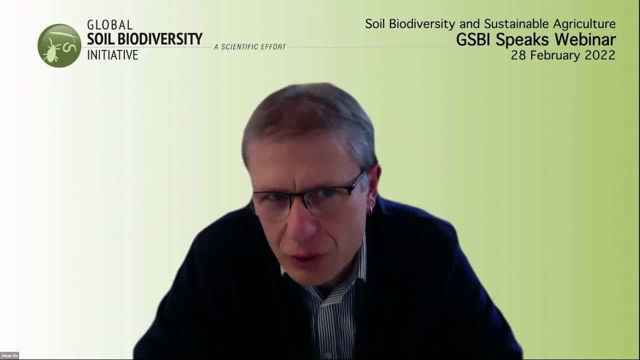 your improvement of soil biota under those conditions. Any thoughts, Or maybe somebody else, if Sarah is not ready to take on the question? But irrigated soils are an interesting one. Yeah, Yeah, I don't know if I understood. the question is: which soil biota? 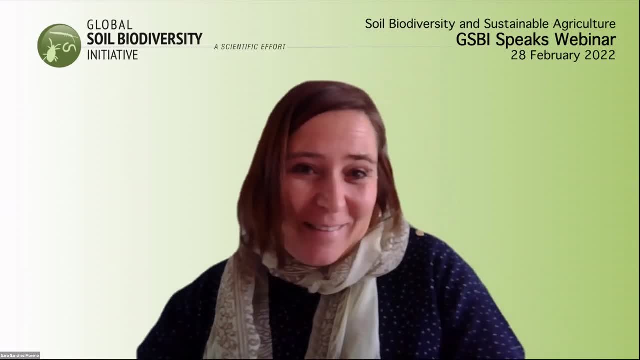 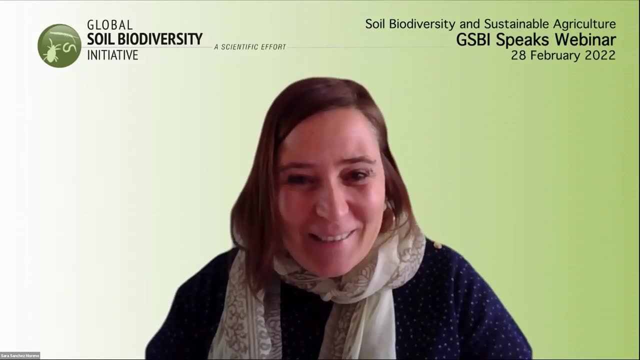 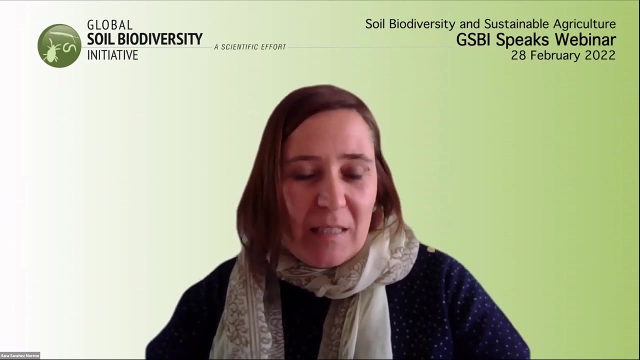 do you want to increase in irrigated systems? And I would say basically all of them. I mean, I don't know how should I choose one? So, as we've seen, basically most soil organisms play beneficial roles on nutrient cycling, carbon sequestration. 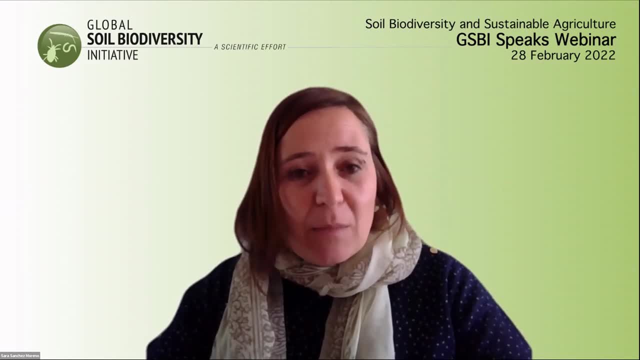 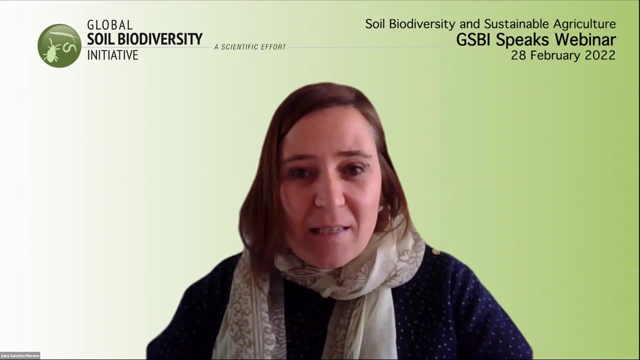 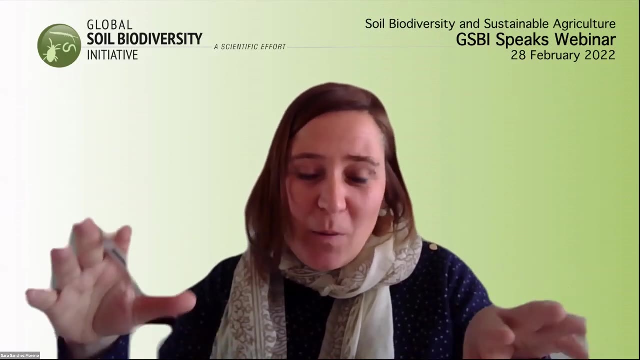 crop, biomass and crop yield. So, for example, soil animals. I've seen, for example, Johanna, I think in your presentation and one of your beautiful slides you showed at the start, Often soil animals are only shown as pests. So only arthropods and plant parasitic nematodes and so on are shown. 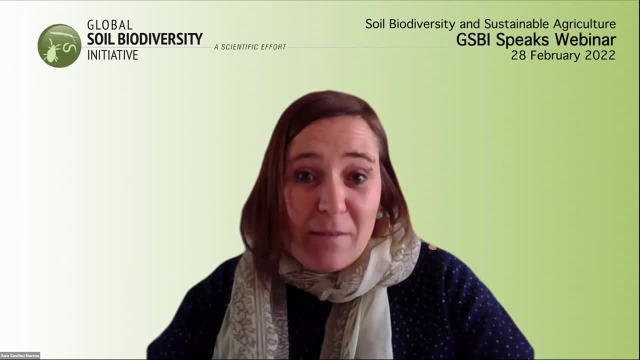 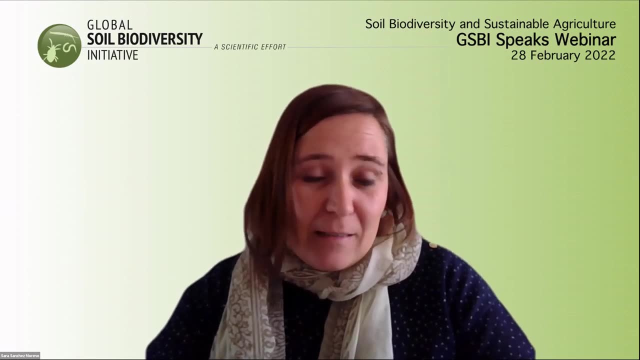 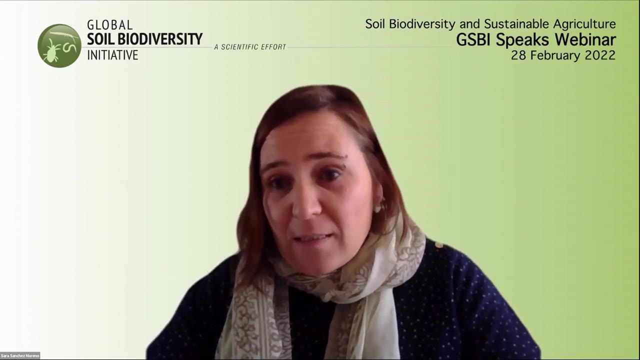 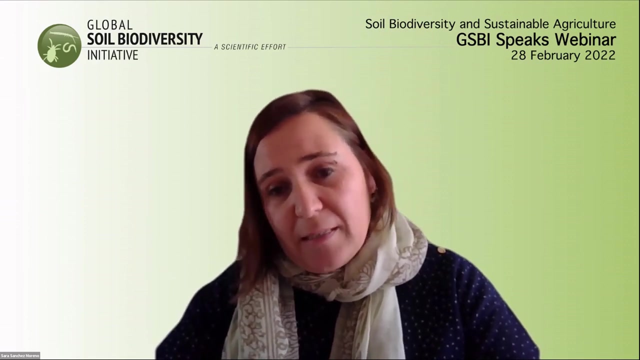 while most soil animals are actually beneficial organisms. So, except pests and DC and vectors of soil diseases, I would say all soil organisms should be promoted in all agricultural systems. Doesn't matter if they are rain fed or irrigated systems. The thing in irrigated systems: 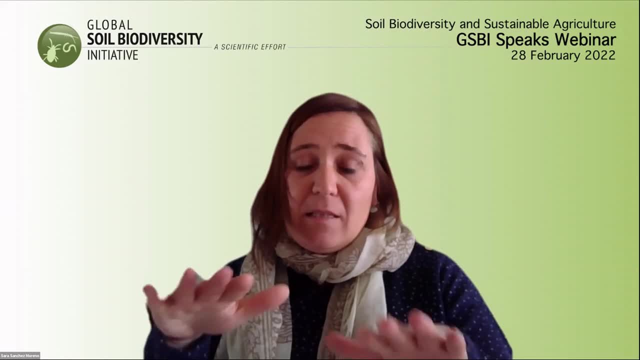 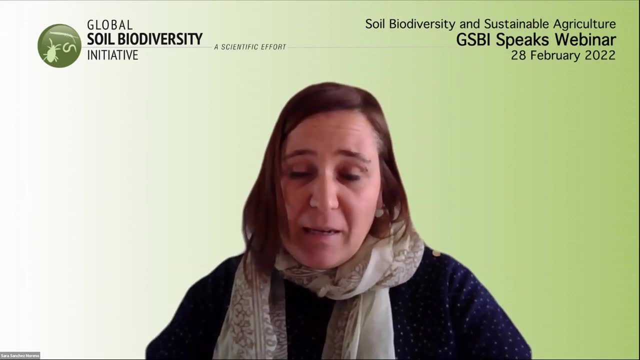 depending on the irrigation is that the distribution of soil organisms can be very, very, very patchy, because can be very, very shaped by the irrigation type. So but that is basically it. I would say all, all of them, Yeah. 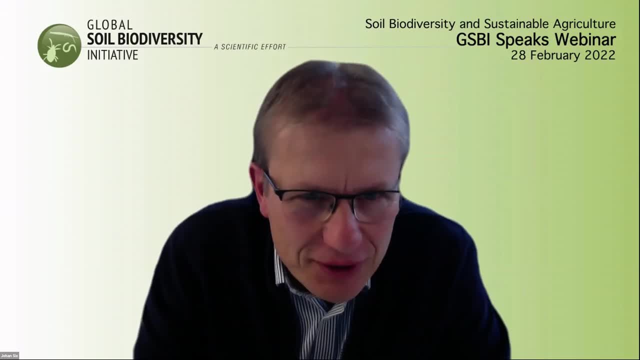 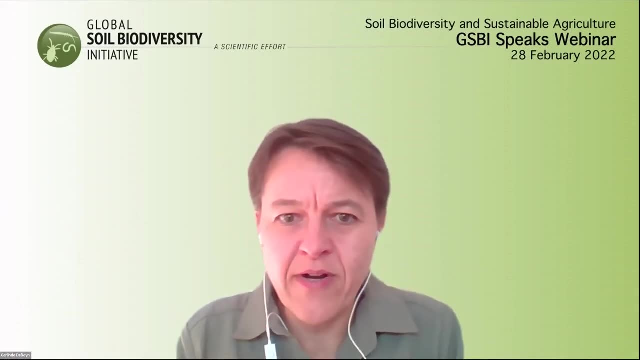 Thank you, Helene. you seem to want to say something, Yeah, yeah, Is it really just irrigation, or irrigation together with some mulching or organic matter management, Because you still need to provide some food, right? So the idea, then, that the food all comes from? 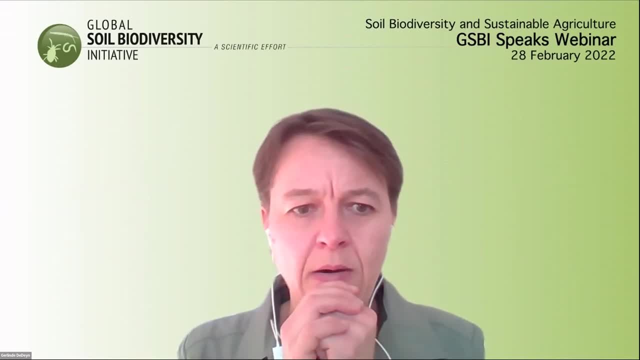 from the crop itself and the turnover of roots. or, I just wonder, irrigation, is that just water or does it also mean mineral nutrients and and skipping the whole organic matter that contains nutrients? I I think it's important to have that organic matter with kind of slow release. 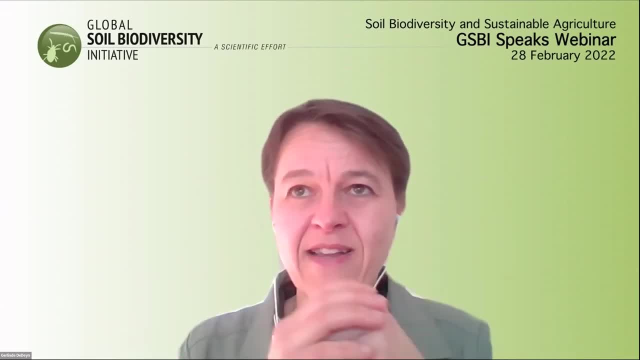 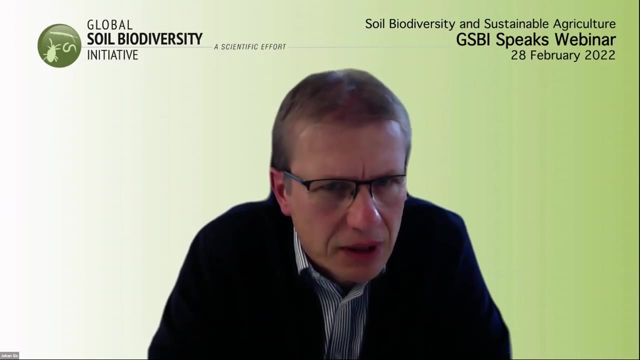 nutrients and being inhabited and and and attracting, like these ecosystem engineers, that that water is a nice start, but I, I think you need more than just water, Yeah, So there's a question also that I mean. so now, until now, we have been mostly talking about how the 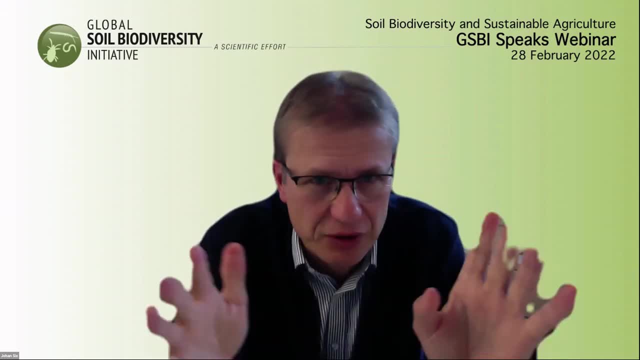 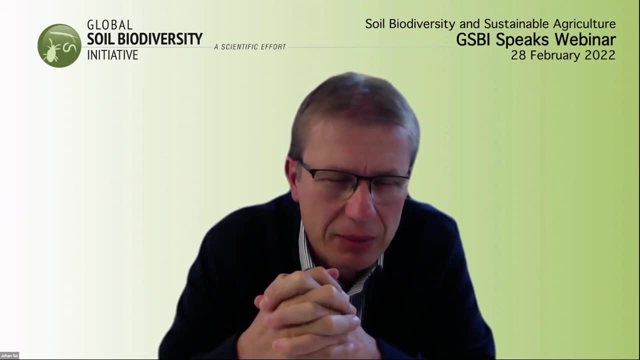 you know how management or whatever is affecting specific groups. but there's a question from the audience also on how much of do we have interactions and specifically about how the soil microphone, how do they affect actually the soil microbe, my volume? 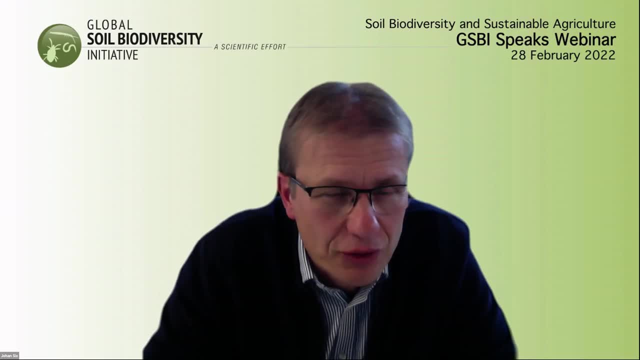 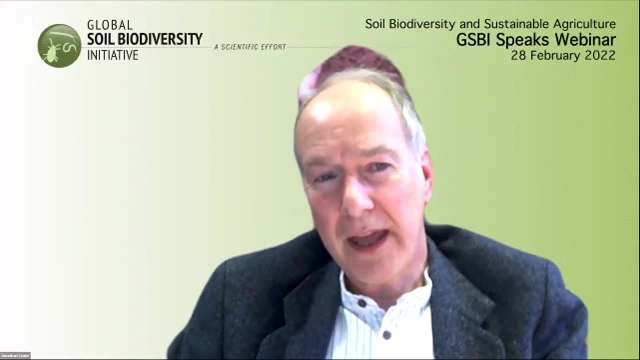 and also the phytobiome. Any thoughts on on that There have been. I've not done them, but there have been studies that have looked at these sorts of interactions And it is clear that there are interactions between, for example, 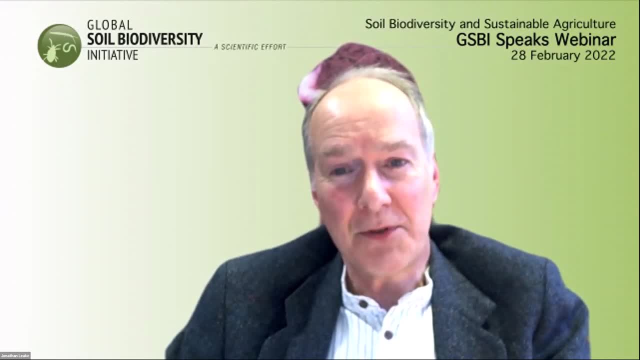 earthworms and mycorrhizal fungi, and they're not always as negative as you might expect. You might imagine that earthworms, by chewing their way through the soil, would break up mycorrhizal networks, But I think there's a kind of 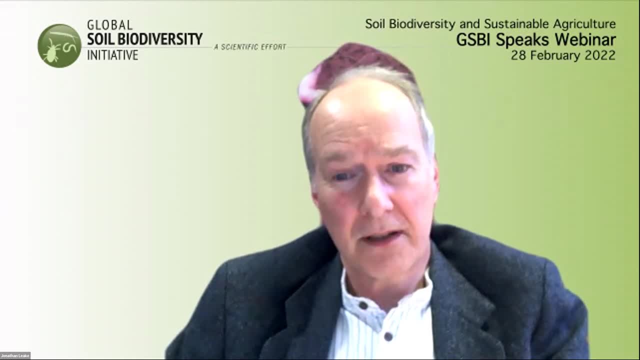 but I think there's a kind of synergy between them, that that they tend to operate, as I say, synergistically. So, yeah, I mean, I think some of the some of the bigger, more disturbing soil animals may, burrowing animals and soil may actually cause adverse effects on some of the 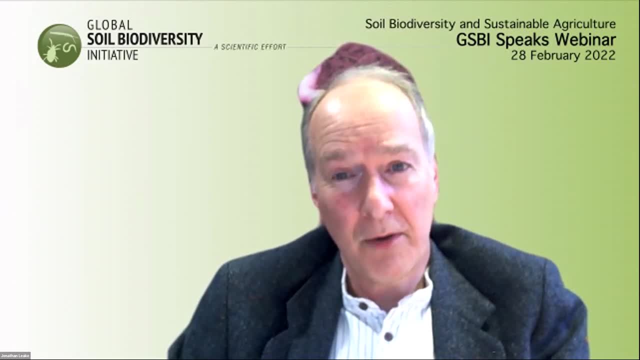 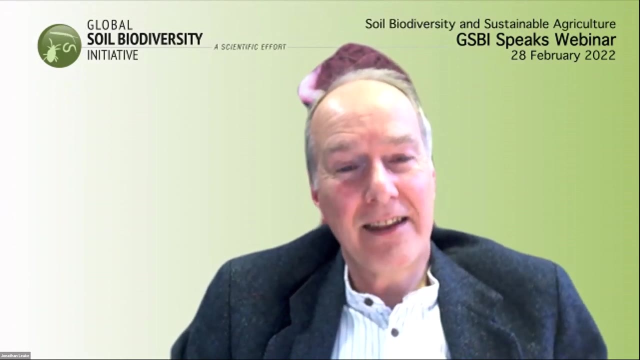 fungal structures and and larger microbial communities and and networks and so on. But but actually I think in in well balanced soils with a good diversity, these things tend to be compensated by better growth of the organisms anyway, And and the improved porosity is. 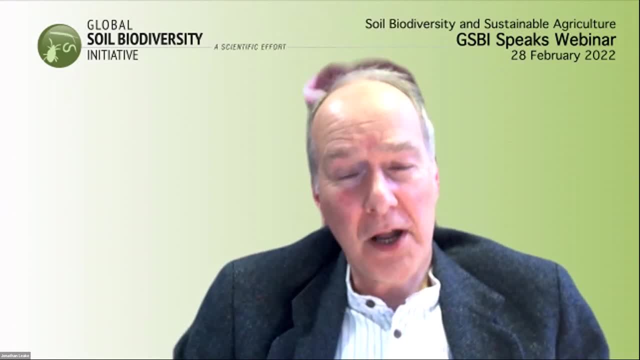 is often one of the key things, because I think we've often overlooked the importance of the relationship between soil structure and soil biology and the extent to which soil biology plays a very important role in generating both aggregation and also pore spaces- And, I think, a really critical issue for 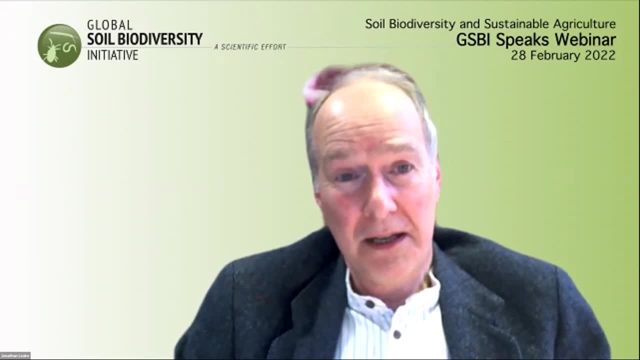 for maintaining healthy soils is that balance between parts of the soil which have been physically protected and parts of the soil into which gases and water can move in and out very, very quickly, And that that provides a really good functionality. Yeah, 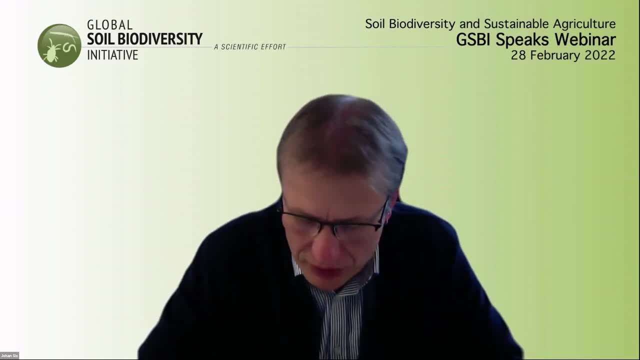 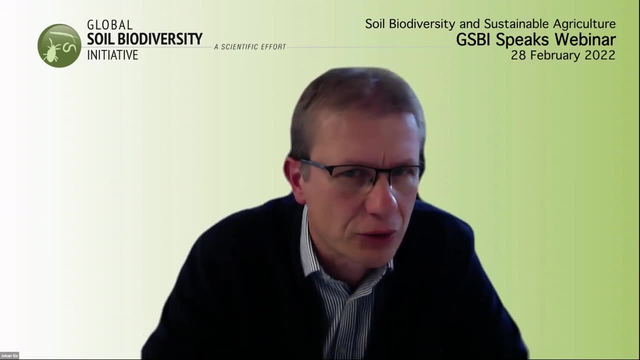 So, Jonathan, since you're onto the earthworms, there's actually some questions also from the audience about your, your systems And and there's a question about if there are also invasive or non-native earthworms that were present in those. 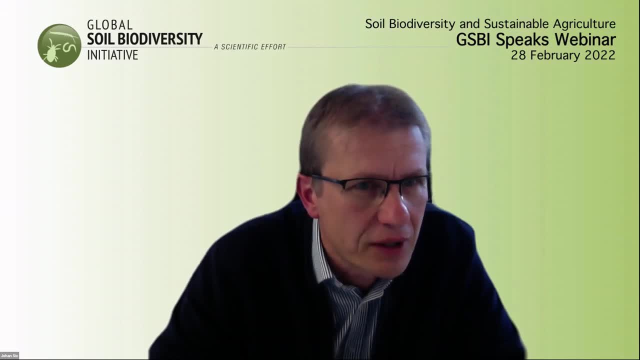 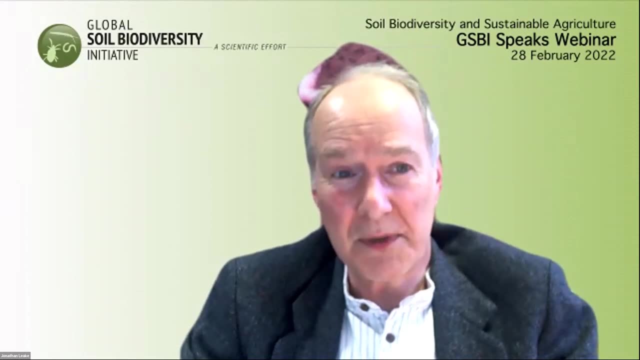 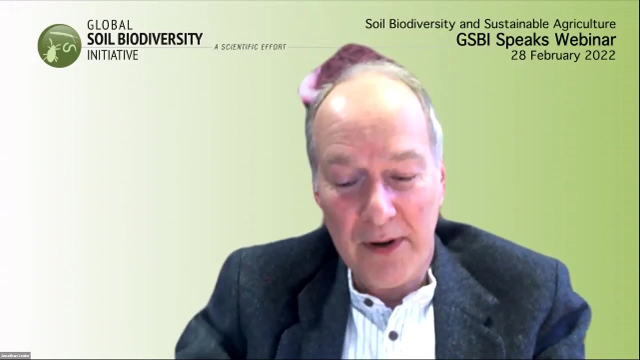 in those lakes, or was it mostly native? They're all native because we we don't have there, in those field systems, we didn't have any invasive species. So they're all, they're all native. What's interesting is- and I didn't really explain fully- 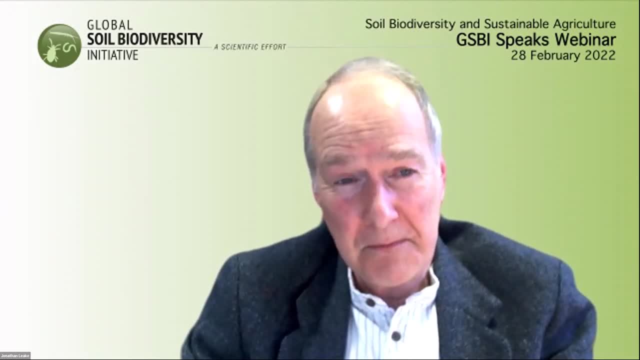 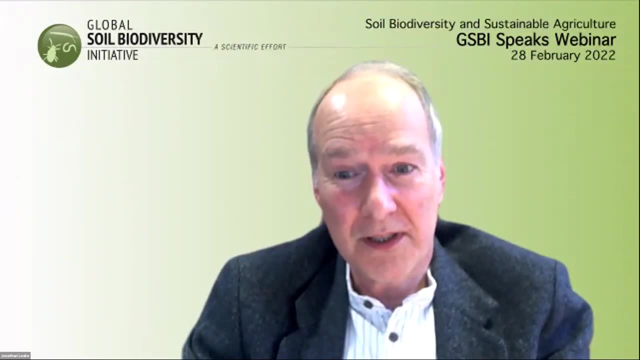 the reason why we had pairs of lay strips was that out of each pair, one of the one of the lay strips was connected right up to the hedgerow. So it was continuous to the hedgerow And in the other of the pair, 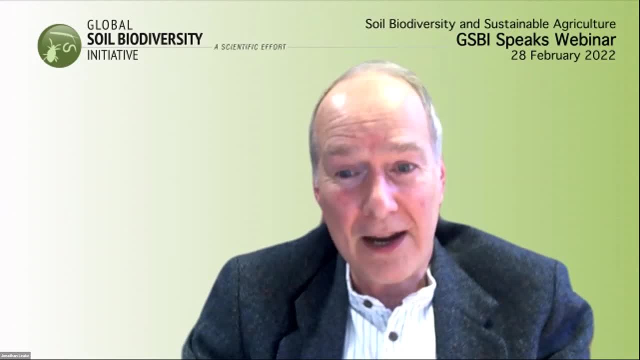 we had a barrier- It was a stainless steel mesh barrier like a curtain- that we that we ran into the soil And we had a fallow zone inside that, between the end of the, the lay strip and and the field margin. 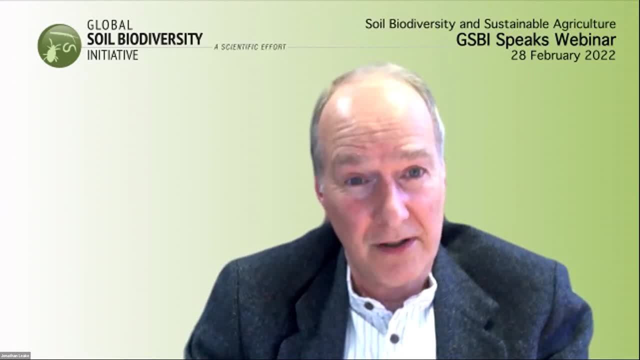 And the idea was to see if we could prevent migration from the margin back into the field. Well, we we saw no effect at all at the barriers And we don't think that the barriers were, that the barriers were being evaded. 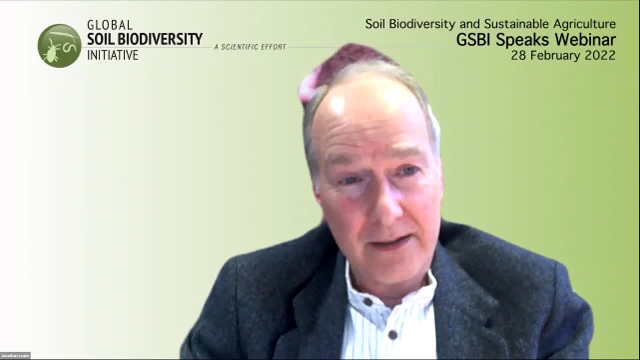 They were very long actually, relative to the width of the strip. So so sorry it's a long, long answer, but the reason why I'm saying all this is that what we think was going on in those fields was was we were re-recruiting from the depleted populations that were already. 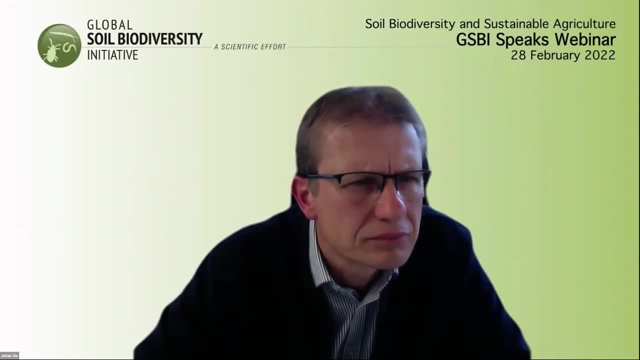 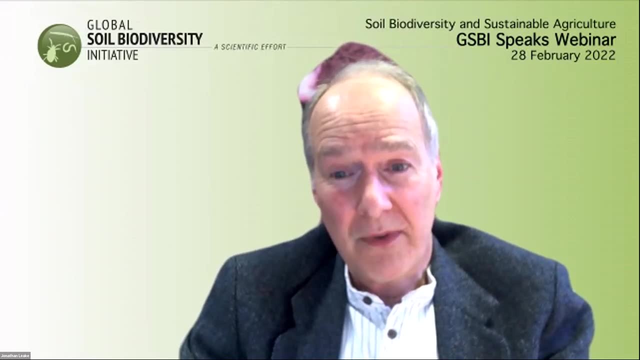 there, So so. so there were small numbers of earthworms- They were still there- of of a variety of species. They didn't migrate in from the edge, but they recovered from within the field, which which, in some ways, was encouraging. 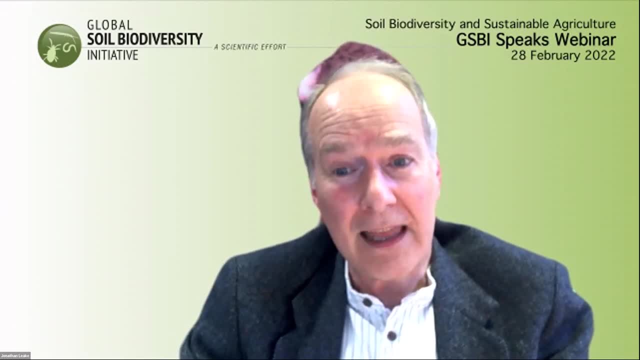 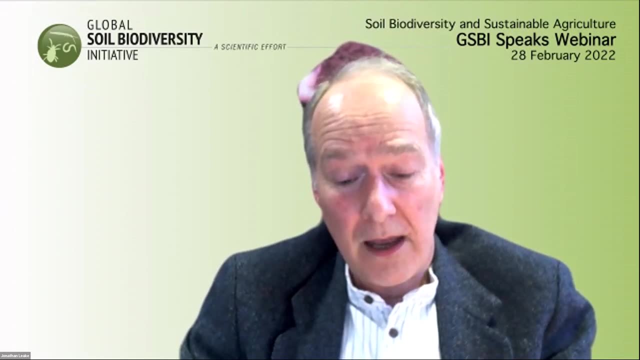 And we think the same was true with the mycorrhizal fungi, Because, again, there was no evidence that they'd come in from the edge, Although it does have to be said that we did see some species of mycorrhizal. 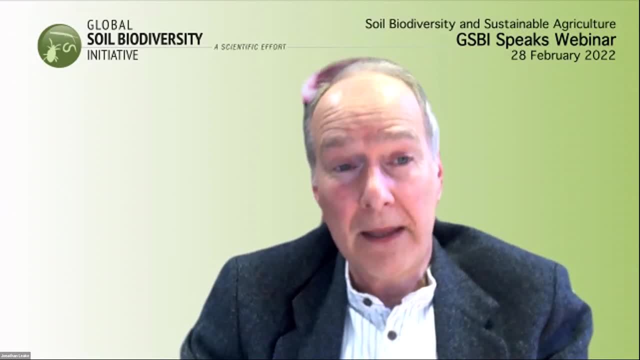 fungi that are associated with the hedge starting to appear in the lays, but they were. they appeared independently of distance from the hedge and they appeared independently of the barriers that we, that we'd inserted in the fallows, that we fallow zones we'd inserted. 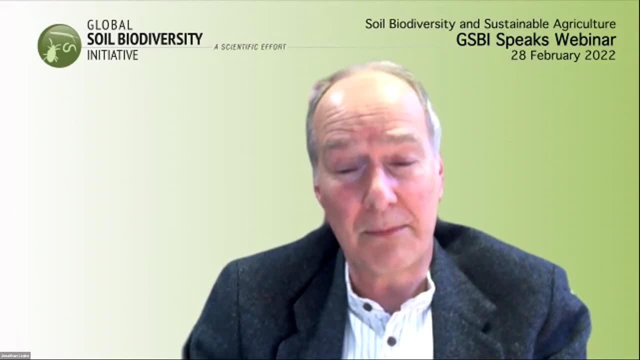 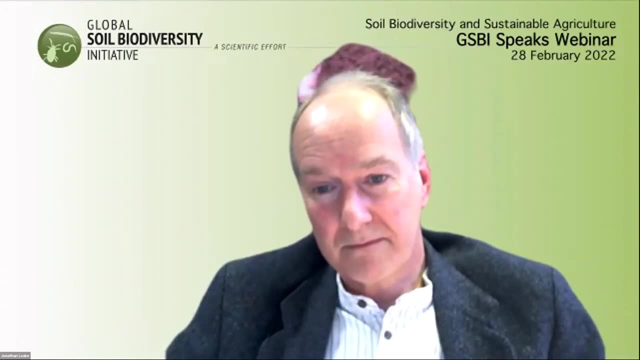 So we think they probably also were recruited from within the field, from from very depleted populations. So so there's some people also that are interested actually on how do you effectively incorporate these lays into your crop rotation, Like what kind of duration do you want and how often? 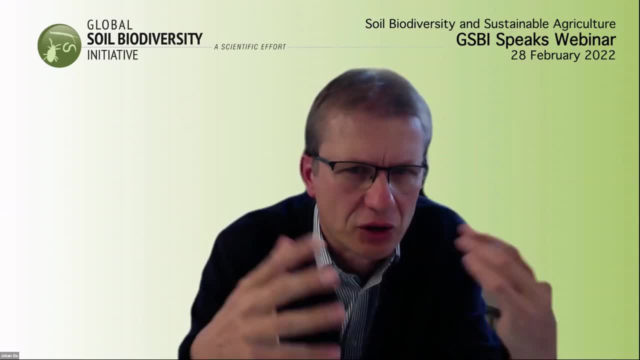 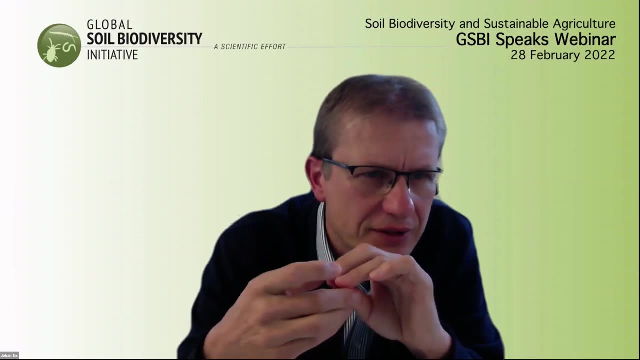 you know how long is the legacy effect of these lays, And so, yeah, what would be somewhere an ideal rotation with these lays is what people are asking, Yeah, So. so this is sort of how I mean this is a bit more of a tribal question. 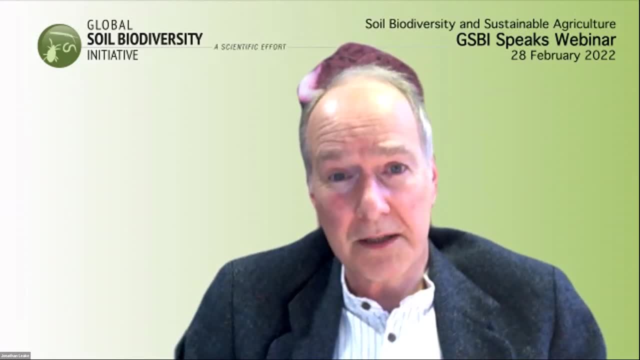 So I think for a lot of why I was, I think, standing in the field for about 20 months talking to my colleagues. I think there's also a there's there's a lot of information, But the the thing that is really interesting, in my opinion, is that the 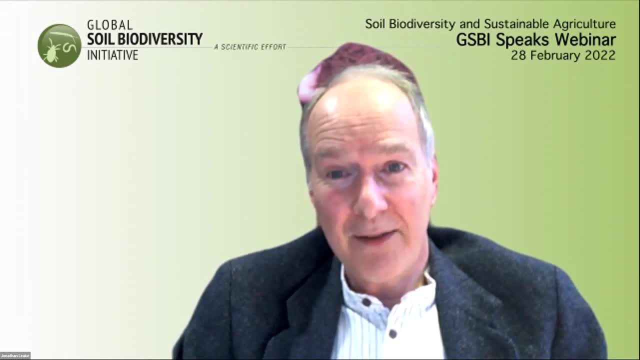 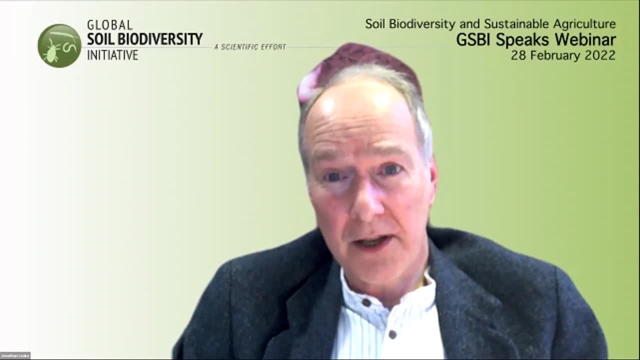 clover. but we're looking at much more biodiverse herbal lays with specifically selected deep-rooted species, species that are anti-helminthic, so they're good for the livestock. species with a high tannin content, so they've reduced the methane emissions from the livestock and they also reduce the nitrous oxide emissions from urine inputs from the livestock, and so this then changes the system quite significantly, because you then end up with much more carbon going in bigger root systems and in those cases you might get away with a two-year lay because they are supercharging the. 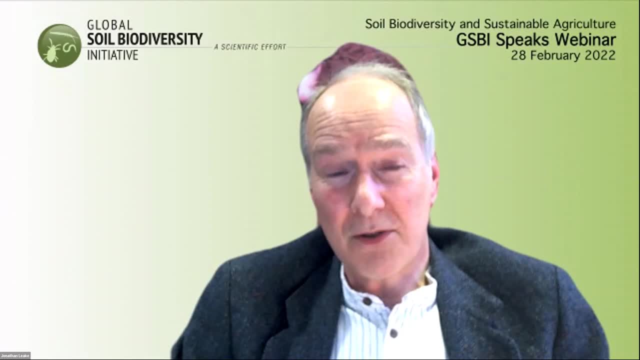 soil actually um, but i think again it depends on your starting point and and some of the farms we were working on they've got problems with black grass, which is herbicide resistant, and actually running the lay for three year years plays a major role in depleting the black grass population. so you get those additional. 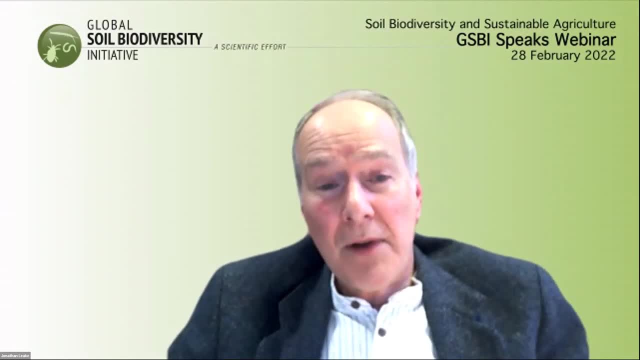 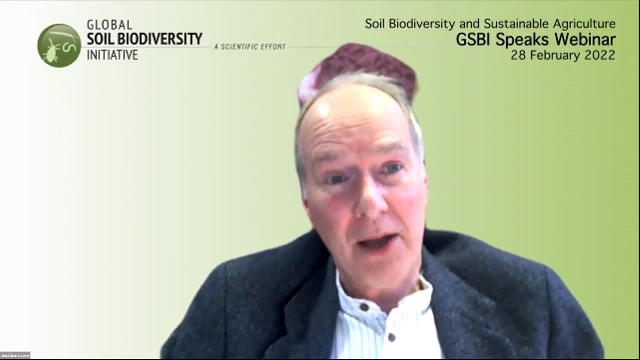 benefits alongside soil quality benefits. and you asked me about at the end how long, how long? well, we're currently trialing second year post-lay. first year post-lay: we've got fantastic wheat yields using only half the normal nitrogen fertilizer. we we were getting yields well. 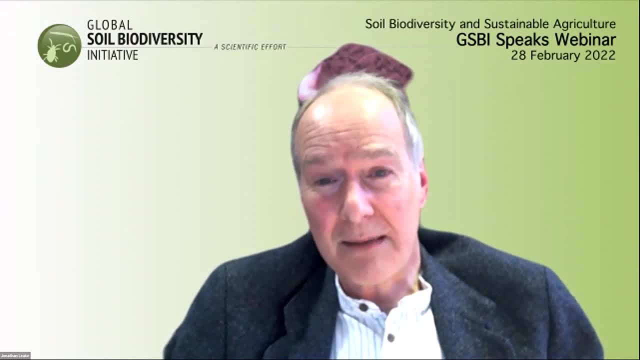 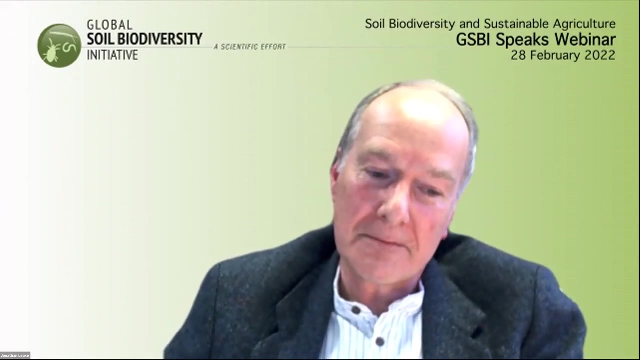 over above national average, and so just demonstrate the amount of fertility and, Stuart, you'll be glad to know. clearly, a lot of that nitrogen's gone into the organic mineral fraction and we're getting it back out again. so so, so again, it does work in practice. so, actually, for for Stuart. there was also a question about like which cover crops. 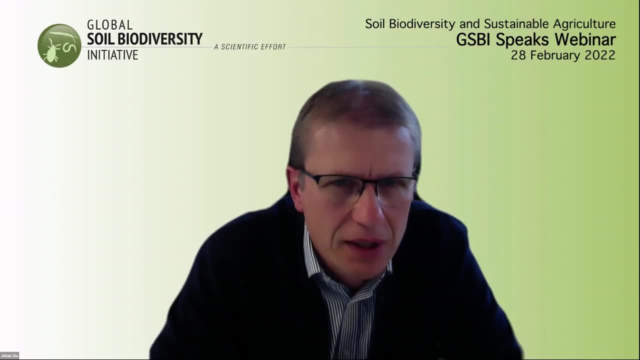 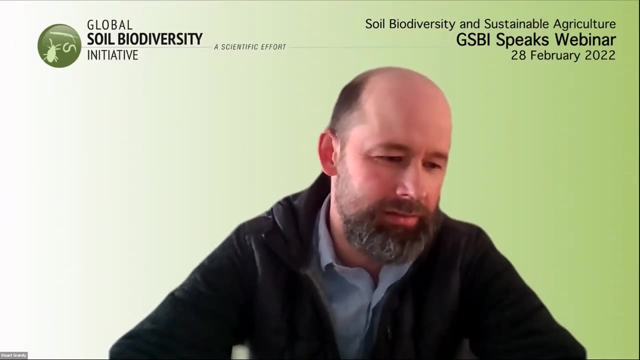 are the are the right cover crops in, in, in your rotations and, and you know to, to really build up that you know um nitrogen any, any thoughts on that? yeah, I think, when it comes to cover crops, uh, that we should not let um perfection be the enemy of the good, and we can always uh hope that we could. 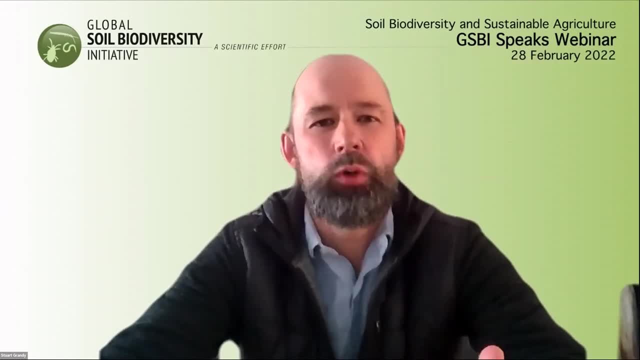 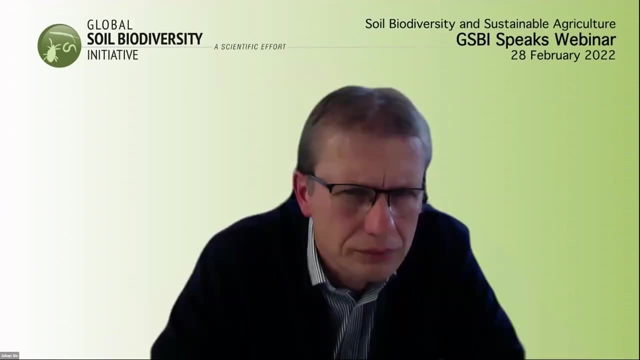 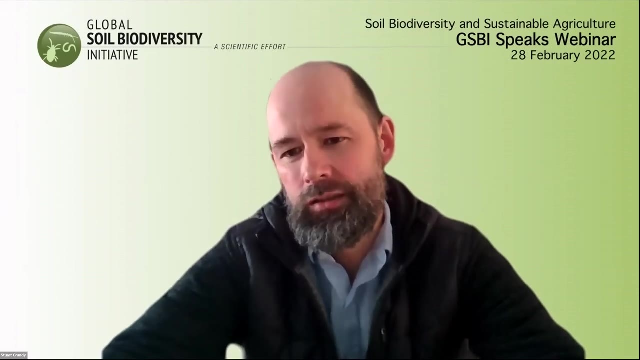 have multi-species cover crops and and increase the perenniality of our annual cropping systems. but economics dictate that that's just not often possible and we've seen over and over again that um the inclusion of any sort of cover crop is tremendously beneficial. so you have to remember. 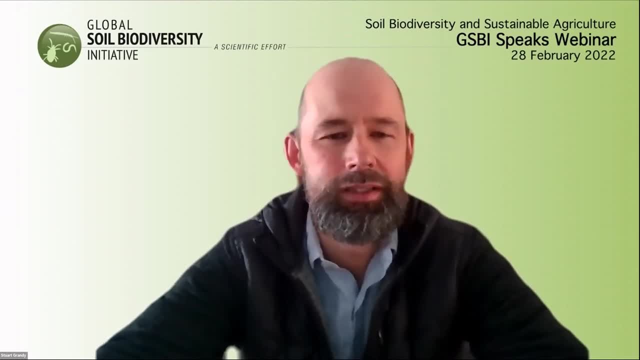 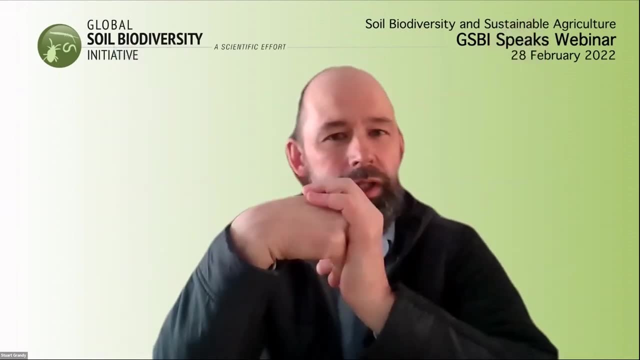 if you're growing something like rye- which is something I'm very familiar with in the types of midwestern systems and northeastern systems that I work in a lot- that oftentimes in the spring, when that's incorporated before main crop planting, it may only be like this: 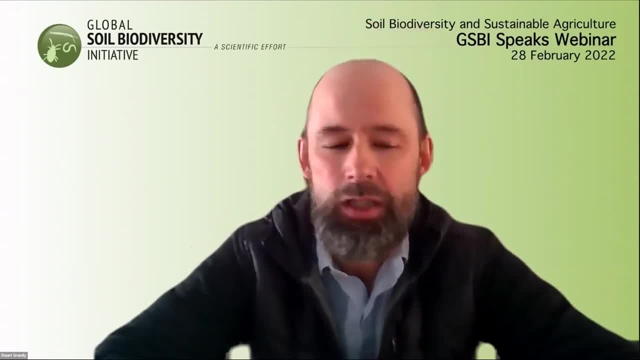 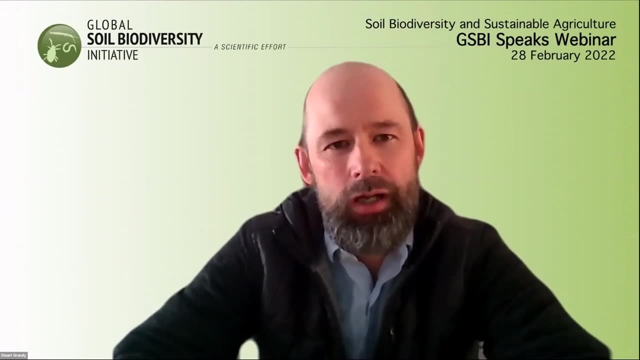 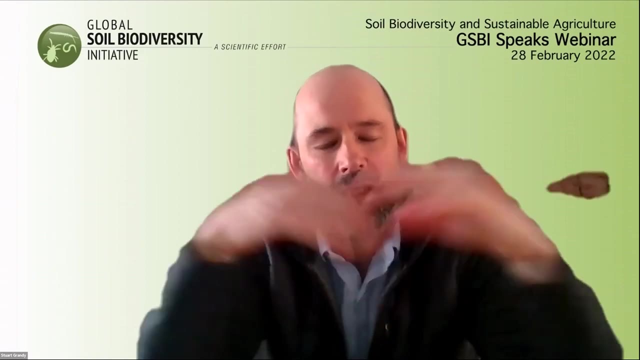 tall. right, it's very short. maybe it's this tall, but there's. those small plants are below ground pumps and they are sending far more carbon below ground than is suggested by that teeny amount of above ground growth. and we've seen this using isotopic labeling and tracking. 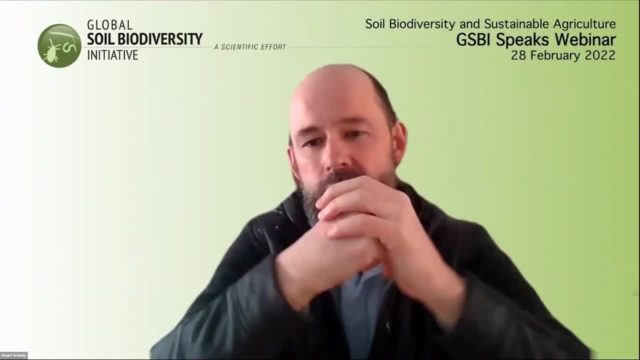 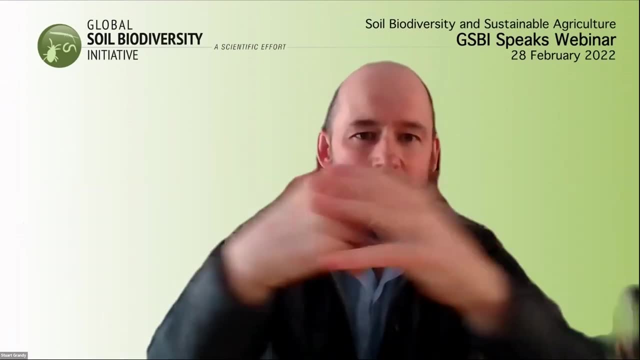 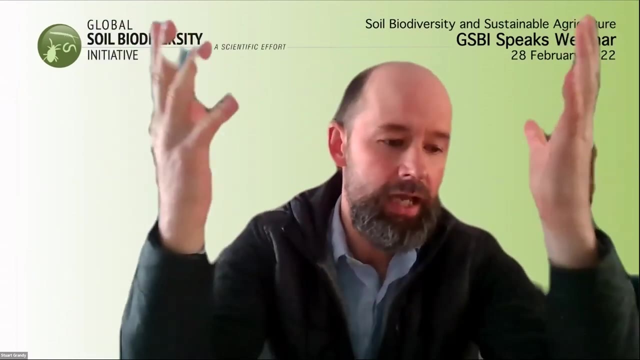 uh, new co, newly fixed co2 below ground, that um, twice as much. um, uh well, as much root biomass is produced, there may be just as much in terms of exudates that are produced, and so I would just say anything that you can do to get a cover on your soil. 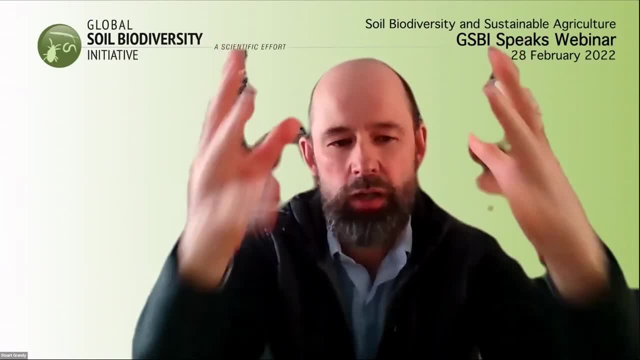 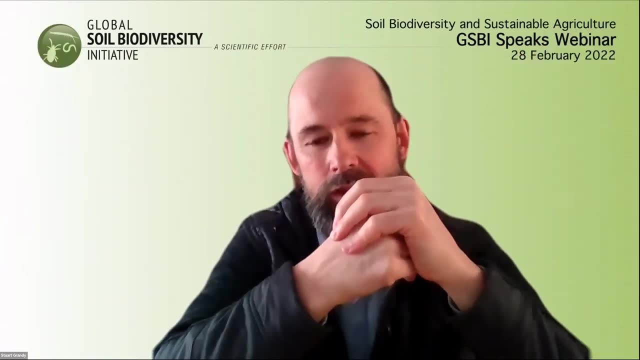 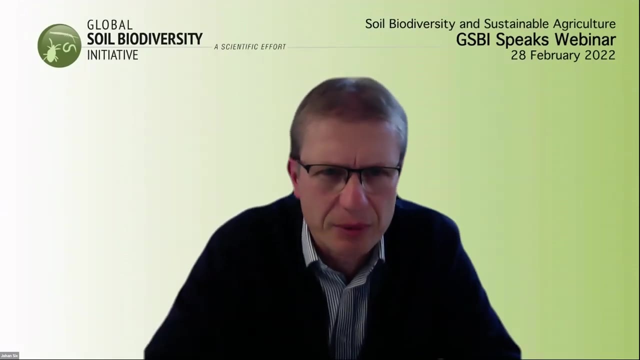 at every time of the year. a growing plant that's pumping carbon below ground is going to make the microbes and the entire soil food web much happier than they would be without those plants growing there. so there's actually also a question about you know. so you've been talking mostly about a 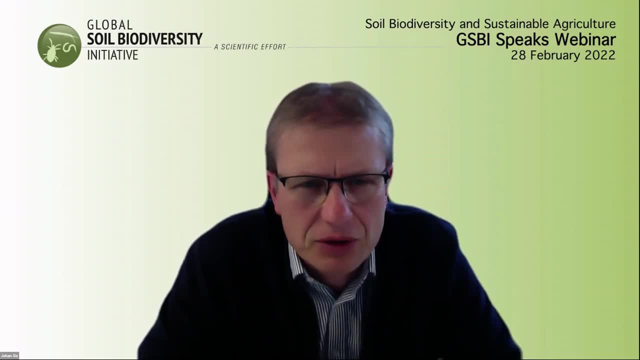 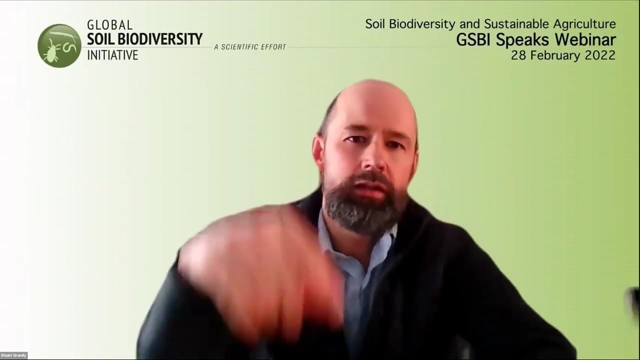 poly and rotation. but what about poly cultures, you know, would they have the same effect? so so you know inter cropping, or or whatever. so do you expect the same as as with these rotations? yeah, I just want to also make one comment, that even those crops that are not fixing nitrogen. so take a grass. 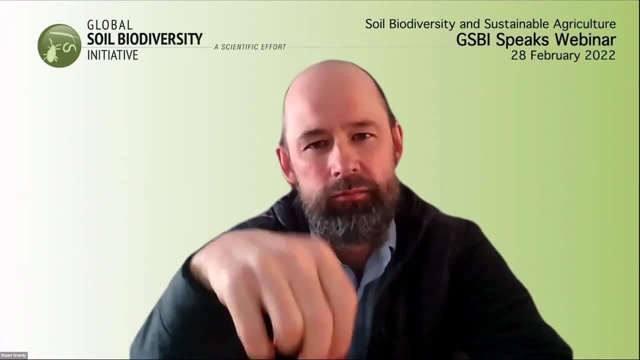 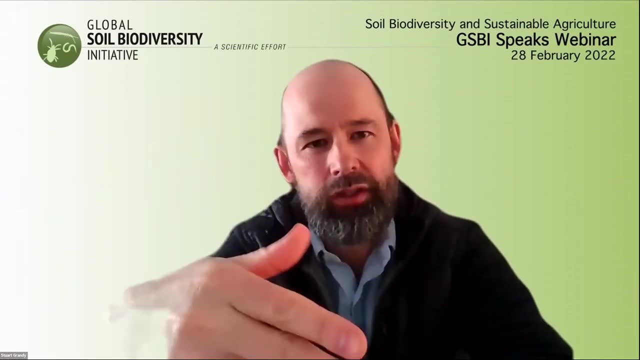 they are mopping up nitrogen that is otherwise vulnerable to loss and that, when we incorporate that crop residue, that cover crop residue, that's nitrogen that's being restored to the organic cycle and subsequently made available for crop production. so I'm wondering if you have any thoughts on that. 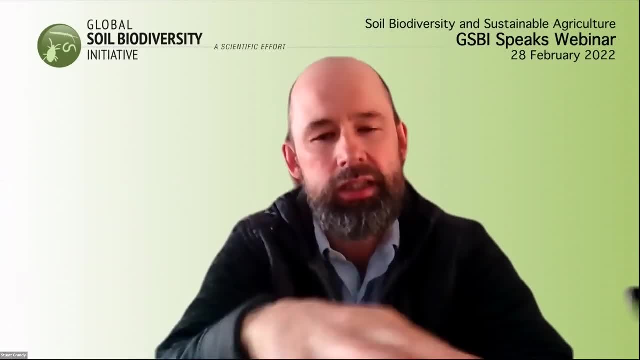 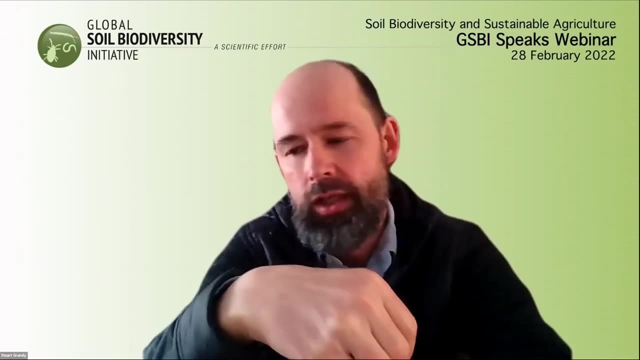 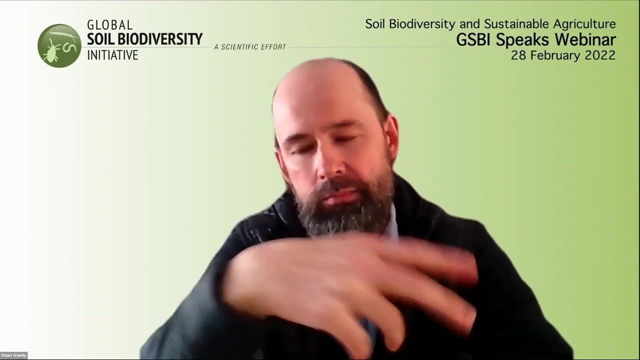 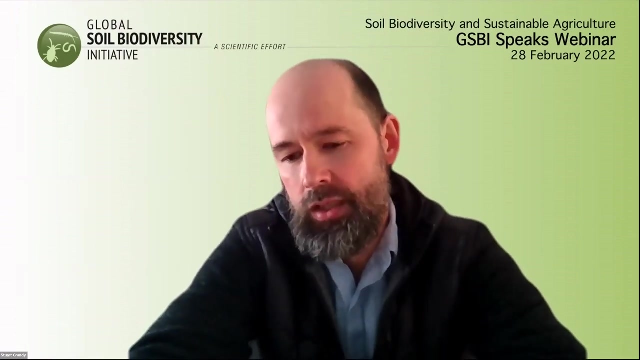 yeah, thanks, great question, thank you. so this is a very unique and complex presentation because so much of Oh phone technology has been focused on just uh, non-organic production with micro bond and pastures for soilائ and other crops are really creating, actually making use of micro bonds to make use of. but 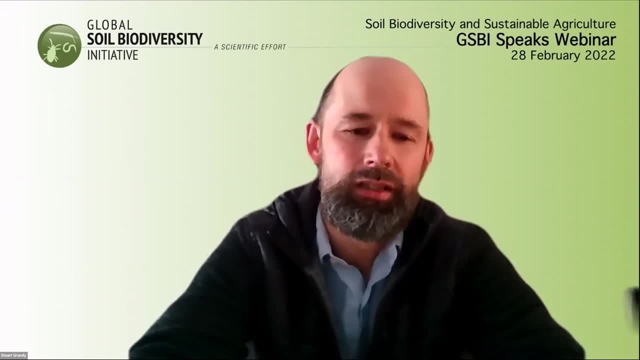 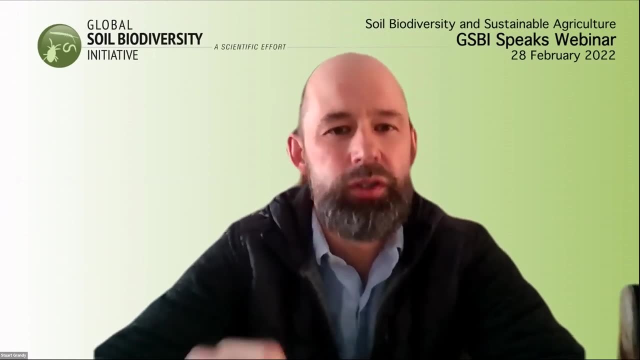 often there are alto exposure to micro bond, so there's also a lot of uh. I've been working on Okinawa smoke, 더 low ground biomass in the building of soil structure that others have talked about, associated with perennials. if that's a if that's a realistic scenario in your cropping system, go for it. 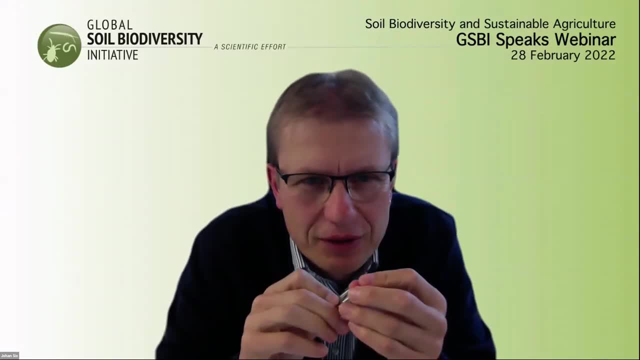 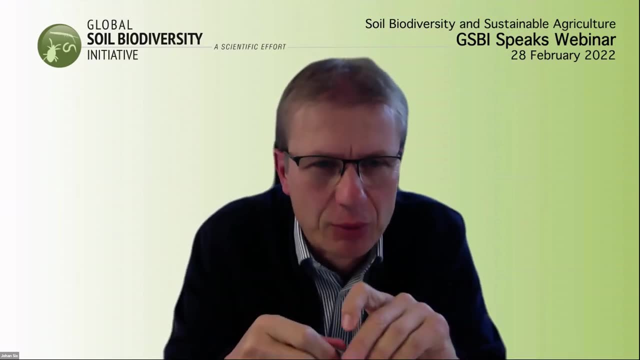 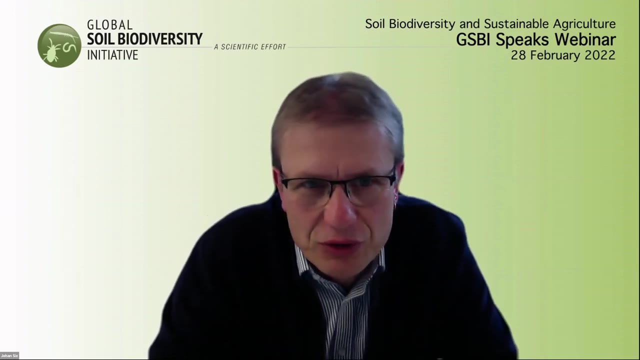 so there's also, there's also two questions, uh, or a few questions from the audience about. you know, you're talking about these, these ways of these new practices or whatever, but what is the the? you know the economics associated with that, and so, from an economic perspective, what is the most efficient way of of improving your soil biodiversity? 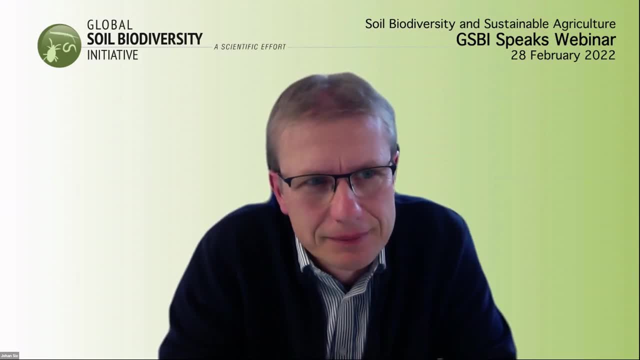 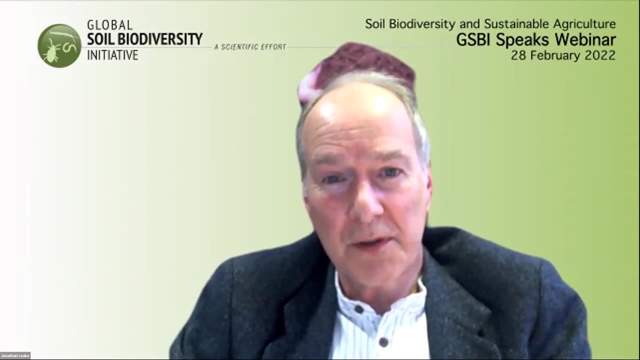 i think that depends on your economic system. so for example, in the uk, where you know the government is now providing financial support directly to improve soil quality, then some of these cropping systems with lays become financially viable in a way that they won't in a system where there is no direct support for that kind of 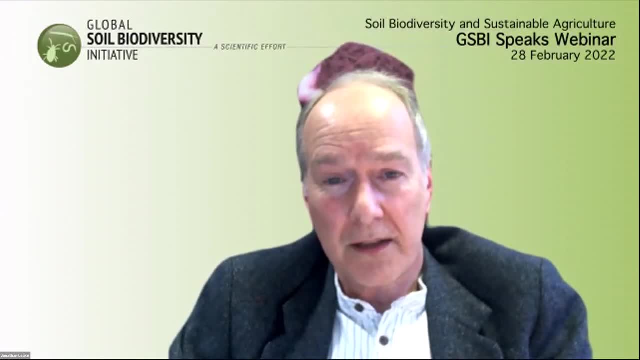 intervention, um, but i would also say that you know that there have been a number of studies now that have demonstrated, for example for livestock grazing, that the traditional model that was used in in many western european countries of growing rye grass heavily fertilized to maximize production. 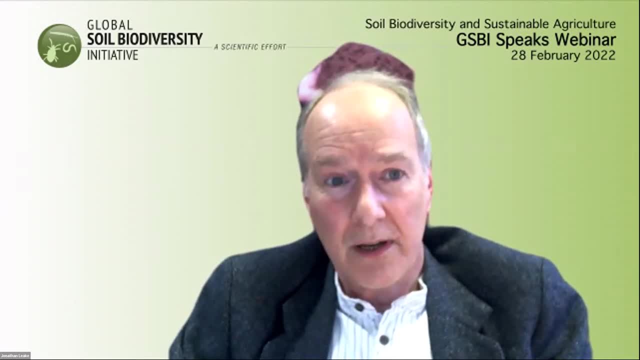 of sheep and cattle has subsequently proven to be economically far less advantageous and environmentally far more damaging than using mixed species incorporating legumes, uh, which provide better feed quality, reduce the greenhouse gas emissions and massively reduce the nitrogen fertilizer requirements. so so i think we are in a changing we're in a changing world. at the moment, the price of fertilizers, particularly 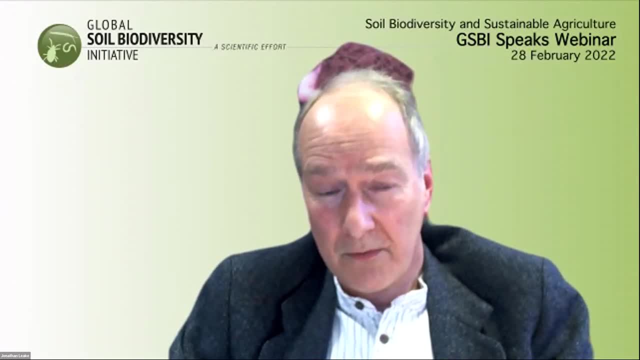 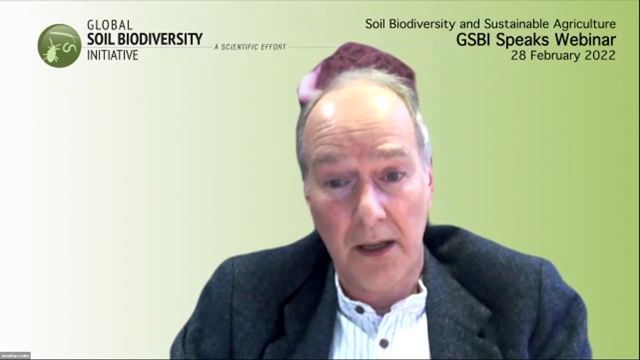 nitrogen fertilizer is also having to, causing many farmers to have to rethink high input, high output systems which have got low efficiency. um, and the one final thing i'll say is that, in relation to this, again coming back to the issue about perennials and perennial break crops, particularly in systems using reduced tillage, which, of course, saves fuel, 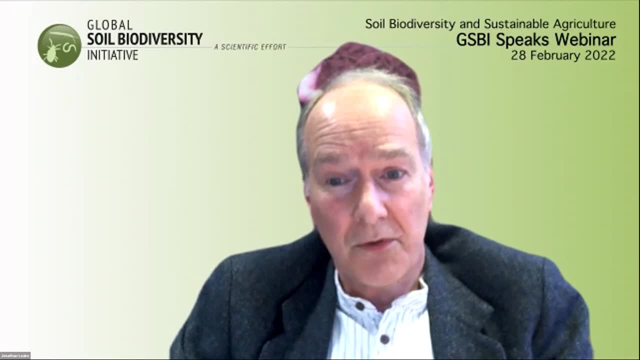 and diesel costs. um, if you're moving into a system with reduced tillage, having previously grown a really deep rooting lay, for example, it opens up the pore space deep in the soil for the root systems of the following crops to go down and gain access to nutrients much deeper in the soil than they. would ordinarily so. then you suddenly improve your nutrient use efficiency and water use efficiency of your follow-on crop, even if you use a very reduced tillage system, otherwise not not be able to deal so well with soil compaction. so having those living root systems actually doing the 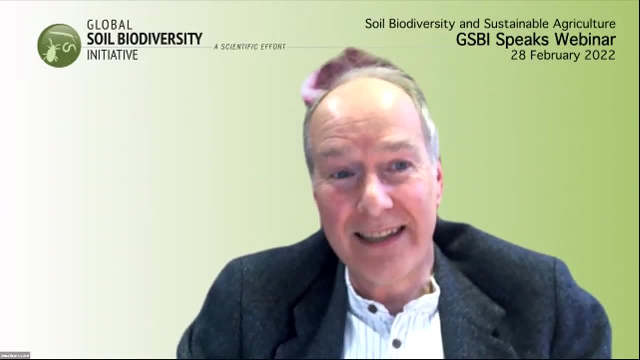 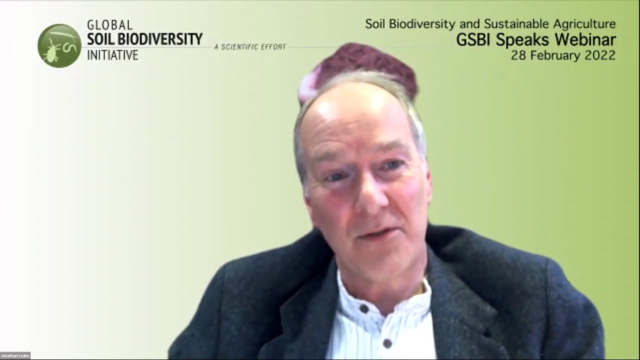 burrowing, and and taking out the steel and the diesel and using the organisms to do the hard heavy lifting for us strikes me as being one way forward that actually we perhaps need to try more widely because of the where we're, where we've been trying it, it works, and i and, and and and. the results speak for. 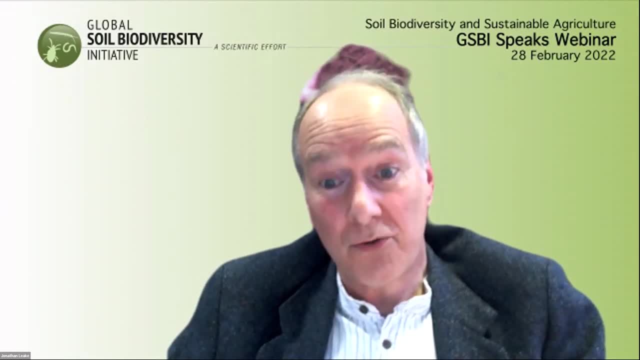 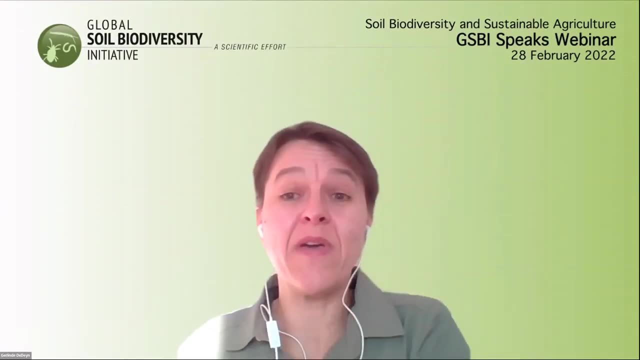 themselves in terms of fertilizer savings and and also really good crop yields as well, at least for a couple of years, thanks, so okay, yeah, i was just gonna add that- and maybe also irrigation savings- i don't know whether they irrigate a lot, but like with with drier summers and springs, i mean. 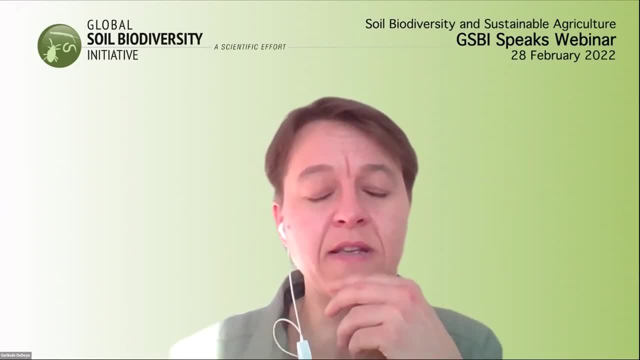 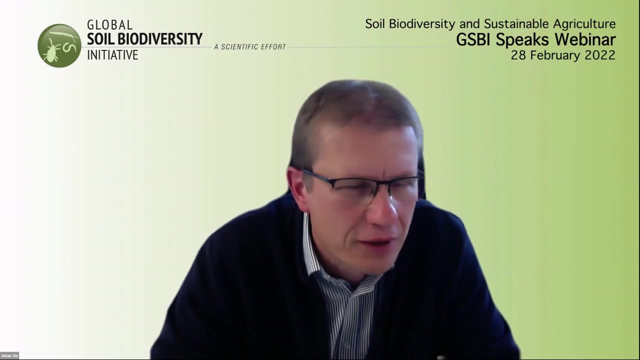 yeah, having those roots go deep enough and having the sponge activity, the buffering because of the well-developed soil, yeah, that plays into risk reduction, i think. yeah, there's also a question actually on another aspect of the economics, but then more from a research perspective there's. 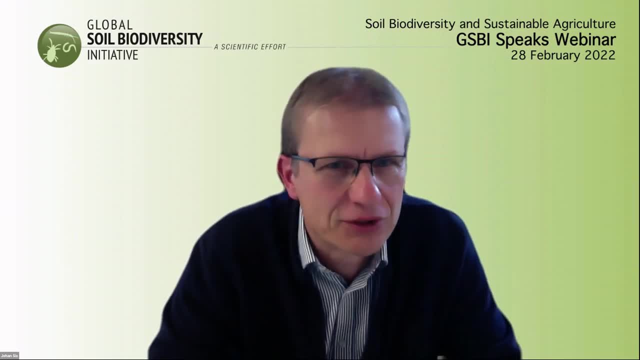 there's the indication that that you know, you guys are all having quite some funding compared to other places in the world, and and so they're asking about you know what are some of the more economic ways of of assessing, you know, the, the soil, biodiversity and and and? 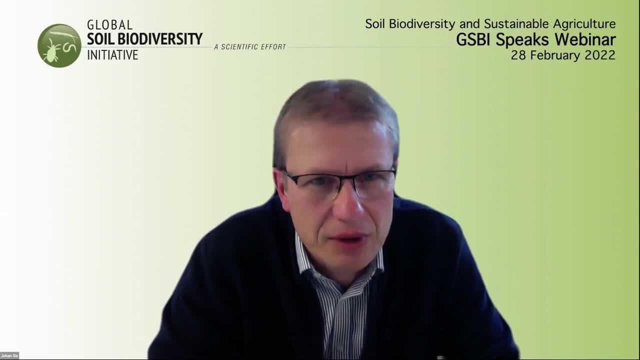 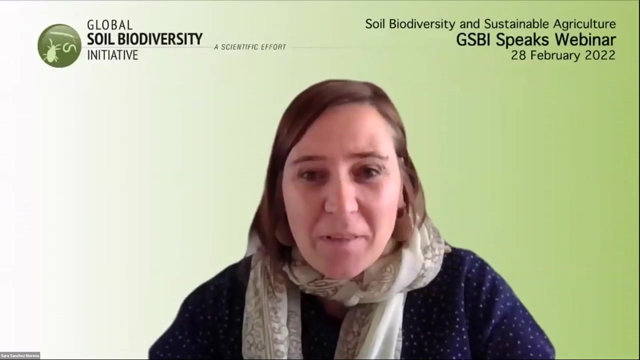 the how it's impacted by management uh in agriculture. any, any thoughts on that? what? what would be? you know, your your preferred, not so expensive methods to to do some good uh assessments? i don't think maybe you have. yes, yeah, i don't think that should be very, very, very expensive. 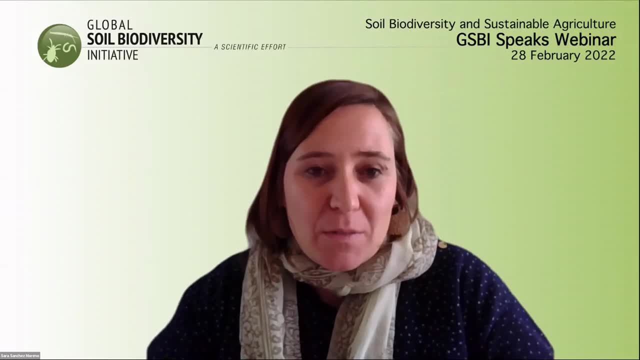 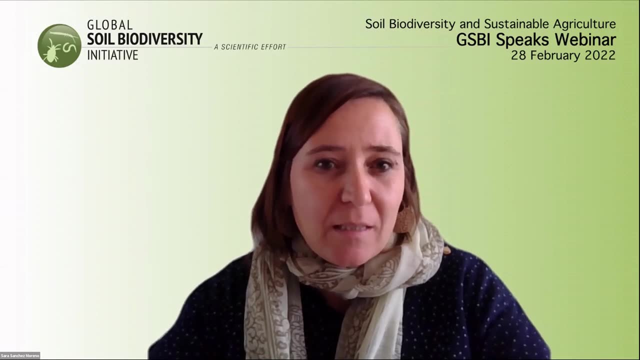 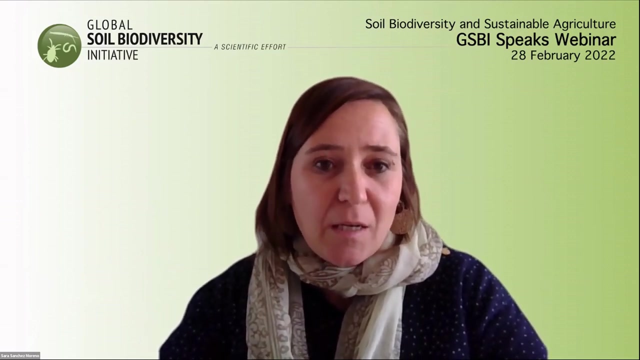 um, i mean, everything costs money, of course, but in terms of soil diversity and soil organisms and basic indicators, with basic lab equipments, many of those things can be performed without going into cool pcr or very or metagenomics or very expensive systems. for example- it comes to my mind- the tea. 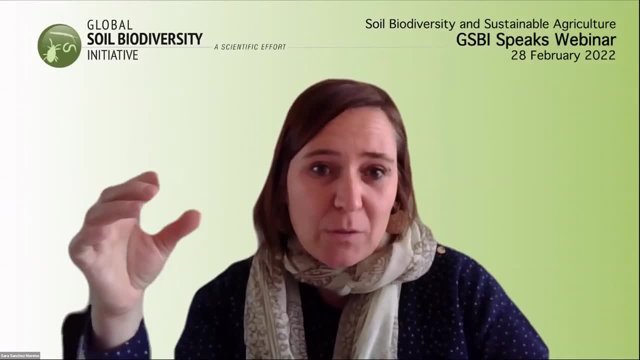 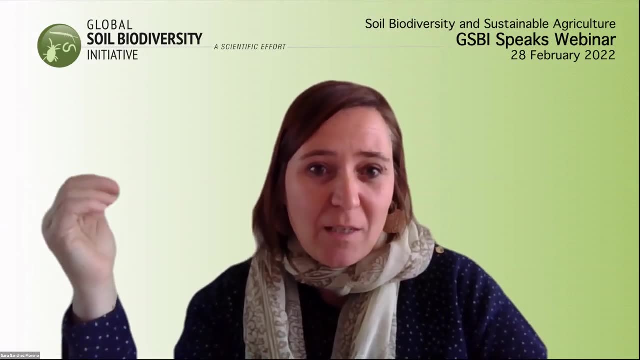 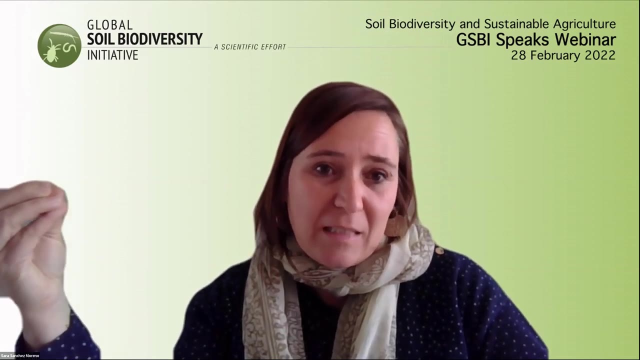 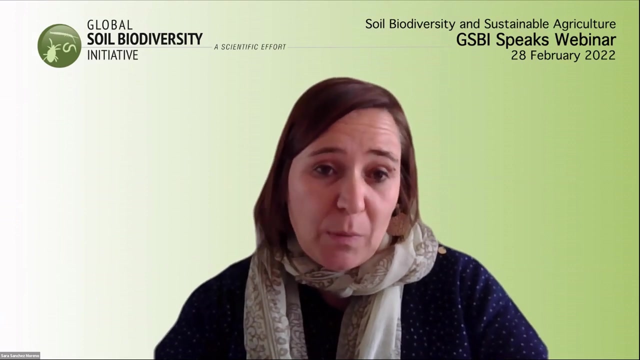 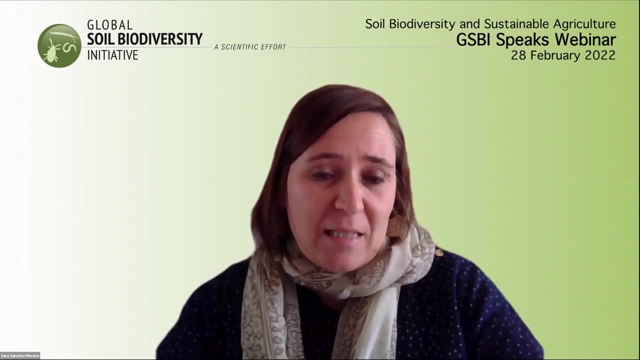 bag initiative, in which tea bags are used to measure organic matter decomposition worldwide. that is a well-established methodology to measure organic matter decomposition, which is closely linked to nutrient cycling. using only tea bags and with basic lab equipment like a very simple microscope or a binocular, many organisms- many soil organisms can be- can be assessed. 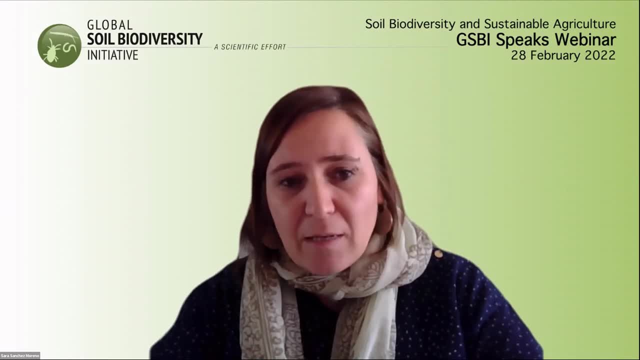 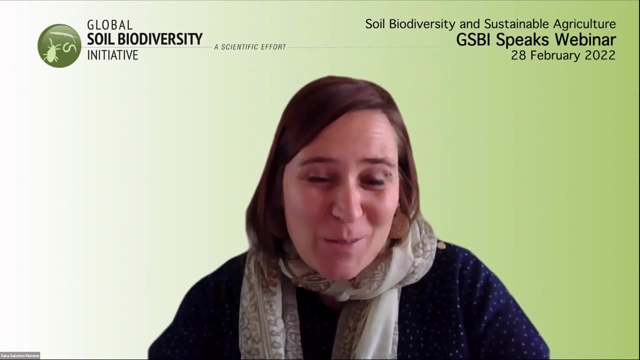 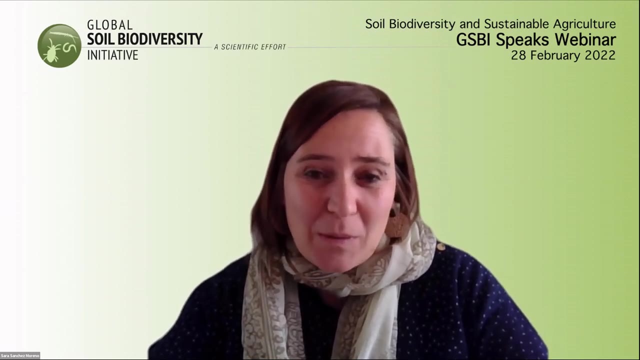 so i don't think that is that that expensive. i think you may have good quality data with basic lab equipment. i at least i am used to do it because i work with morphometrics, so i don't spend thousands of euros in molecular techniques, i just use the basic microscope. i'm sorry, while you're. 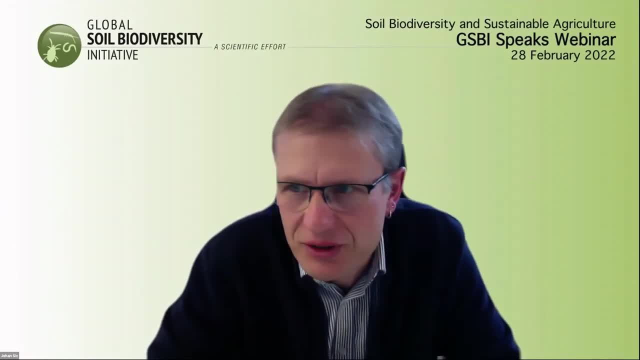 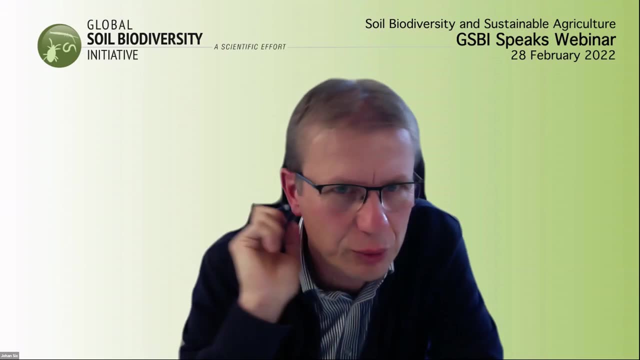 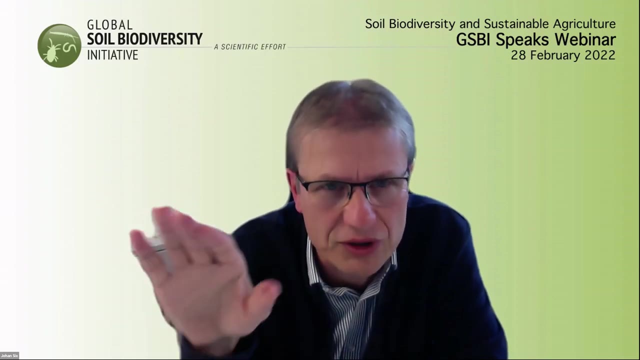 while you're talking, i i wanted to also ask another question that's in there and let's see about: um. you know, when you, when you show the relationship between the nematodes and the crop, yield that, this positive relationship, where you also- i mean, was that the whole population or was it and did it? 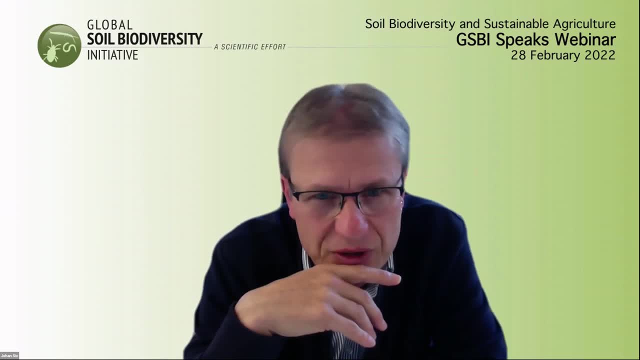 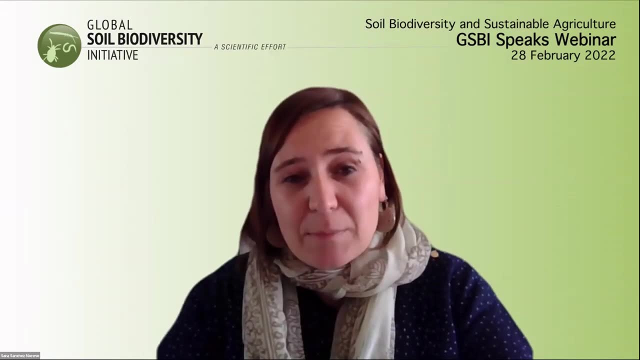 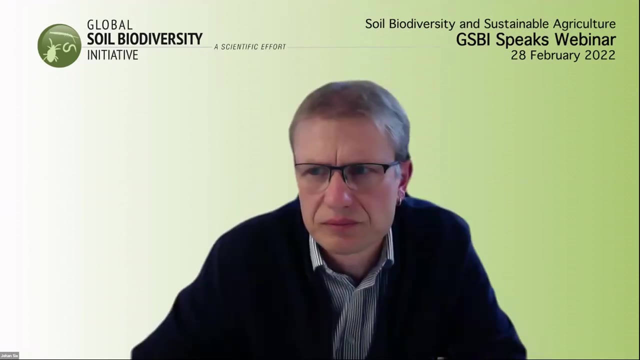 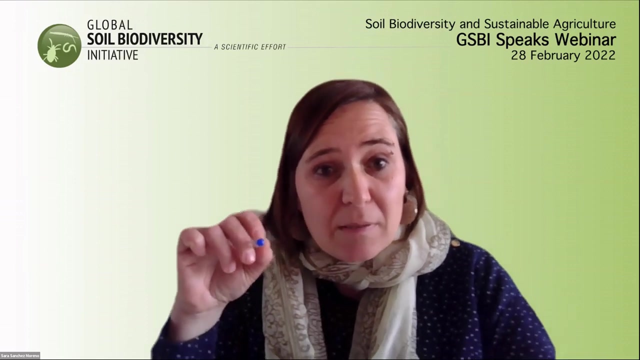 include plant feeding nematodes or was it a specific group of of nematodes that was showing that positive impact? in general, soil organisms abundance is not the best indicator because that might include very different organisms. some of those might be very different organisms beneficial. some of those might be negative. so you have to go a little deeper into the community. you. 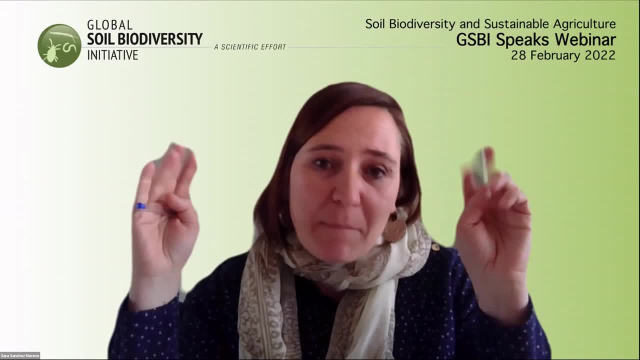 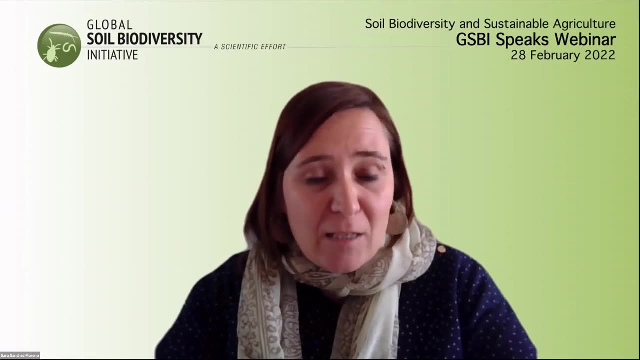 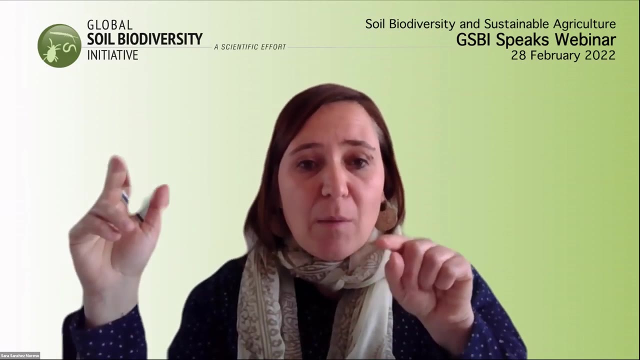 are studying and at least being able to differ between what can be seen as beneficial organisms and harmful organisms. in any case, in the case of nematodes, in general, beneficial nematodes are always positively correlated to crop yield, but we know well a specific group of soil nematodes which 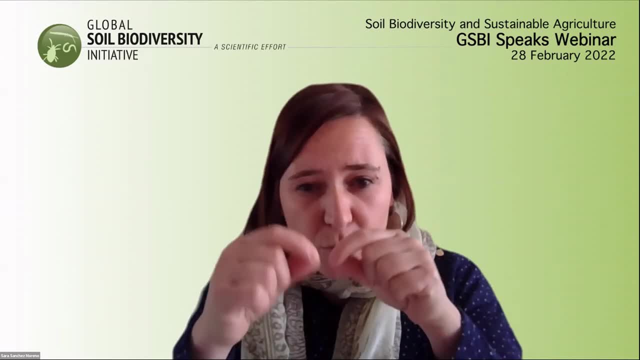 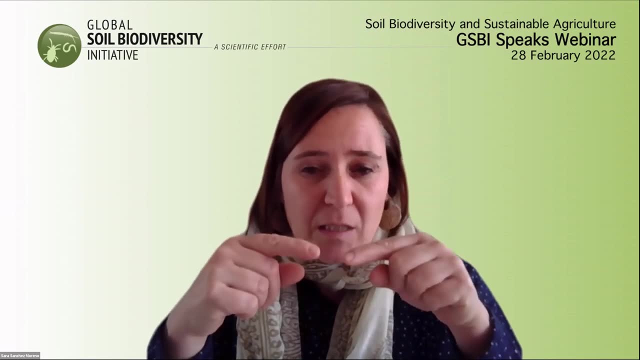 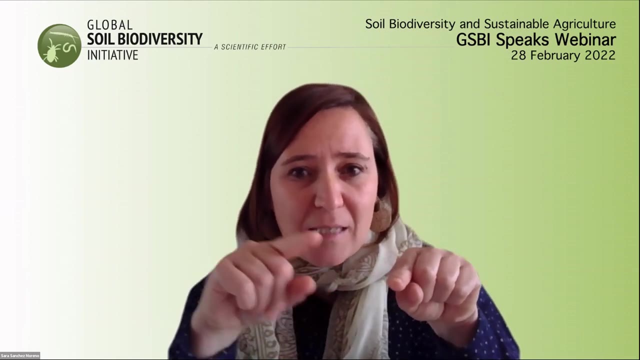 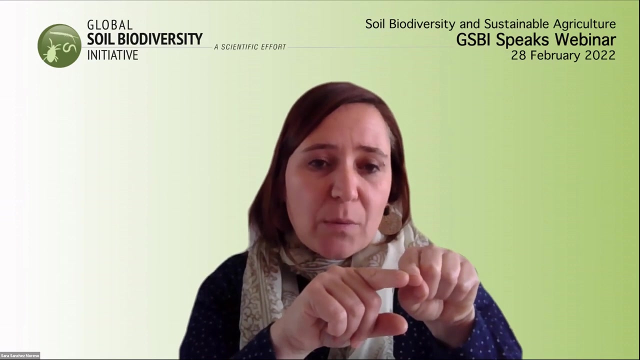 basically bacteria balls and which maintain a very close relationship with soil microbes. so by grazing on soil microbes they promote nutrient mineralization. so more nitrogen, more mineral nitrogen is available in soil and soil fertility clearly increases. so there are many studies in different countries in which we've clearly seen that the more those bacteria beneficial. 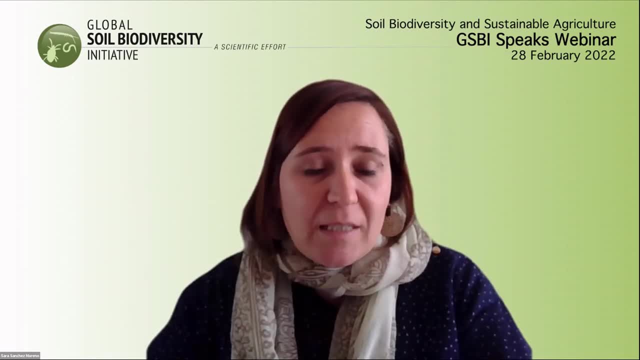 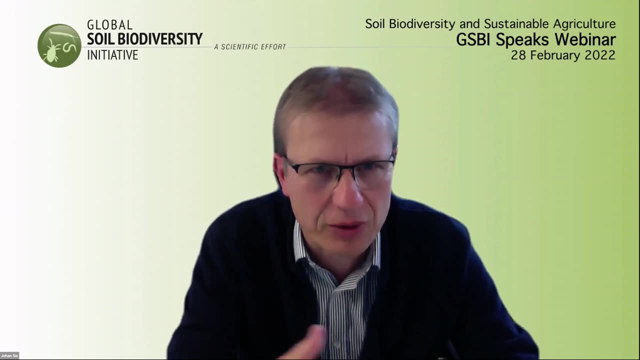 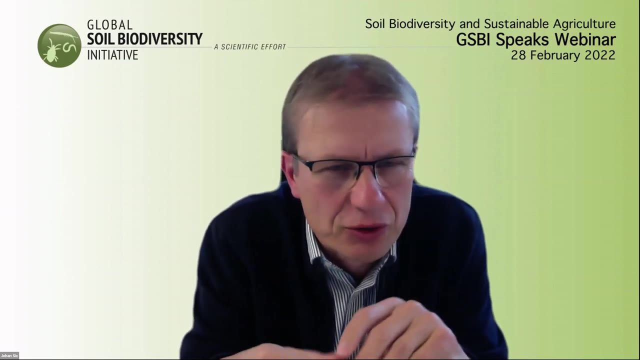 you have in your soil, the higher the crop yield is. there's also questions from the, from the audience, about you know. you've been talking quite a bit about these crop rotations. we have the lays, we have the, the, maybe the crops with deeper roots, but there's also questions about you know what? what does compost, for example, do? and and also. 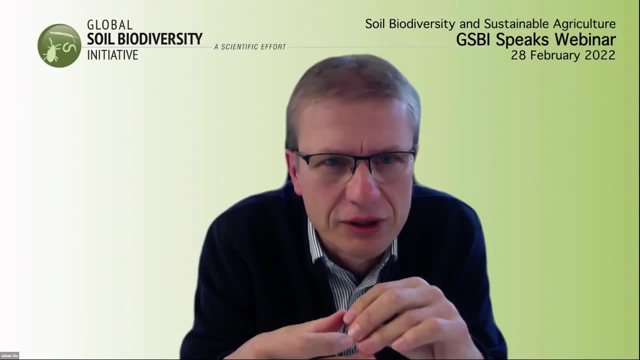 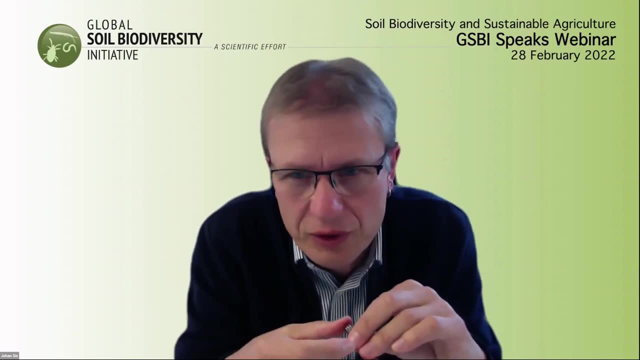 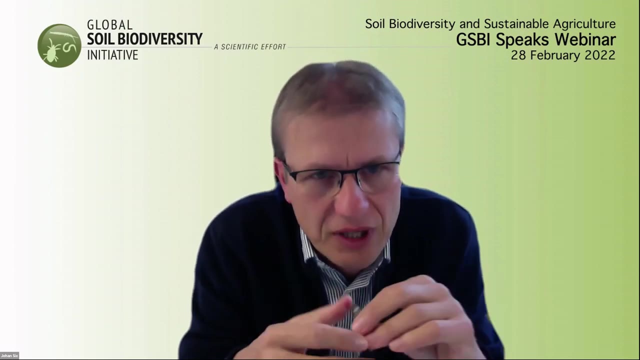 what chemical fertilizer can do, and is it only negative or are there also positive effects of of fertilizer, especially then you know when it comes to, for example, the maom, and you know can can you uh put have some of that uh being put well, stabilizing by, by chemical fertilizer or 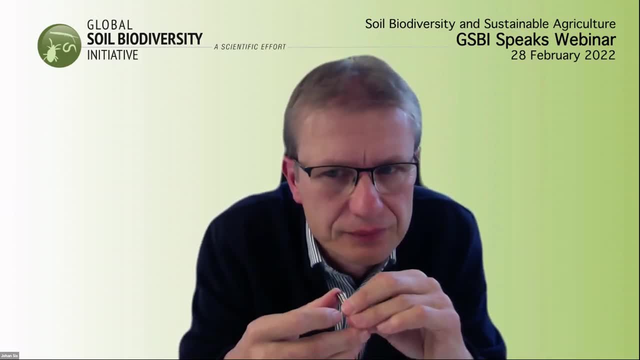 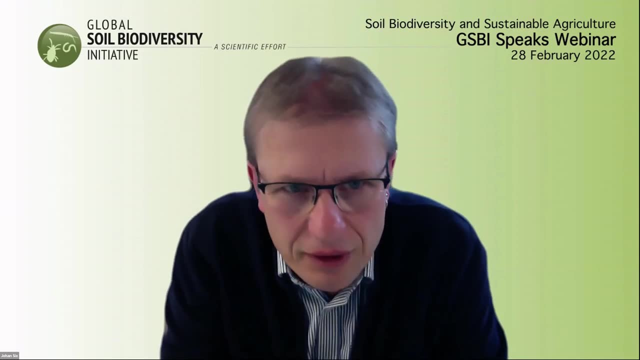 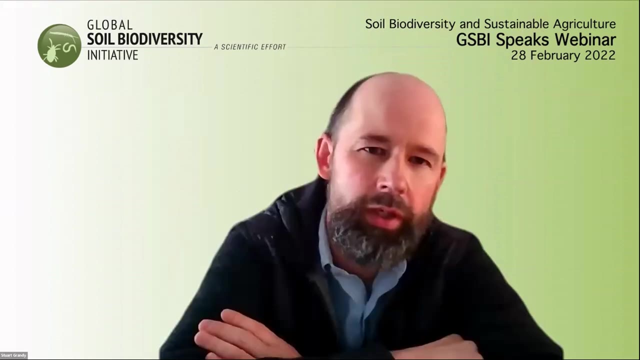 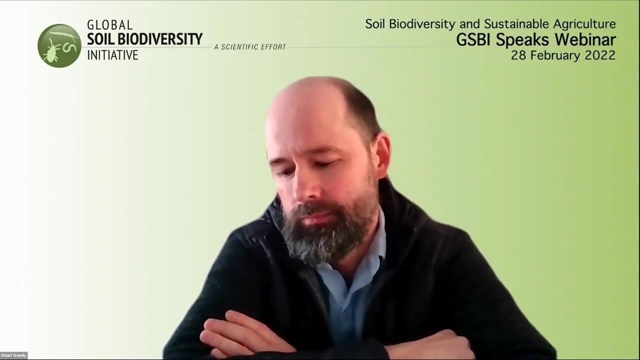 this compost or other amendments, maybe first on for for uh stuart. um, you know the the effect on ma omen. what do you think? well, one way or another, we have to replace the nitrogen that we're exporting from our agro ecosystems. um, we have very, very large and many systems, very large. 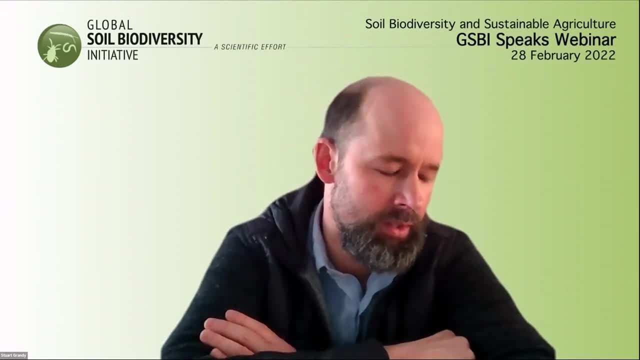 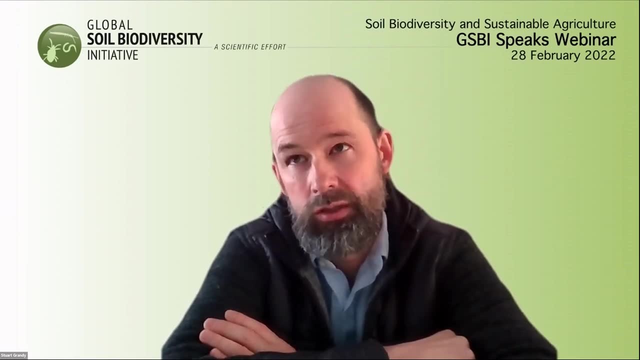 internal supplies, that nitrogen is cycling and and potentially made available to plants and microbes, and we could certainly be doing a much better job intercepting um nitrogen, um having our um nutrients and are putting them in storage and then passing them on to different plants and animals. we could use uh these and and and using these uh in our practices. we would say that 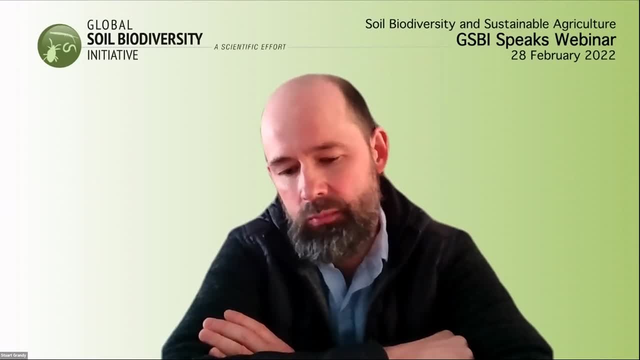 just like what josh said about. you know we could use a lot of nitrogen from our own ears- uh, using our own. i always think that we should keep this, but you know as we are, you know, exploring, a lot of externally applied nitrogen is going through that organic pool. anyway, it's entering. 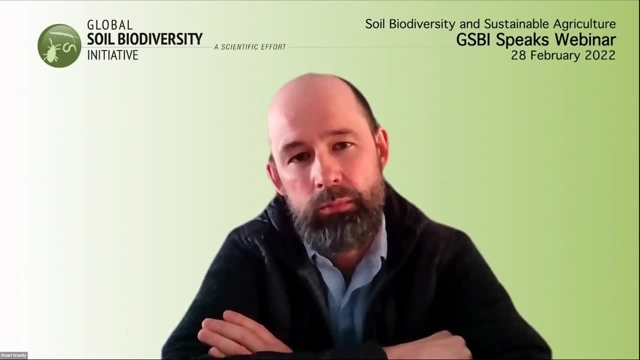 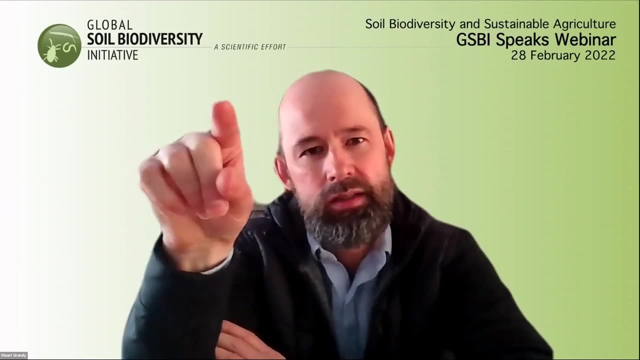 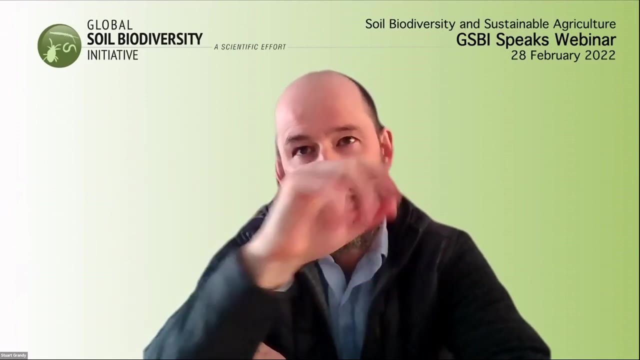 into the mayon pool and subsequently being made available to plants, and that's why the fact that that whole process of external nitrogen being taken up by microbes as they decompose, other organic matter entering the mayon pool, cycling on and off, minerals being remineralized and 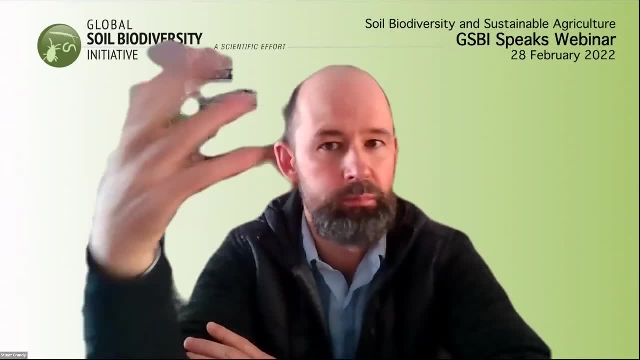 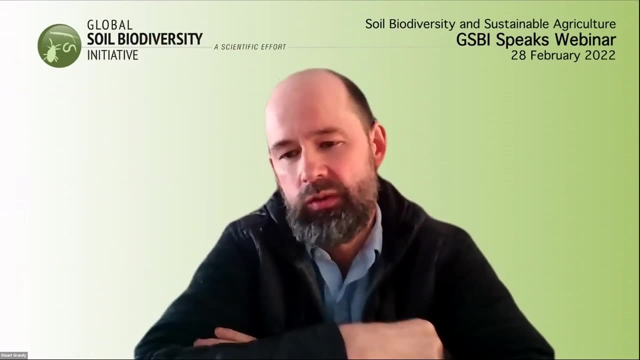 subsequently being intercepted by plants is so important to better understand. you know, right now we just black box it and we've just come up with these general estimates- that you know some very small percentage of soil organic matter and it's going to be available each year. but our laboratory 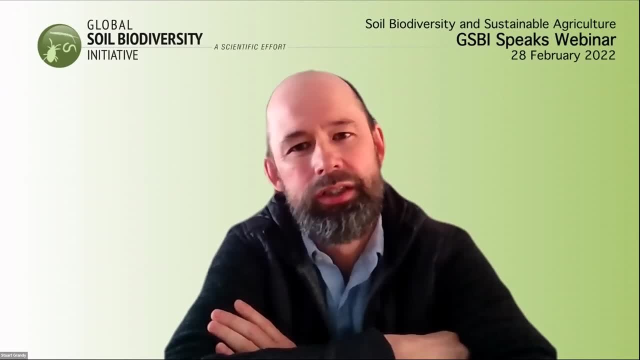 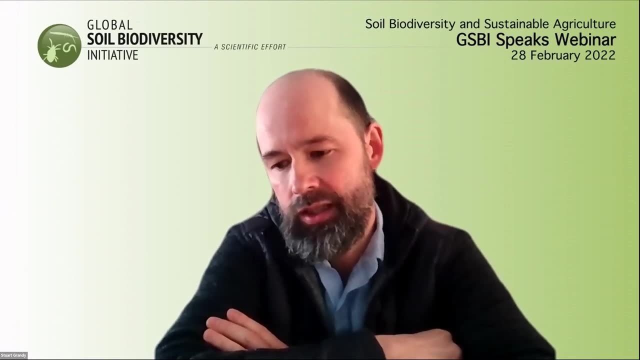 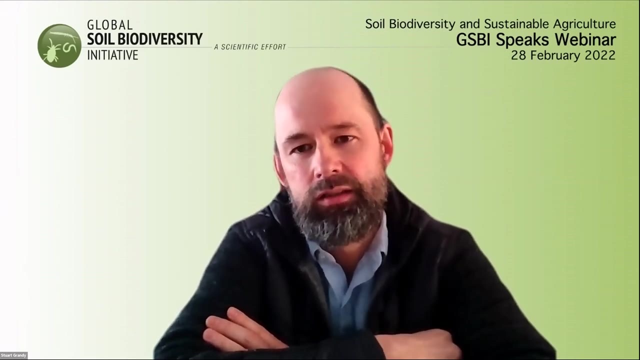 methods and crude assessments are in no way good indicators of what's happening in the rise of and the potential for plants to take that nitrogen up. so, to summarize, i think that external nitrogen fertile fertilizers can augment this process, not suppress it, but we're we have to better understand the 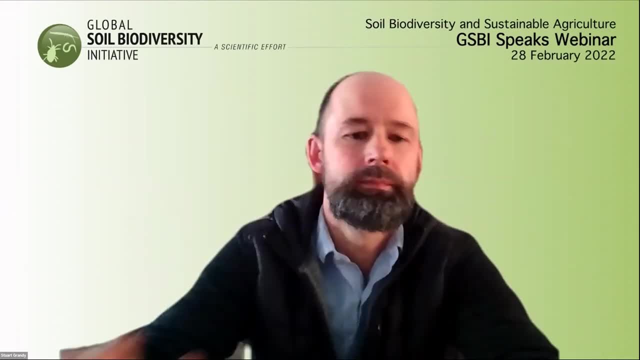 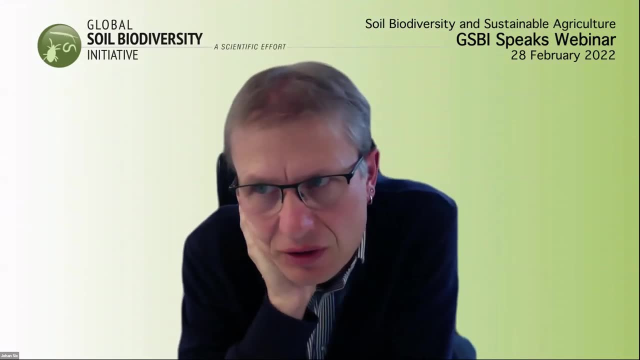 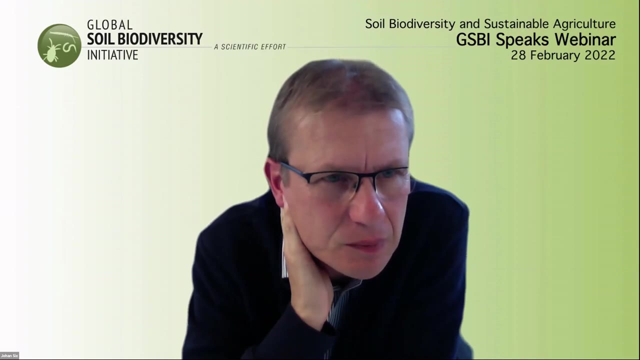 processes to optimize the two working together? yeah, maybe as a short follow-up question that's been asked to joventon is: is the effect of nitrogen on on the amf in agricultural systems? i don't know, to be absolutely honest with you, but i don't think there's a massive effect. 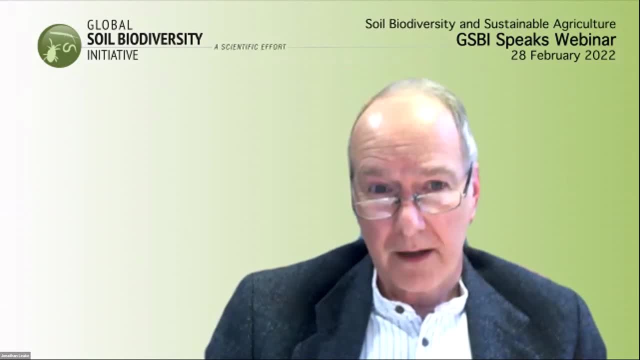 um, and the reason why i say that is that um, for example, with wheat, um, you know we, if you change the management but still use the same nitrogen fertilizer loadings, um, you still get quite high levels of mycorrhization. so i don't think i think the issue with the issue with a lot of these crops, 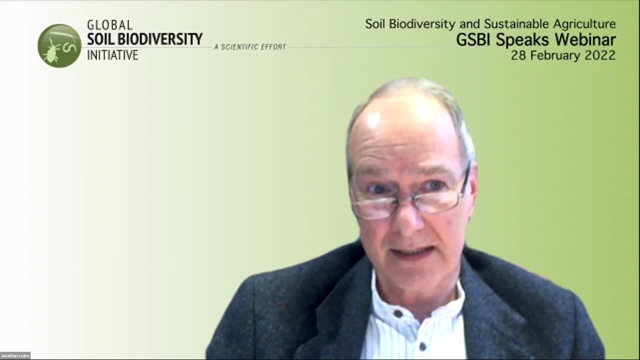 is that the mycorrhizas are phosphorus sensitive, but they're less sensitive to nitrogen because the um the arbuscular mycorrhiza is, is a is adapted primarily, but not exclusively, but primarily, as a enhanced efficiency mechanism for the capture of phosphorus um and and their role. 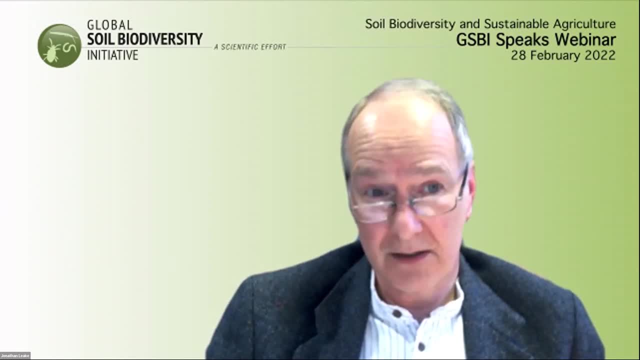 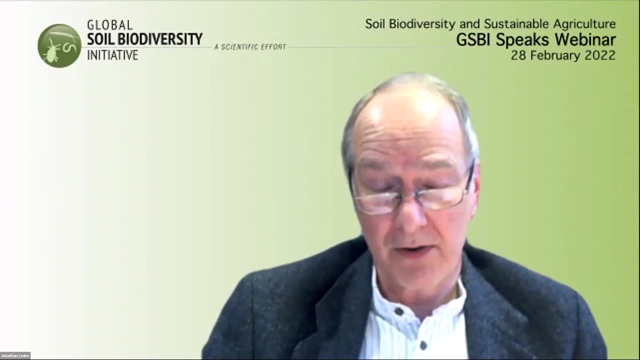 in the uptake of nitrogen is is much more, uh, uncertain, to be honest with you. i mean, they may operate in organic systems and systems of low input, where the where mycorrhizas may be involved in recycling organic nitrogen, um, but in high input systems they probably, probably, don't have the 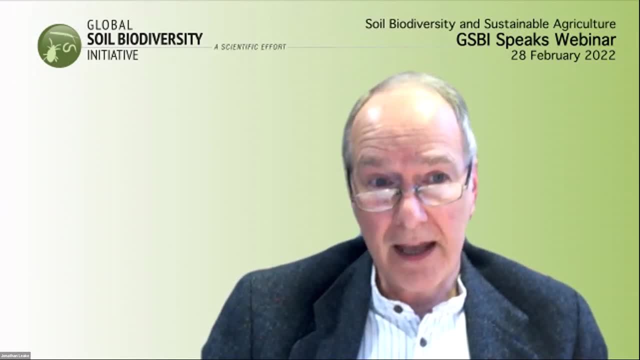 ability to play a minimal role. uh, i think the other issue that's quite interesting is the extent to which some of the chemicals applied in agriculture impact mycorrhiza inadvertently, and there's been quite a lot of studies on things like glyphosate, where glyphosate additions do seem. 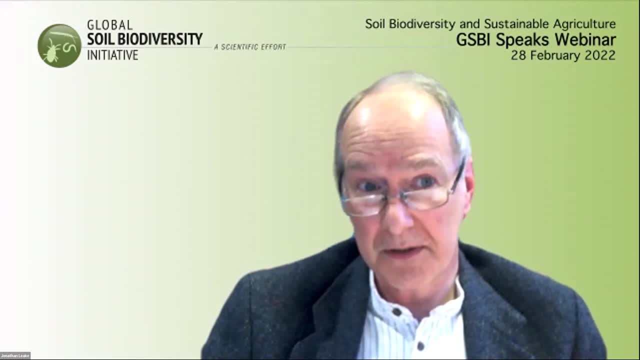 to have negative effects on mycorrhizas under some circumstances. um, but it's interesting, in our experiments with lays we've sprayed off the lays and direct drilled and we've still got better results in terms of how much glyphosate has been plowed or in um shallow disc cultivated uh land. 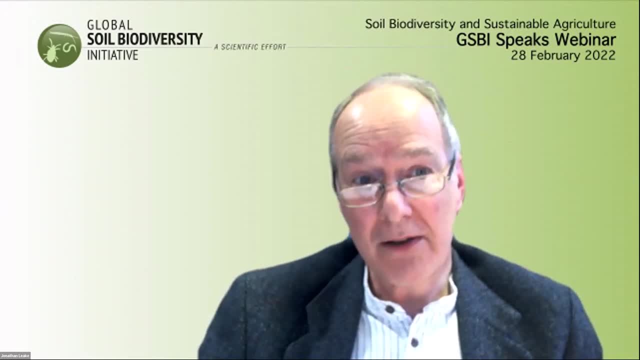 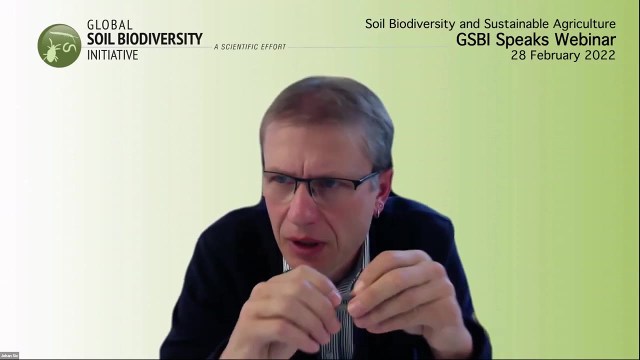 uh. so so it does. just, we don't have a control with no glyphosate, but we still have very good mycorrhization after use of glyphosate uh with a direct drilling approach into laying actually still related to this nitrogen uh. stewart, there's a question about um. you know when you want. 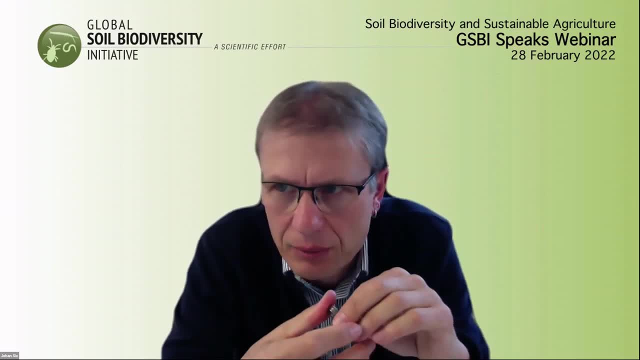 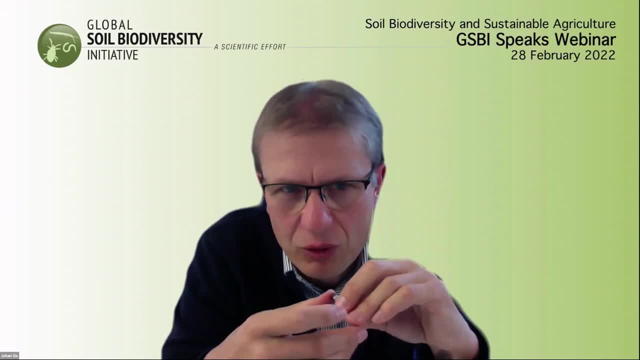 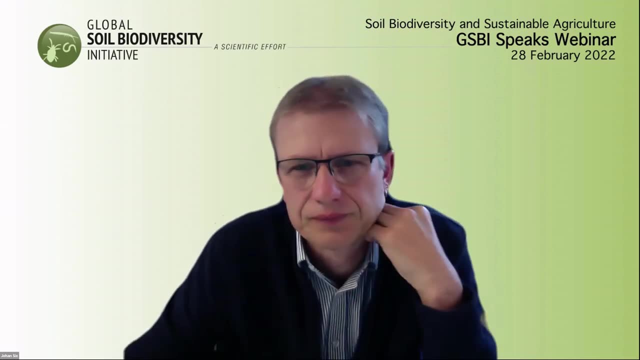 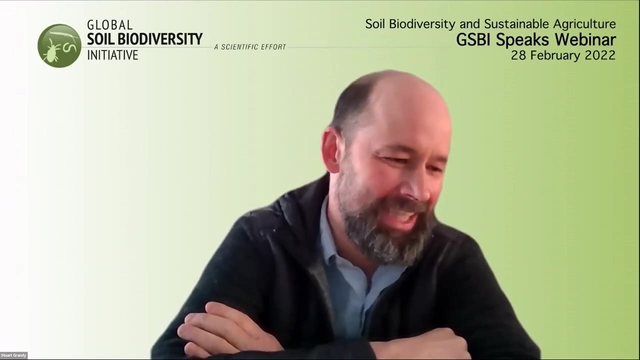 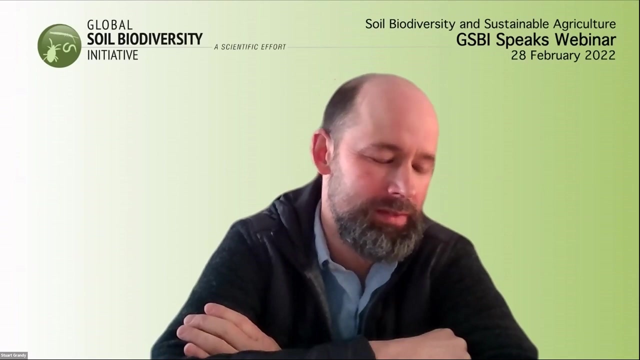 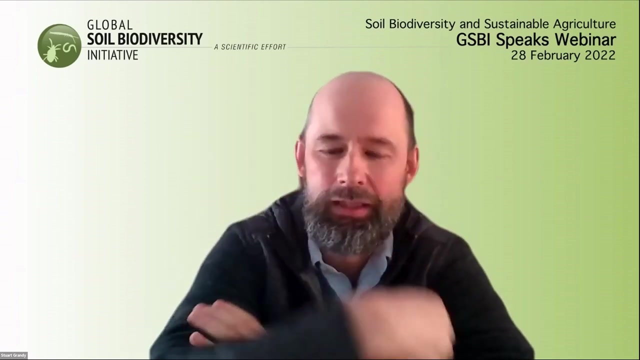 fractionation method, that that is made, that is best, or, or, yeah, any any recommendations on that? well, of course, this is something soil scientists love to argue about. uh, you can't get enough of at times. um, i think that, uh, the simplest approach is just to use a simple soap like hexameta phosphate, shake the soil, pour it through 53 micron sieve and 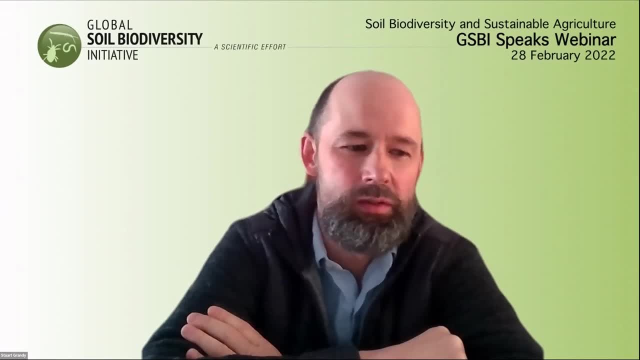 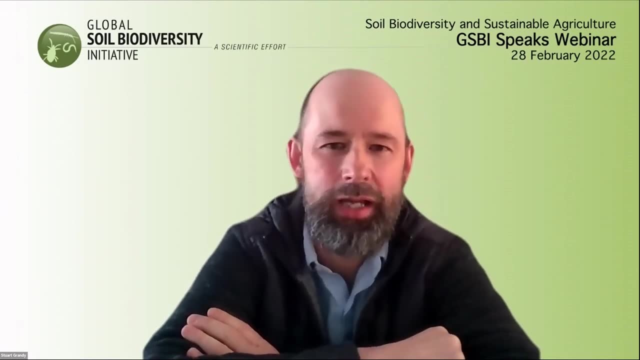 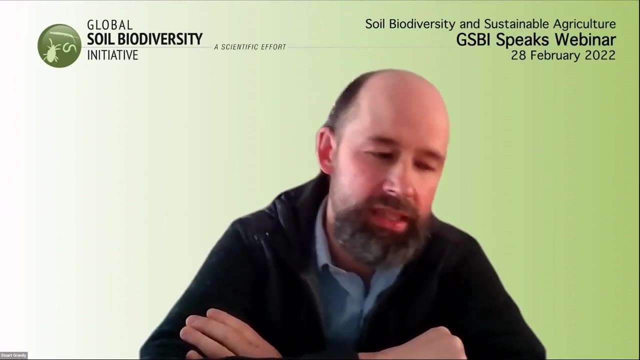 that separates your less than 53 microns so silt and clay fraction from, uh, the sand fraction, um, which would include the palm, so that particular organic matter, by definition, is ending up in the greater than 53 micron fraction. now when we get into more detailed mechanistic studies, 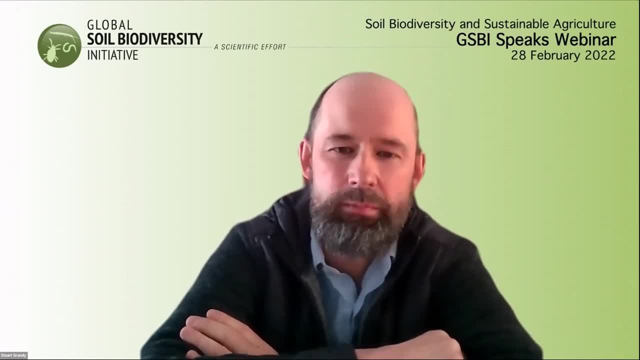 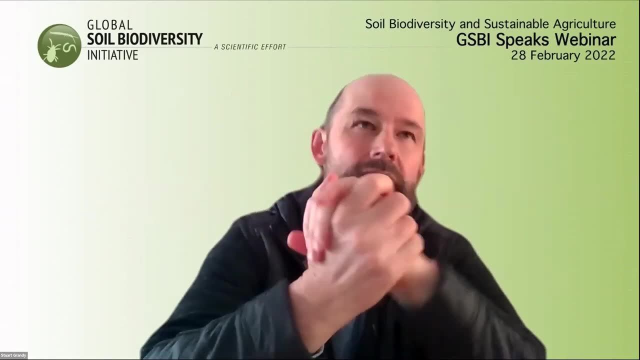 in my lab we're very interested in separating out that less than 20 micron fraction and the reason for that is that the 20 to 53 micron fraction captures the core silts and we think a lot of those are primary particles and they are not associating. 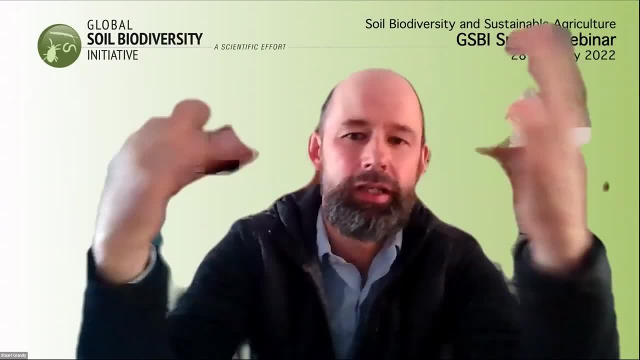 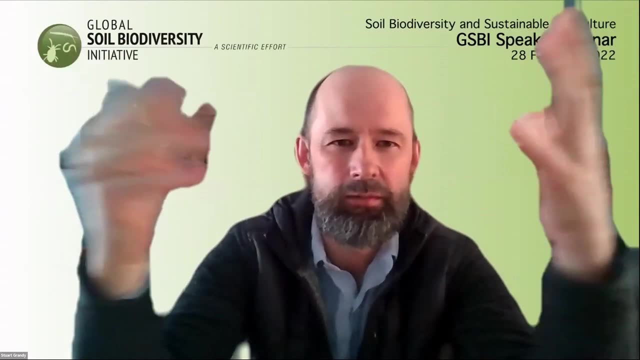 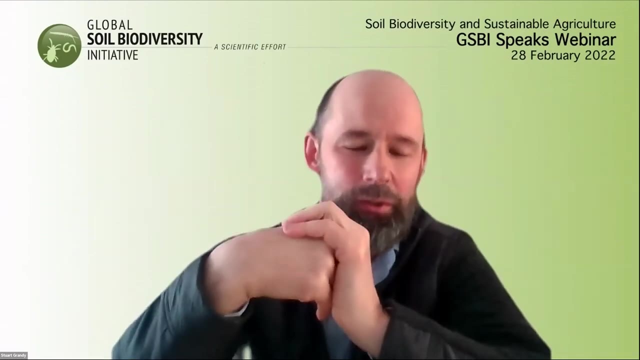 with organic matter in the same way. they're acting more like a primary particle, just a small sand. they don't have the surface area to volume ratio in the reactivity. so we get very interested in that smaller mayon fraction as sort of a hotbed for nitrogen accumulation. but again that takes. 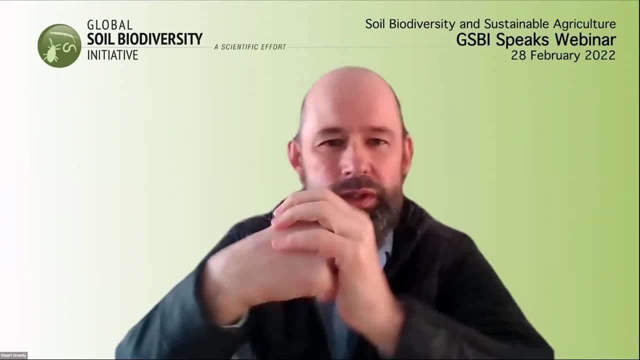 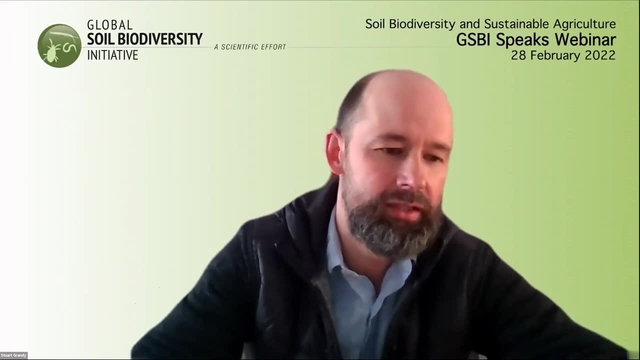 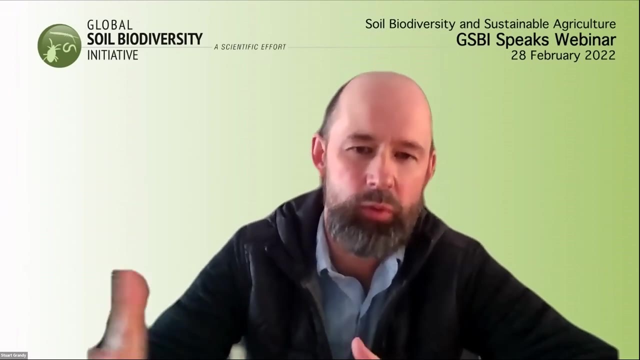 quite a bit more work, and so it depends on the study and what sort of resources you have have available. but if you remember back to that study from kbs that bowls et al did, it was in that less than 20 micron fraction where we saw most of the accumulation of organic matter associated with crop rotations. 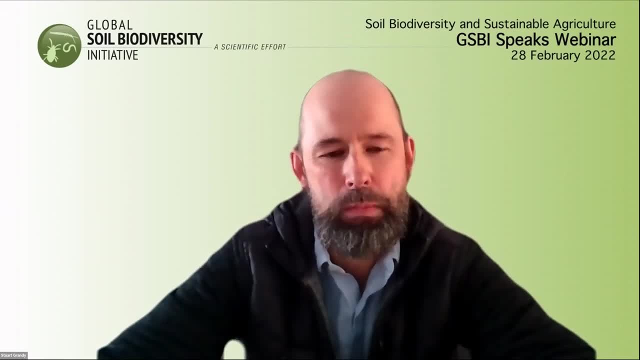 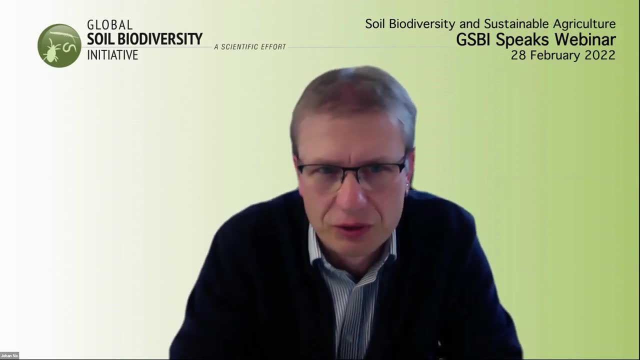 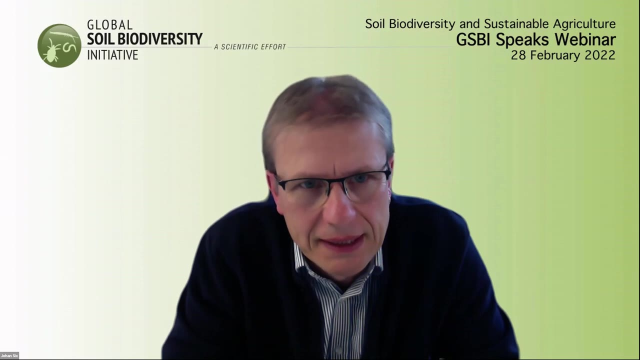 and and nitrogen in particular. so there's also a question that that's maybe a bit critical for you, steward, as on the um, so you're clearly focusing on the malm and and and how that plays a role in in providing nitrogen to um, to the plant, but but what about the palm fraction? is it really just not playing? 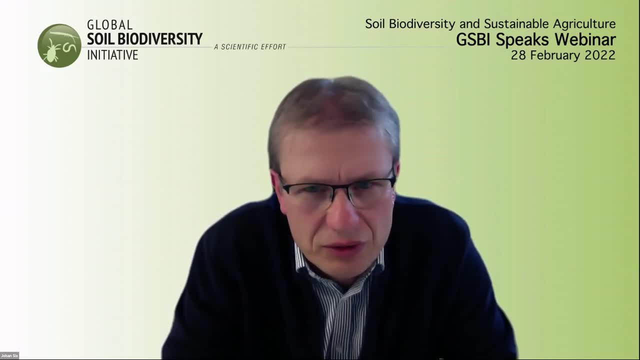 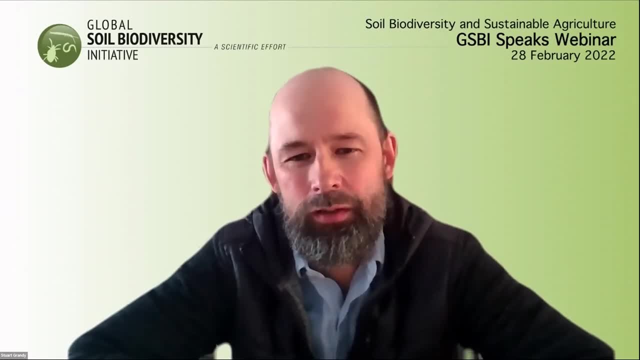 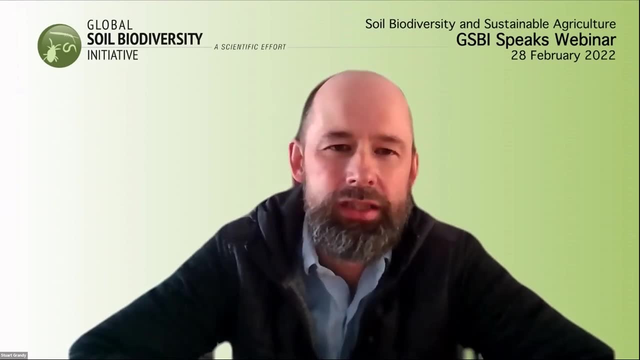 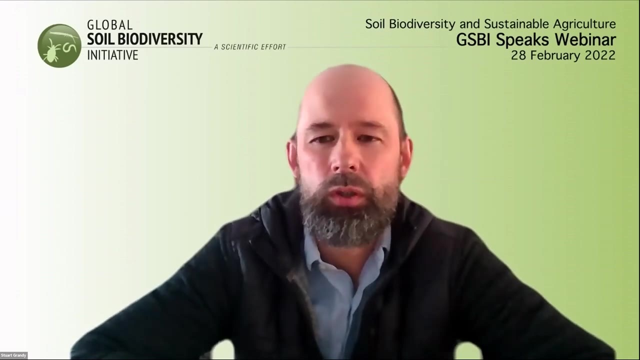 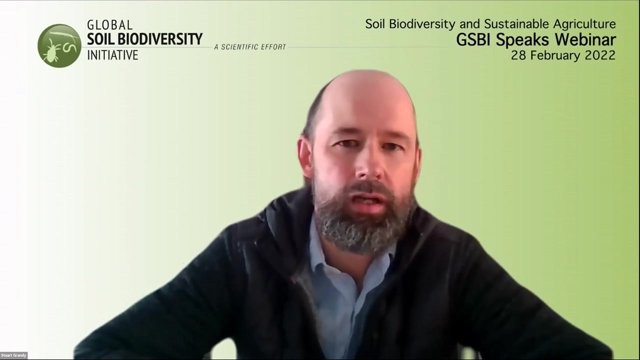 getting overly focused on any one fraction. there they they work together, they interact. the breakdown of one supports the other. um that palm fraction is a really rich source of carbon. um, it has a much higher carbon to nitrogen ratio. it decomposes relatively quickly in agricultural systems a lot of microbes we tend to think of as carbon starved. these are carbon limited systems in. 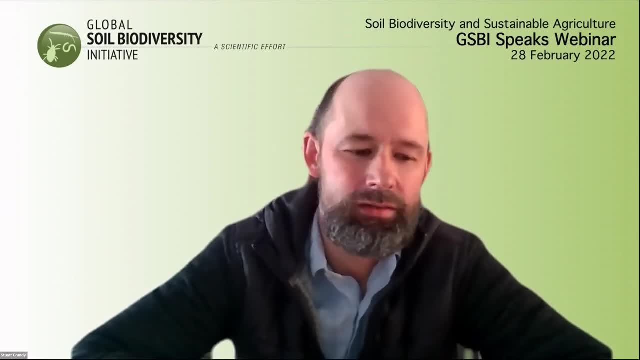 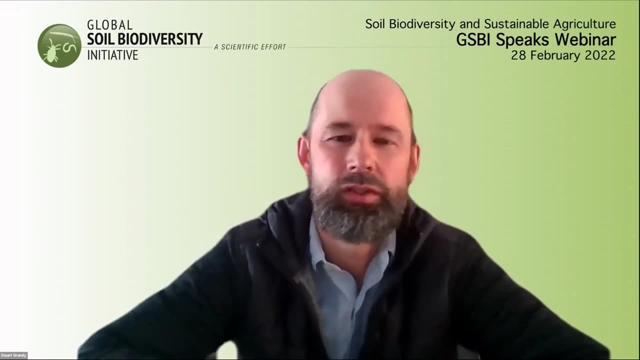 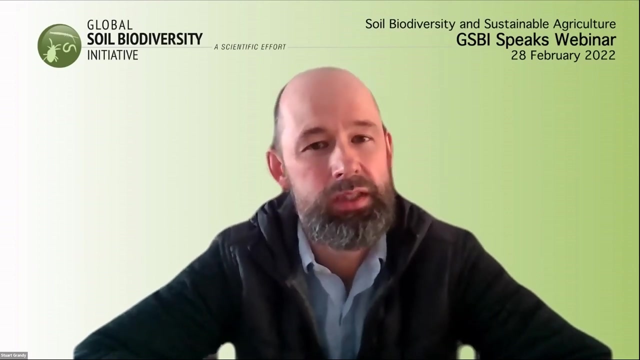 that palm. it's a really important source of carbon. it serves as a seed for aggregation. it serves as a seed for the formation of microbial biofilms. it's the decomposition of palm that forms mayom. in turn, the mayom nitrogen may help support the decomposition of carbon or nitrogen limited palm. 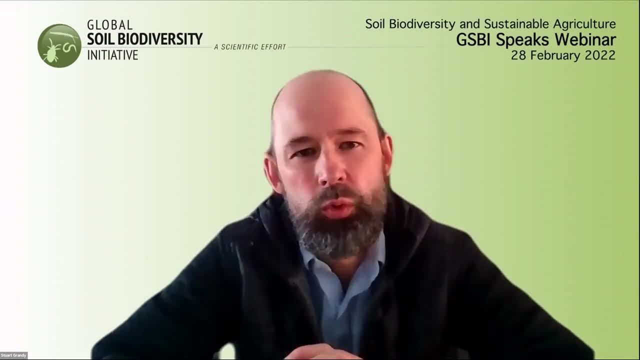 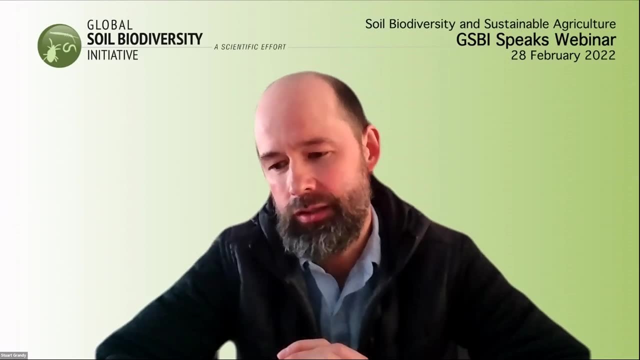 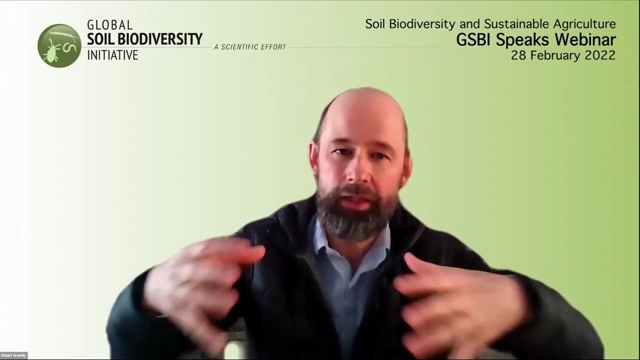 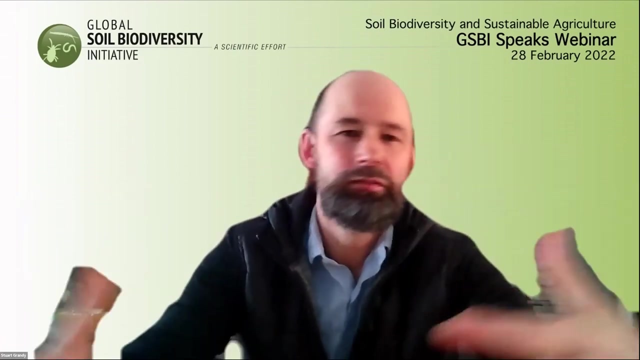 so there's important interactions between these, these different pools, and they are both serving really important functions in the soil. you could coming back to aggregation. you can think of the mayom, carbon and nitrogen and that pool of nitrogen helping to support the formation of little aggregates, and then it's the palm that helps to and the formation of microbial goose and things around it. 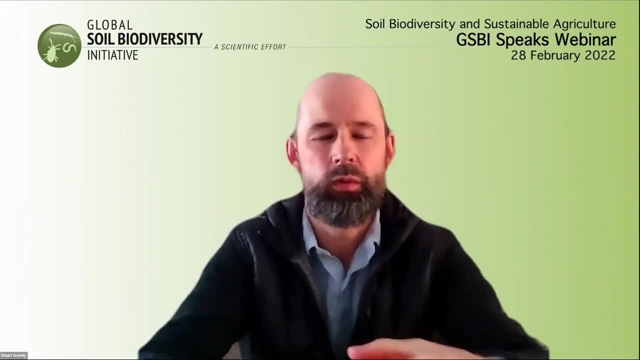 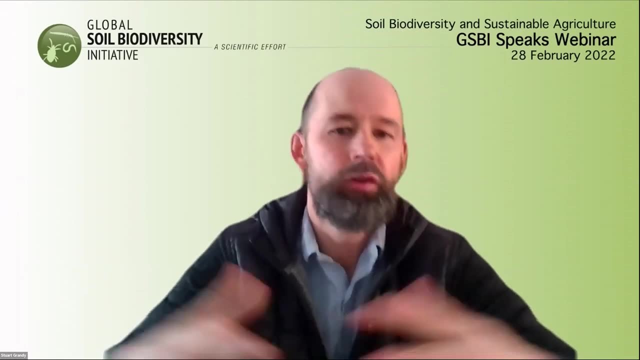 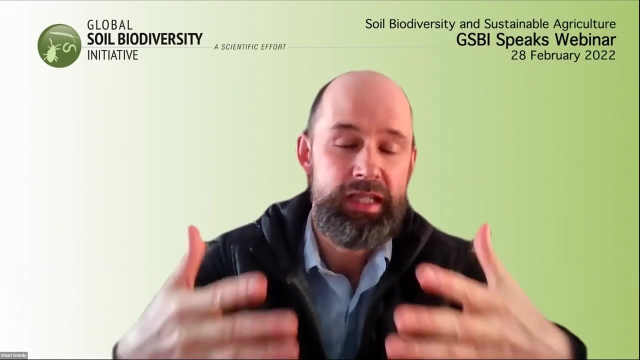 that helps to bring together those small aggregates forming around mayom to form the types of bigger aggregates that really increase pore spaces. so all the organic matter soils is super important. we are just focused on mayon because it's largely been overlooked. as a nitrogen source, it's been considered somewhat inert and we think that there 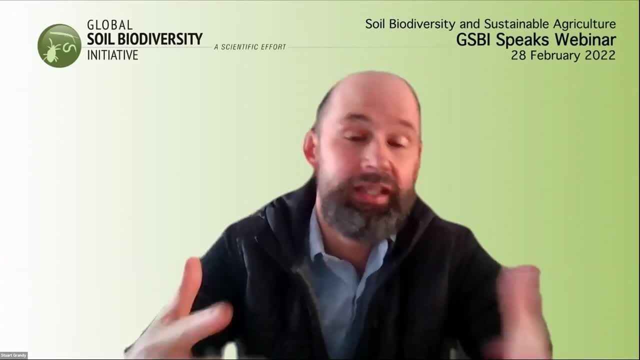 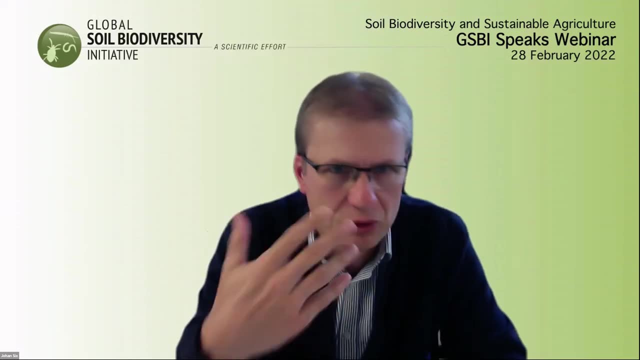 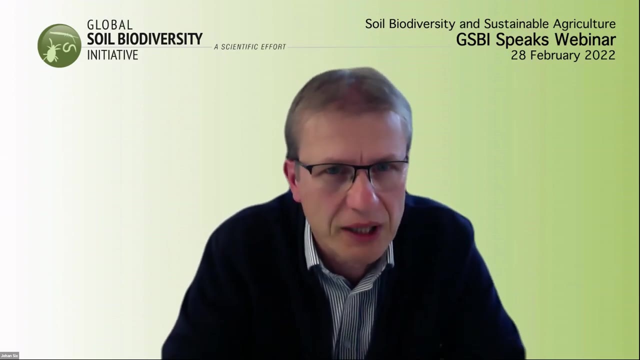 are these plant microbial mechanisms to access this pool? that's like 80 to 90 percent of the total n, so we're actually been talking quite a bit about. you know just how these microbes, and, and then how micronutrients, and, and lead to increases in in plant uptake and such. but there's actually also 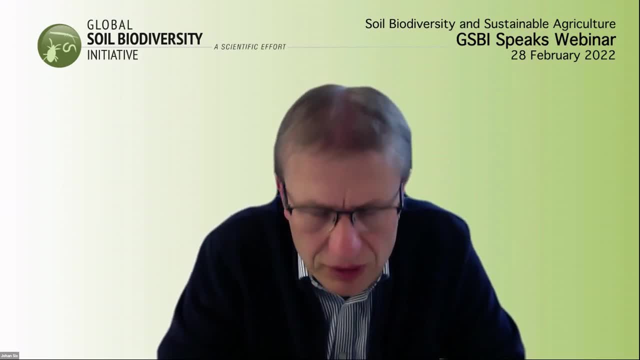 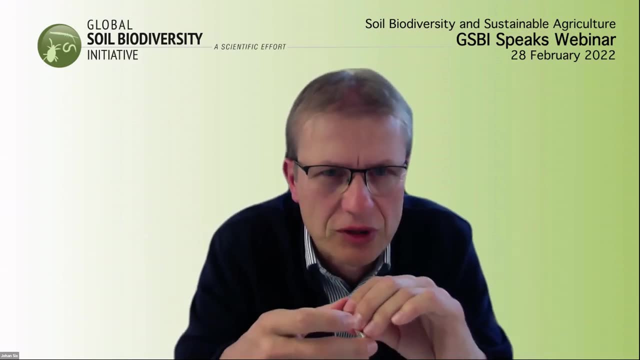 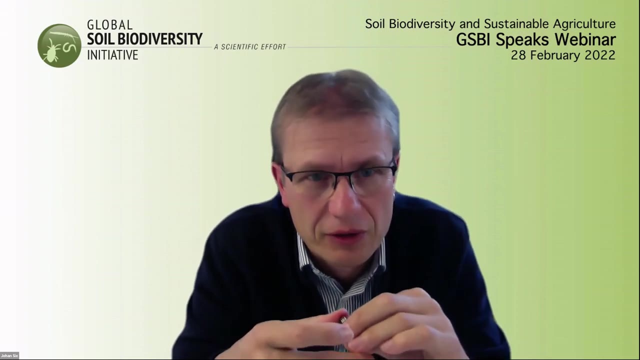 a good question, you know, and- and this was directed actually to herlinden- about if you're talking about, you know, the, the food security, and how microbes can play a role for food security. are you really only talking about the, the yield, so the quantity, or is it also the quantity and the quality and and so is there. are there any indications of of actotherapy that might be there? you know, liquid nitrogen is just in you know soil, but i think it could probably be very good for we have a fewshaped also. you know, nitro NSTA is really a must. he can work the most on nitrogen, like Nit سے. going against nitrogen, like Nit, Columbia старim or nitrogen, still works out very well to me, especially because I think with nitrogen. you know, sometimes you take nitrogen and nitrogen and this good fit means nutrients and distorting petals over time because the nitrogen continuing some property are just likeege exclude. 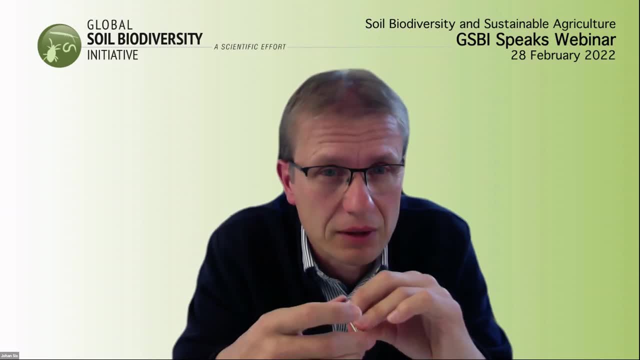 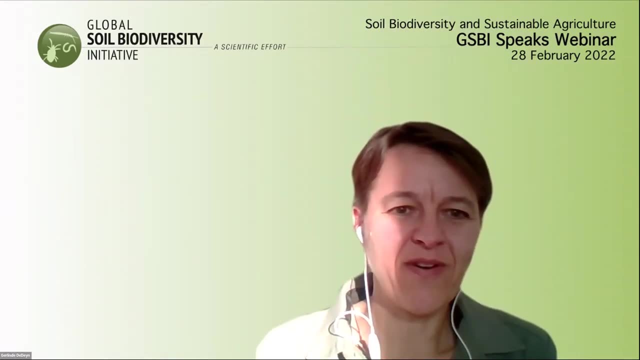 how microbes can actually play a role there. you know, in improving the quality of the product that we're having Very good point: definitely quality. I think we were in the past- maybe some people still have been- focusing a lot on this quantity, but it's definitely not only carbs that we need. we 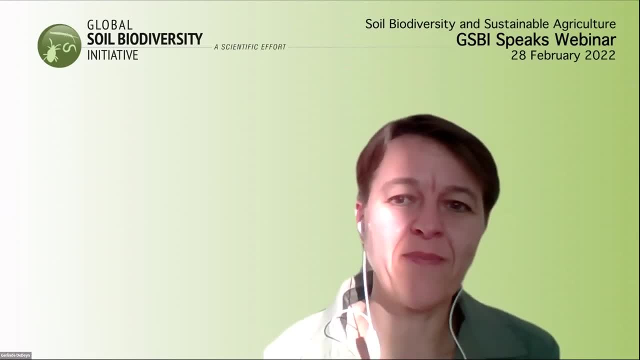 need a very balanced diet, and so also the soil needs a balanced diet, and when we think of these closing loops and recycling, we also need to take care of good balances and avoiding pollutants. when it comes to things like micronutrients, I know, for example, that mycorrhizal fungi- they really can. 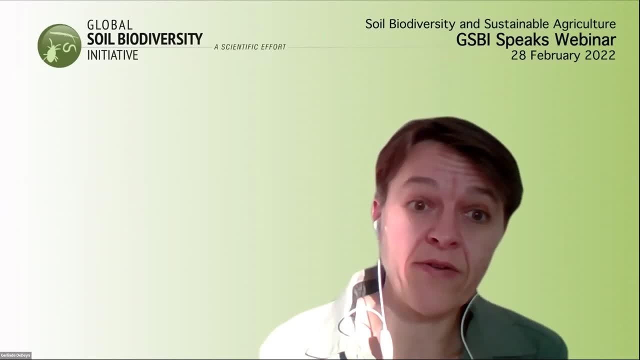 can be very beneficial in that for helping plants to acquire the poorly available but still present. they need to be present. that's, of course, a prerequisite. if they're not present, it's not that any of these organisms are fixing it from the air. that's quite different from nitrogen. 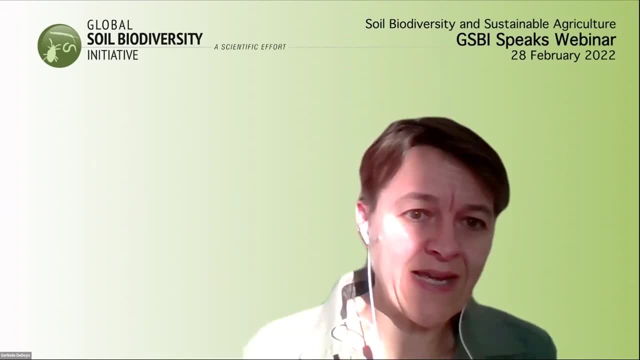 so they need to be present. But promoting accessibility for plants: yes, the microbes have a big role in that to play, in terms of zinc and many other micronutrients. I think there's also a role for really taking a good look at the roots themselves, like in our breeding efforts for new, new crop varieties. I think we 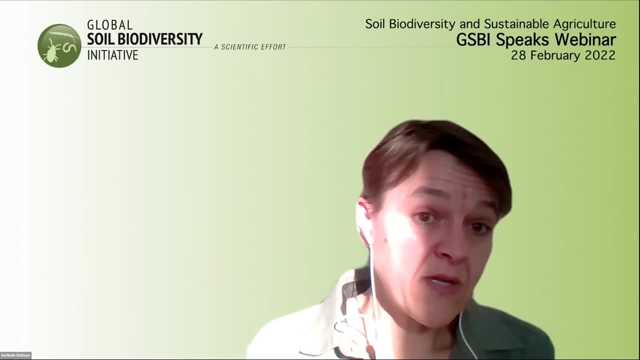 should be more aware of it. and even also crop genotype or crop species combinations that, via their exudates, promote certain uh via microbes, often even the availability of certain micronutrients, and then a very yeah, actually we also work on on one of these examples, but maybe it's a bit of an exotic one. 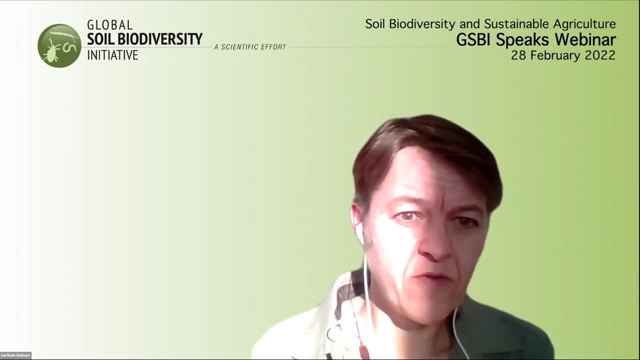 where we also work with traditionally fermented foods, so basically actually augmenting the quality of the of the food product. in this case it's it's a fermented grain-based beverage, non-alcoholic and inoculant, that really provides a microorganisms and also some enzymes or roots harvested from. 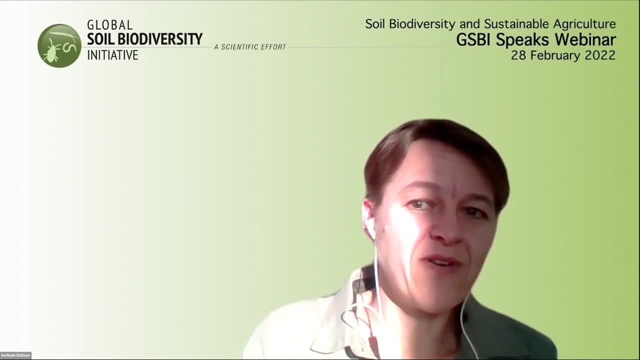 endemic plants. so that's, that's one of the other projects we're running, just to see how is this relation between these microbial communities coming from the soil into the roots, into this beverage, into the, the, even the vitamin um compound? so yeah, so there are links out there. maybe they're not always that obvious and maybe it's especially more traditional type of foods, because here in here we like at least what i experienced in the netherlands: we try to kill things to protect it from not being risky for us to eat, although i like some. 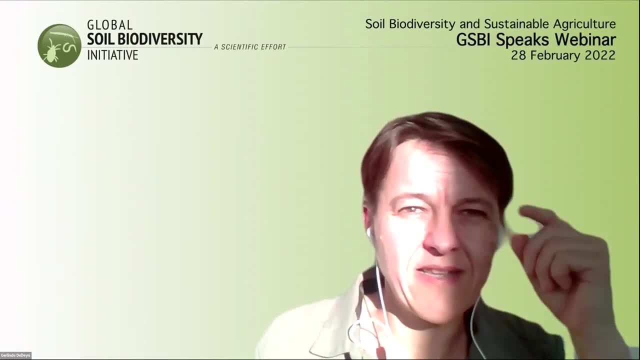 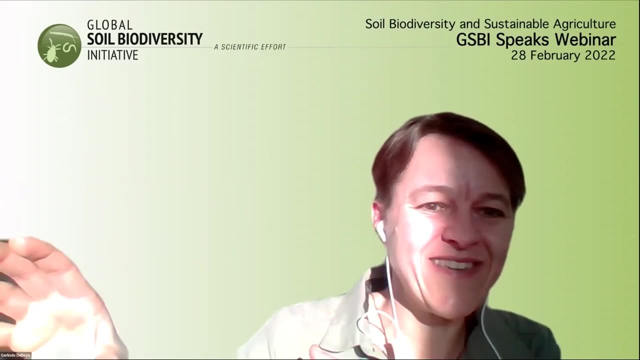 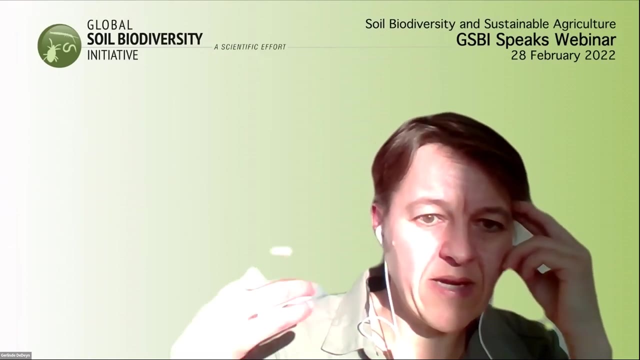 raw based milk type of things, but but they're quite rare. here just to say, yes, there are direct connections and quality is super important and i think that's more on the agenda now than than the the quantity of course we we had. we needed to have that quantity fixed first. i 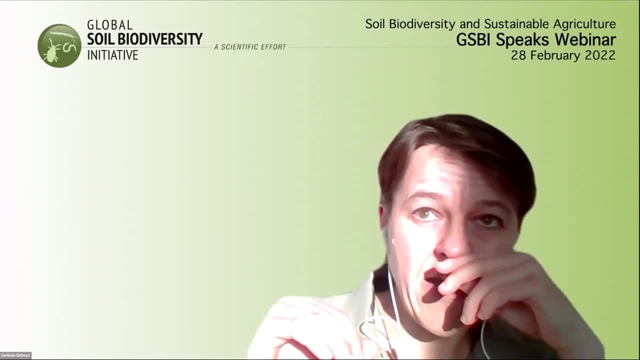 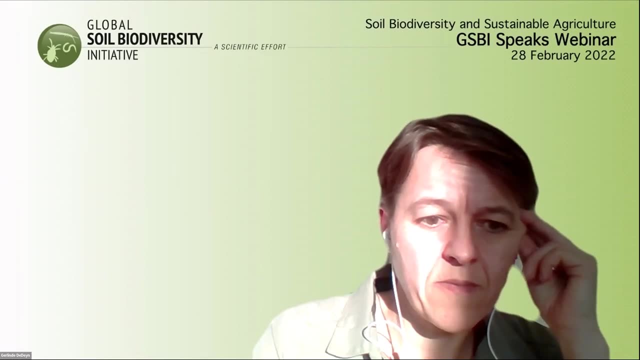 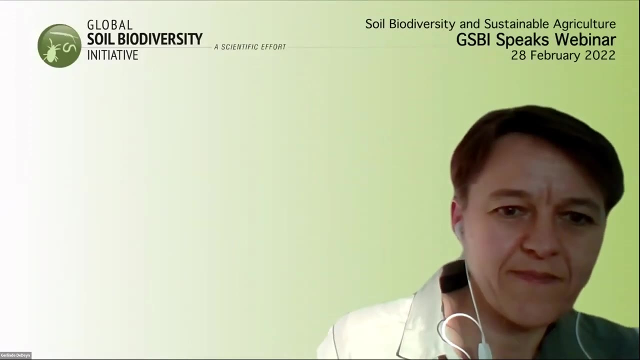 imagine, but also thinking of overuse and and micronutrient deficiencies that really occur. yeah, they're more difficult to study, but they're very important. yeah, there was a bit of maybe. just yeah, yeah, maybe, thanks, maybe just one last question. uh, you know we've been talking about 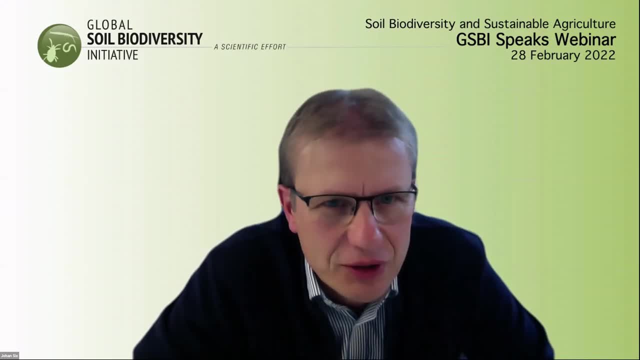 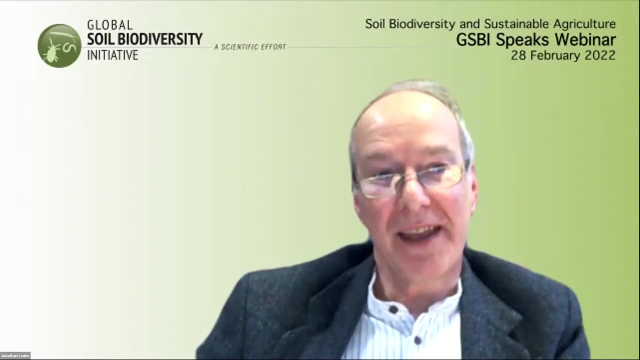 yeah, this compost, the rotations and whatever. but there's actually an interesting question: what's the role of livestock in all of this and can livestock actually help? uh, you know, with building up soil biodiversity. building up soil structure, you know, having a good soil, that that harbors in the the, the soil biodiversity, so livestock. so we're running experiments now. 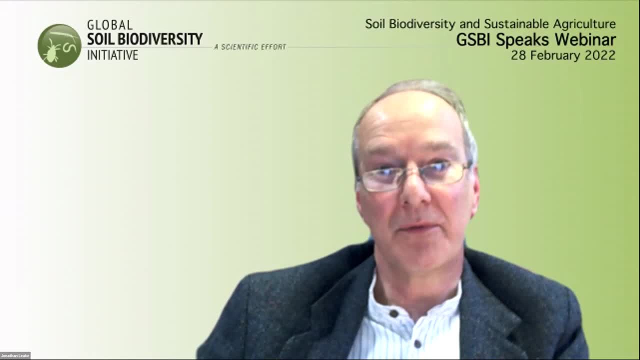 comparing: uh lays managed by mowing versus grazing and there are slight differences but they're not great actually and i would say it isn't essential that you have livestock there. um, and there are disadvantages with livestock. you can get surface soil compaction. you get localized problems with livestock, causing soil erosion. 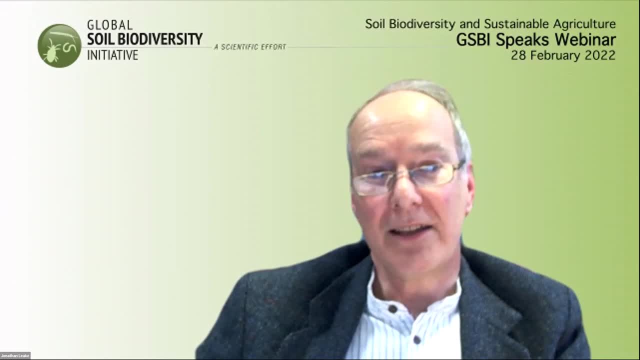 in a way that you don't get if you mow, on the other hand, you get the manure and the urine nitrogen cycling coming back. on the other hand, you could potentially um add those materials back from livestock that's housed, so you don't have to have the livestock on the fields necessarily. 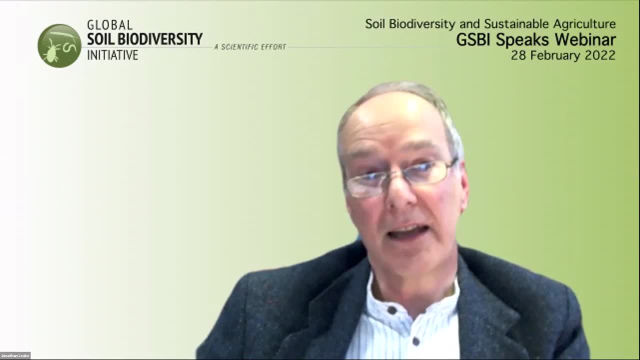 you could produce silage and feed it to the livestock and then, uh, inject slurry back into the ground and provide some of the nutrient recycling in in those roots. so i i think you know the upshot is i don't think you absolutely have to have livestock. i think the systems with 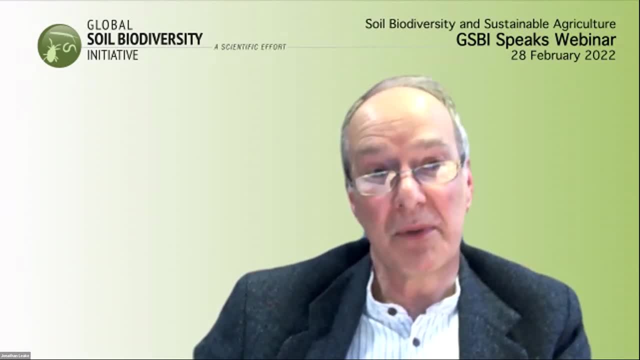 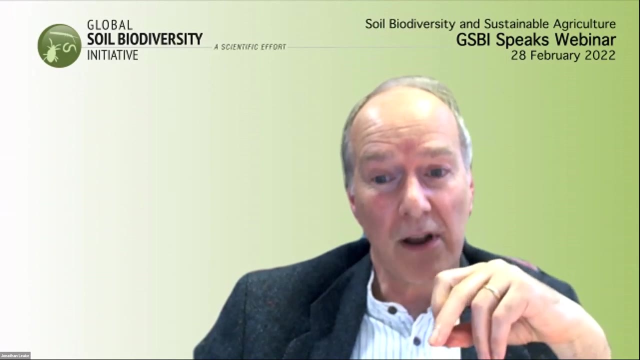 livestock are very efficient and they can be made very efficient by by choosing species that that give very good feed quality, suppress intestinal parasites and also play a role in reducing methane emissions. but, uh, but, as i said, i don't think the livestock are absolutely essential, even in regenerative systems. it's possible to generate regenerative farming systems that are livestock. 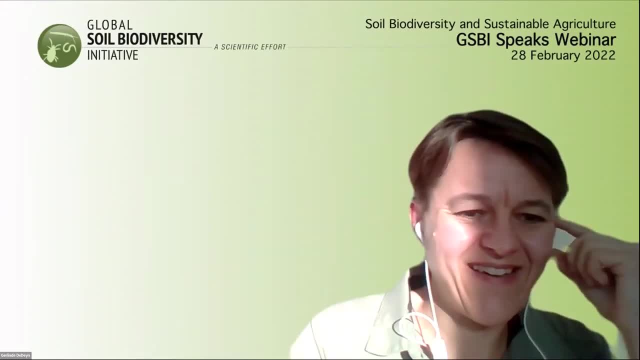 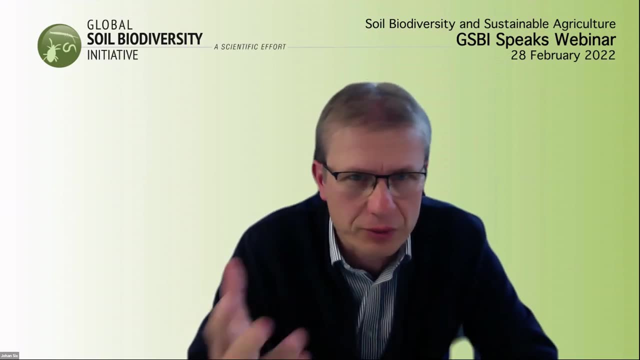 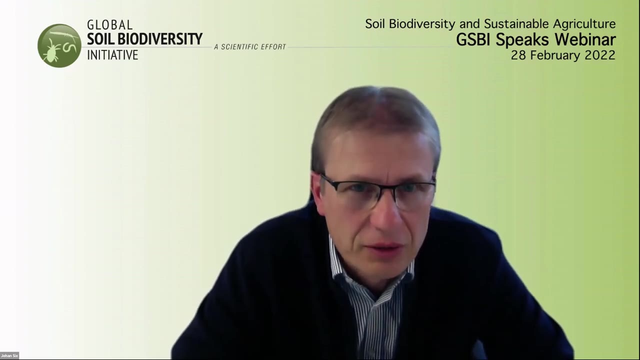 free. i think obviously we do know that in in organic farming i mean, there's a lot of manure being used and organic farming, i mean it's one of the ways that we see that that life is much more in the soil. and you know because of that input and obviously you know if you, if you don't have, 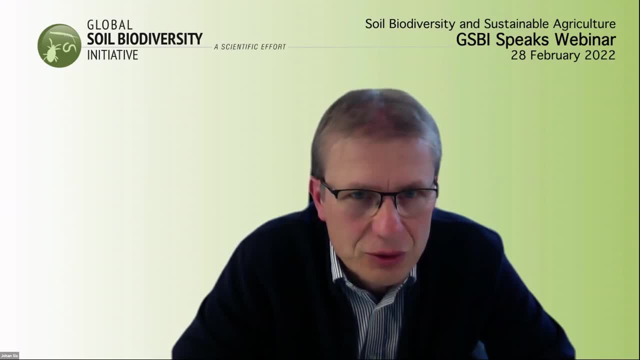 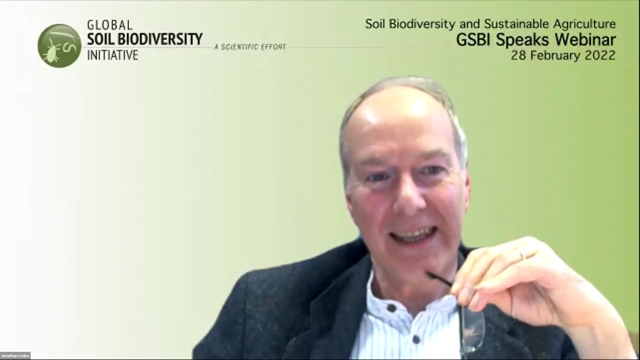 the livestock to to provide that, that, uh, that manure, then then, yeah, what are you going to replace it with? um, you know? i mean, obviously you can do some lays, um, but um, jonathan, you're off, sorry, living root carbon is the key thing. living root carbon, and that's what's missing from a lot. of our systems, actually because our crops have been bred to have relatively small root systems, or indeed we're actually cropping the roots in the case of potatoes or sugar beet. but then, when it comes to lays, i mean, you do mow them right and you also want something. 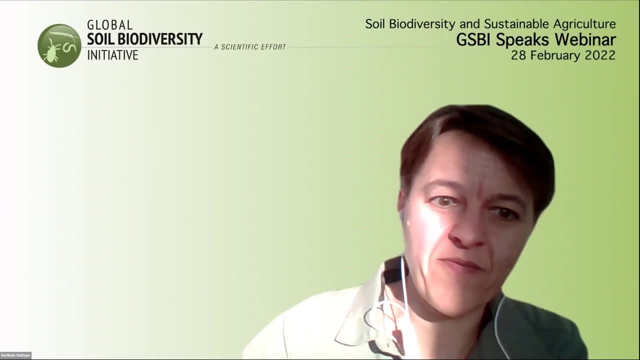 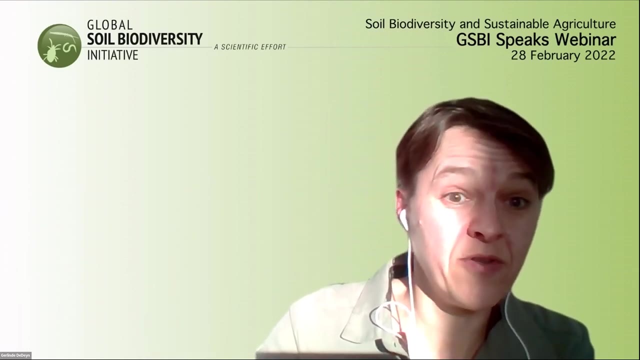 to eat that and then to produce poo with structure, hopefully like formula, when you can be really beneficial in helping to build well soil, organic matter which contains carbon and nitrogen at least. yeah, from from the like the yorkshire dales experiment. i was involved in the former manure. 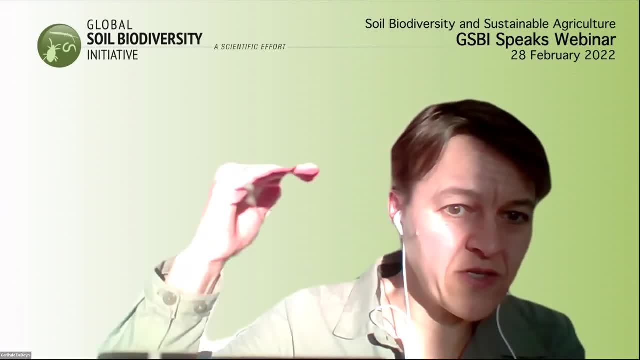 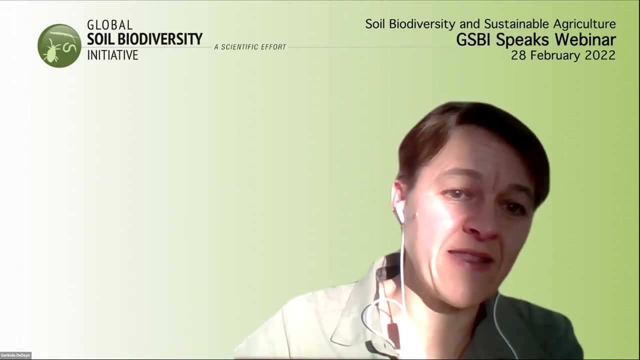 then one had a really big impact, positive. but of course you need a certain i, you shouldn't overdo it either, but um, in such a way that your plant community can be maintained and like in this diagram that i showed, the van zanten diagram on this circular agronomy, actually especially livestock that that feeds on on.